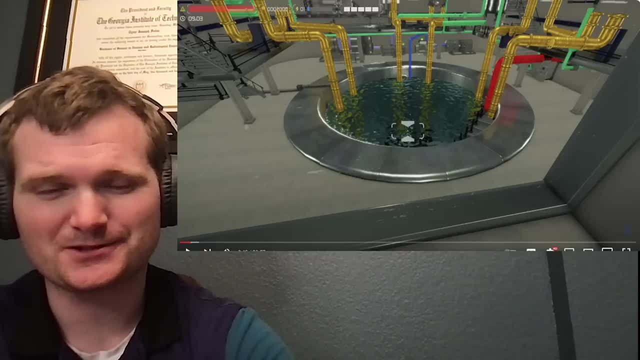 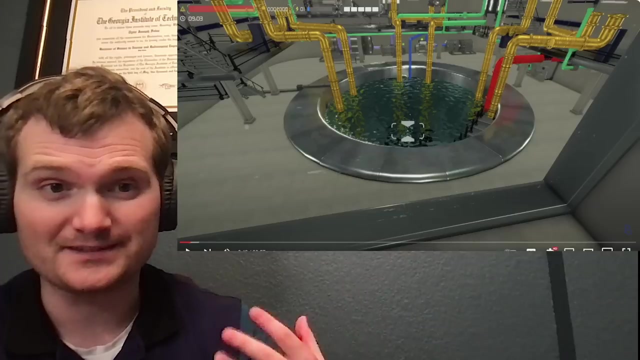 refueling pool and we're clearly shut down right now, because right now it's open. There's no reactor, The reactor vessel, the reactor vessel head has been removed and it looks like got pipes going into it from above. That's weird, You'd never see that. because due to seismic concerns, earthquake- 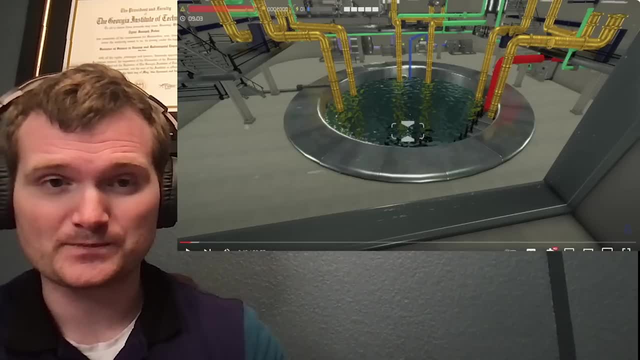 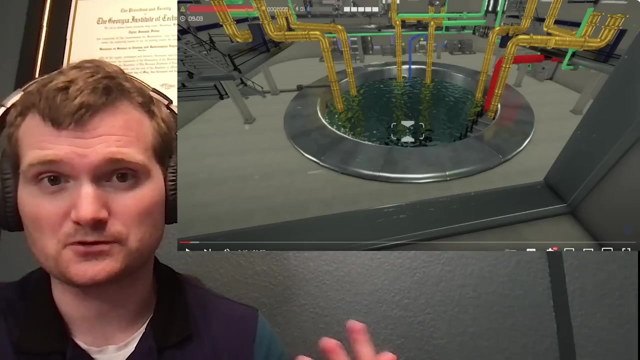 concerns. you would actually see the pipes would be going in underneath, at lower levels from where the pool is located. It would still be above the fuel so you can discharge water over the fuel, things like the residual heat removal system, the emergency core cooling system. You're not going to have pipes suspended. 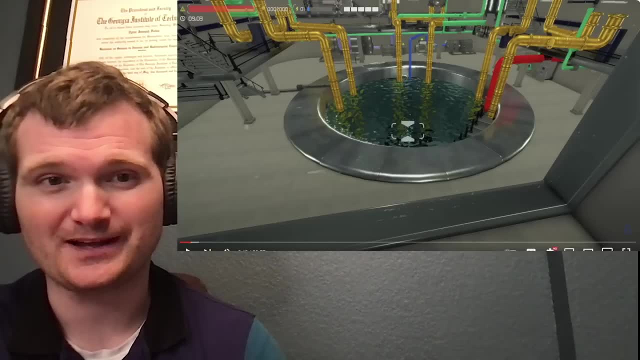 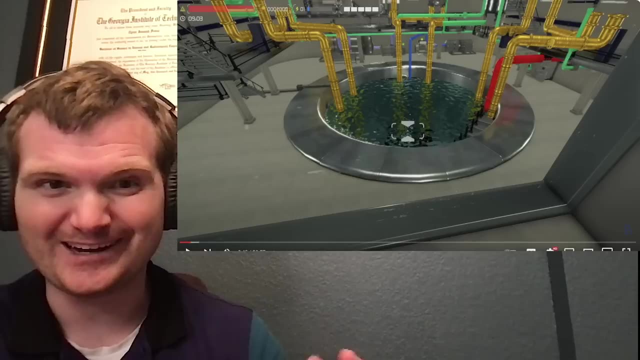 above the core. All kinds of protocol has to happen. This is when you're refueling, before you can put loads over there. Also, refueling would be kind of a nightmare because you'd have to navigate the fuel assemblies around each of these pipes. 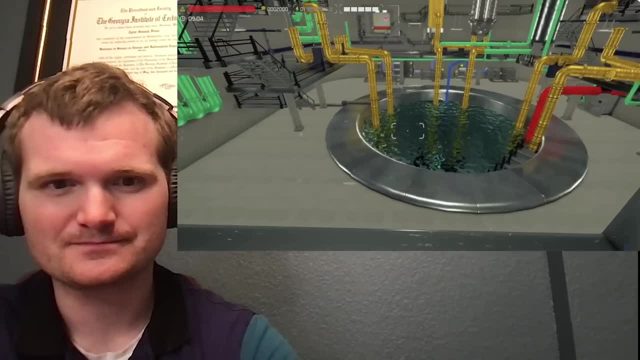 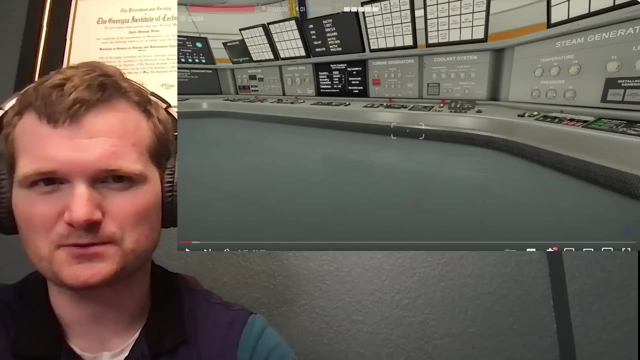 That's another reason why you don't do that: Hovering just a little bit out of the reactor containment room there itself, which is pretty impressive. Also, the control room is not in the same room as the reactor containment building. The control room at the plant I called it would be in the electrical auxiliary building. 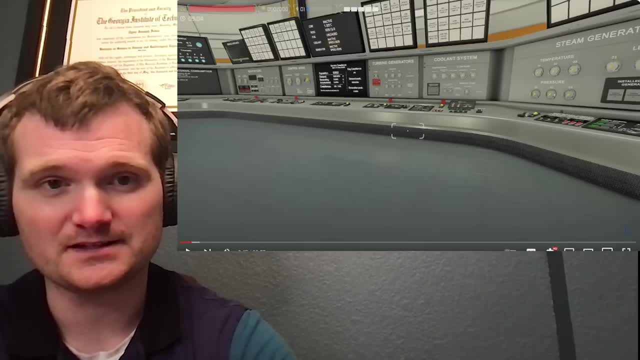 and everything in the reactor containment building is operated remotely Granted. things can be operated manually. You can send an operator in there to manually operate certain valves, ones that are not near the reactor because of high dose rates, things that are within the reactor coolant system, Not to mention high temperatures and high 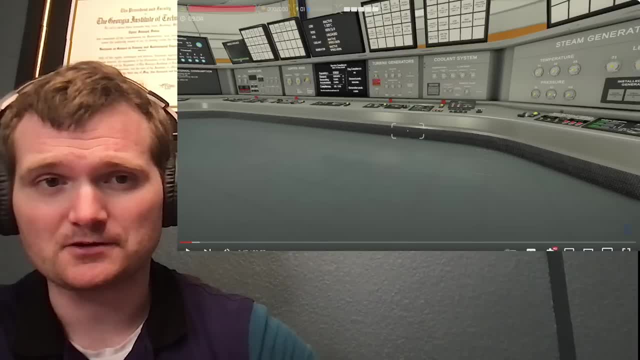 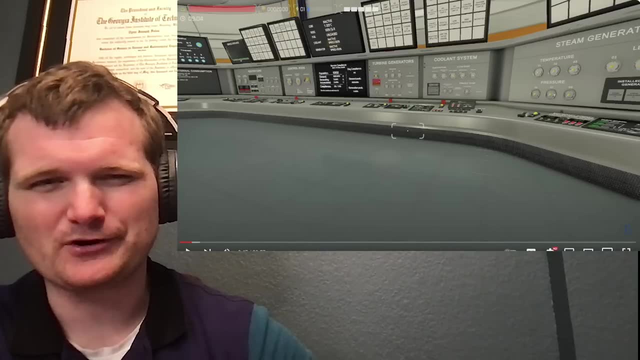 pressures. but there are a lot of other components that can be locally operated in the reactor containment building if need be. But yeah, It's in a completely different area. I've never heard of a control room being inside the reactor containment building. 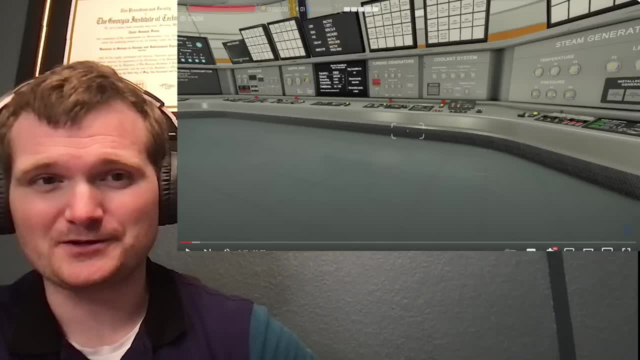 and the reason for that is you just. The containment building is when an accident happens. its design function is to withstand the extreme levels of pressure and temperature and radiation and contain that within there. You do not want people to be contained in there with that hazardous scenario. 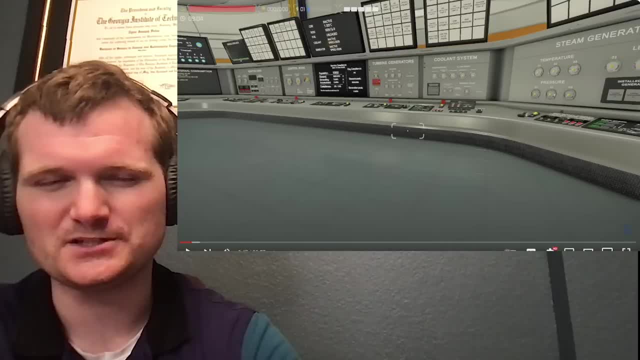 It would not last very long And, yeah, that amount of glass wouldn't do much. in the event of, say, a loss of coolant, accident with pressurized water at over 2,000 PSI and over 600 degrees Fahrenheit, No, That wouldn't do very much. 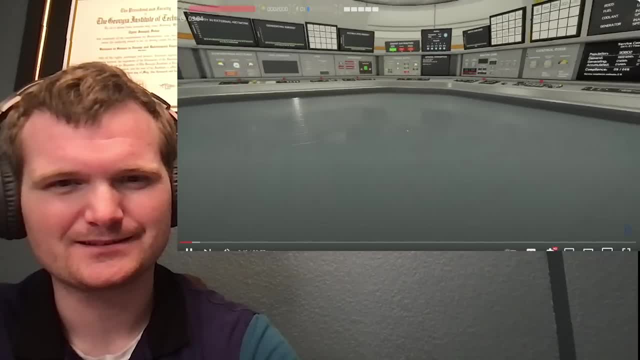 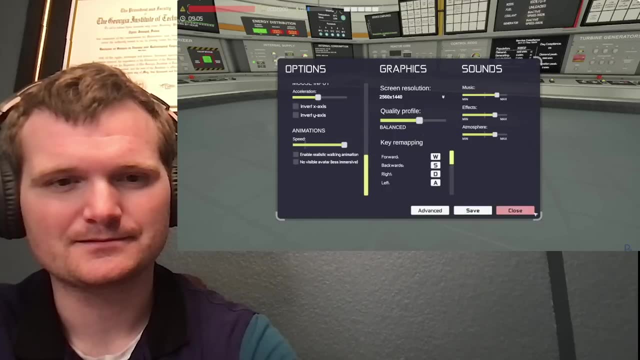 So the first thing you should do when you load this game up- and this is just a quick little tip- press escape, go to options, scroll all the way down and crank up the animation speed And you're probably sitting there going. wait why. 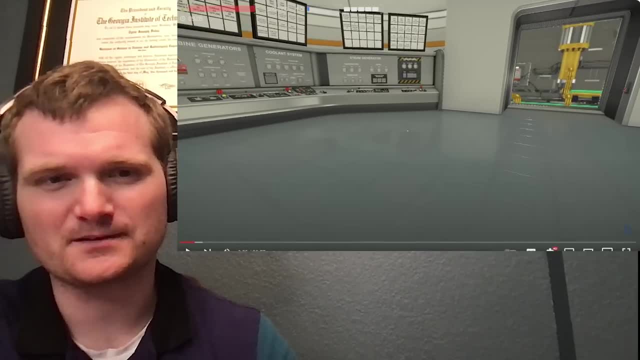 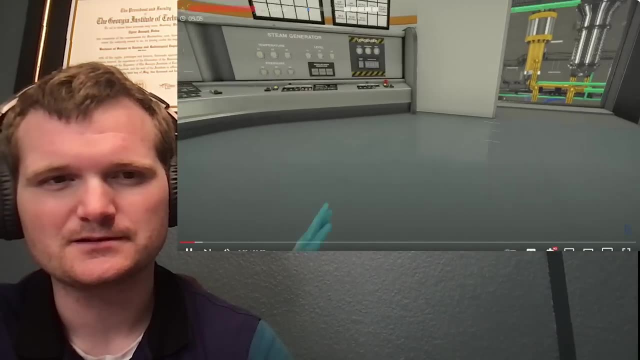 This is So. this video contains commentary. He's going to help you play the game and I will evaluate the realism of this place. Why? Because when you run over here to actually push a button, you'll notice it has to go. 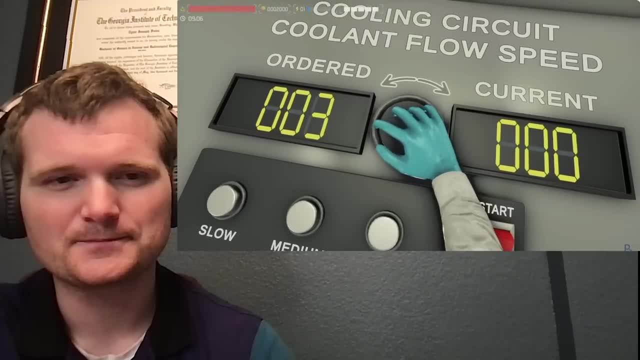 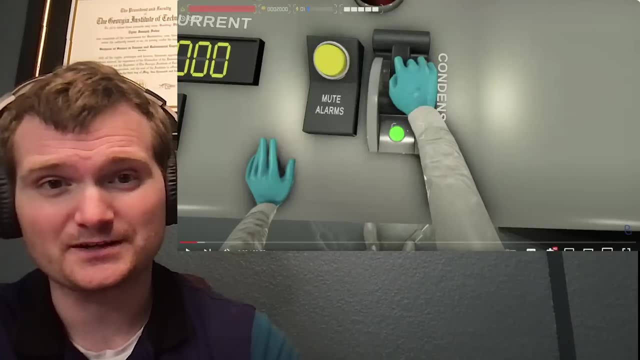 through an animation to push the button. If I'm going to grab onto this knob, you have to actually animate that knob and it takes time for you to finish that up. Now, that's a cool feature showing the action of what it's like to operate. 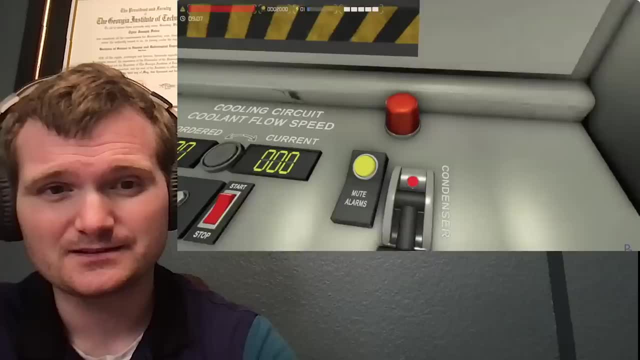 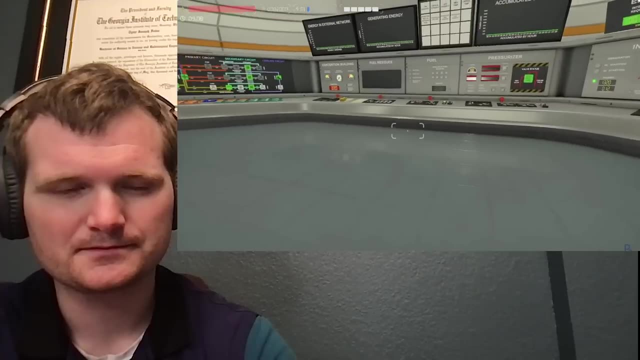 some of these switches. That's a pretty cool feature. And if it's an absolute emergency, of course, and you're cranking on those things, you've already wasted too much time, It's kind of one of those little things. Another really really quick tip of this game, too, is if you hold down the shift key. 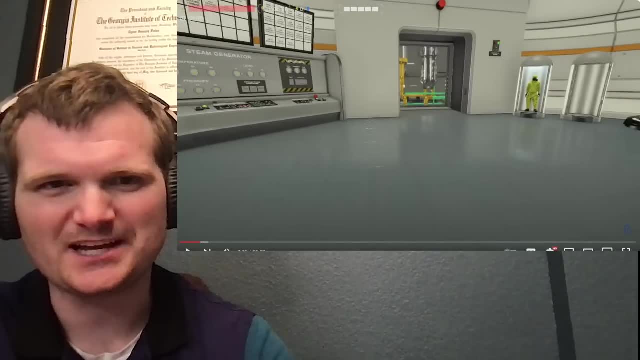 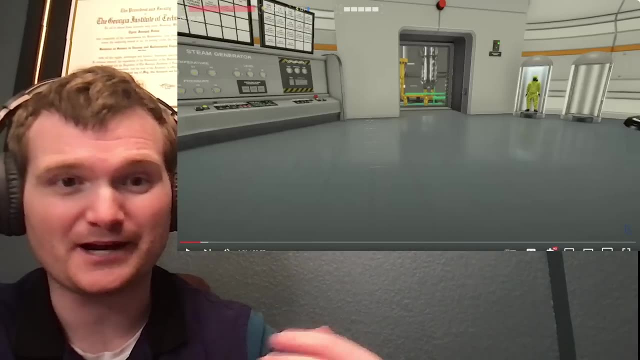 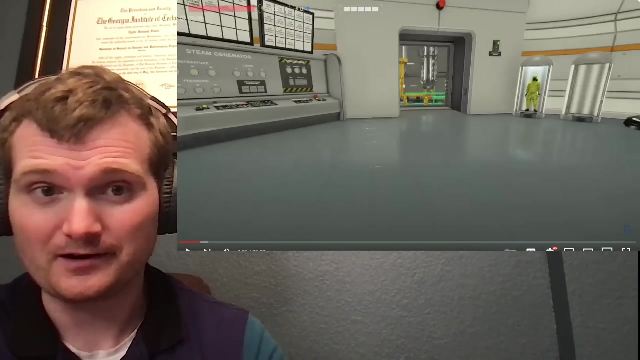 you run a little faster. This control room is huge and it's very, very empty. I mean, it's actually probably around the same size, but there's desks, computers, areas where the control room supervisor and the reactor operators would do a lot of work. just paperwork. 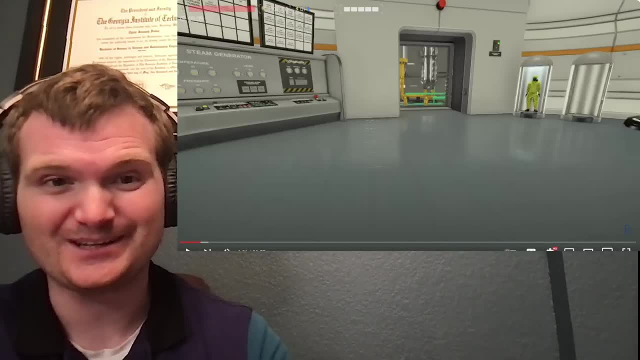 computers, sending emails- Anything you would at any other office job- But here it's just the controls. by itself, It's not the controls and an office, And in some nuclear power plants you could actually have multiple units being controlled from the same room. 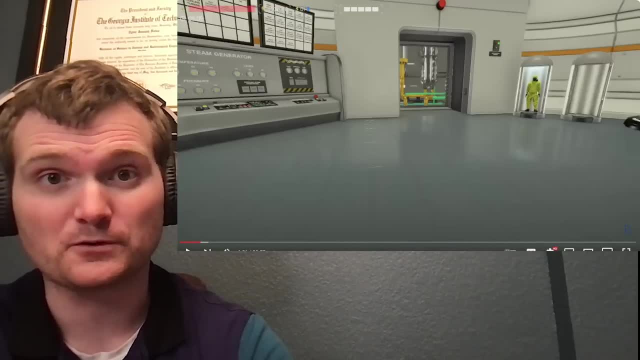 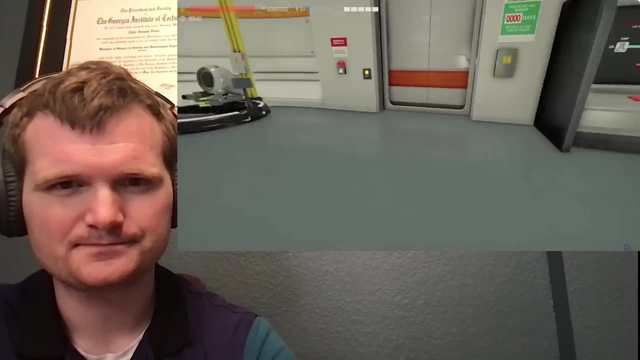 That wasn't the case where I worked, but it's not uncommon for it to be the case. But if you hold down a strafe key and a movement key, you move twice as fast. So if you see me ripping around like a bishop, which is like: why are you doing this? 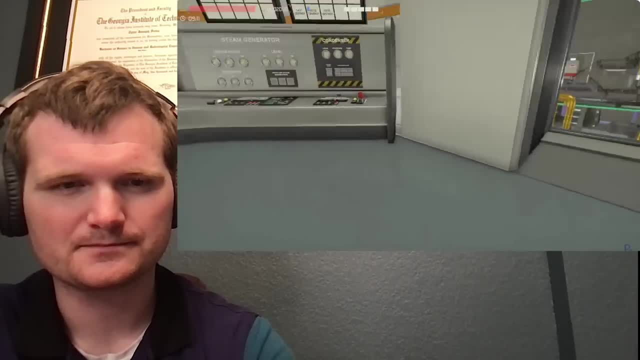 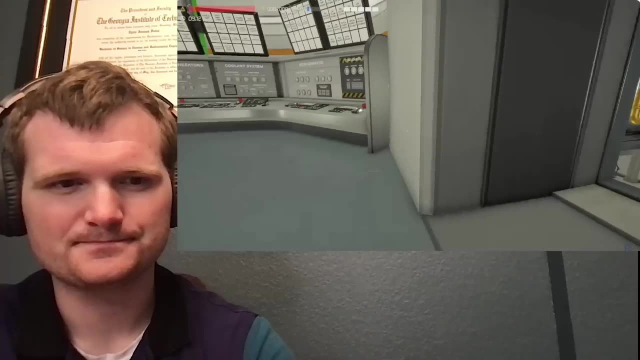 This is a Unity at its best right here, because these two speeds actually add together to make you move even quicker. I know it looks really, really awkward and it's definitely not RP-like, but, believe it or not, it is a fantastic technique. 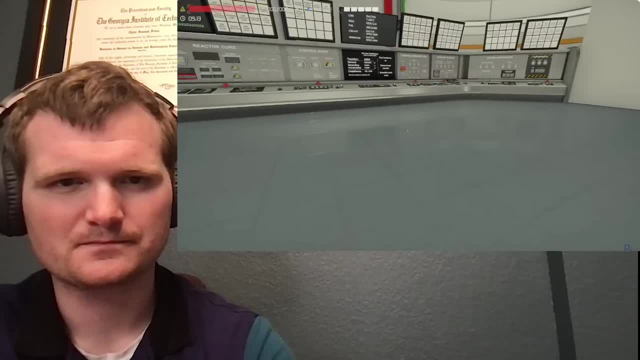 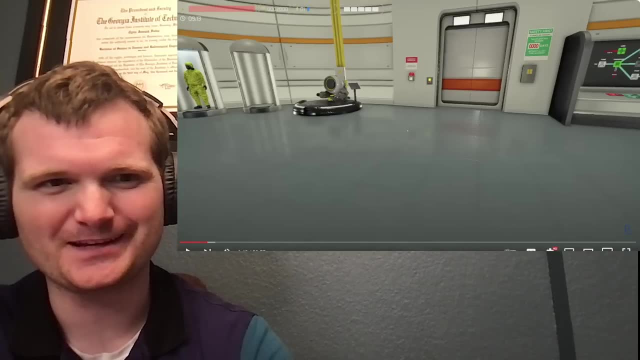 So what I'm going to do today is basically walk you around how to get the thing started. I'm also going to show you kind of what does what. All right, so Rick start up. Okay, that radiation suit over there in this really crazy with a mannequin. 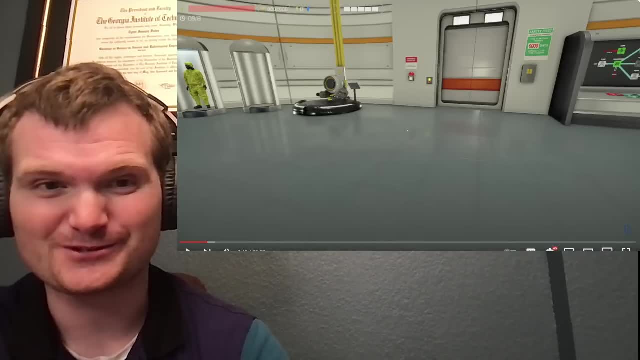 almost display like you're selling protective clothing. No, You don't see that. First off, you don't see these in a control room. The control room is not in a radiological controlled area. Now, it's not unheard of, but the control room would be one of the. 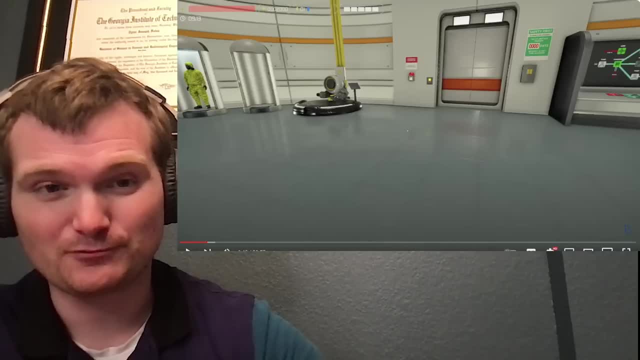 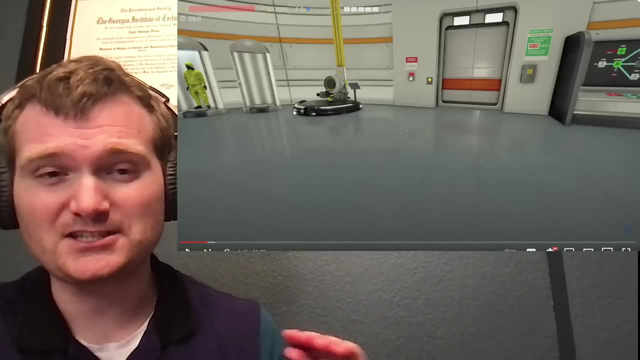 most difficult areas to actually get contaminated. Well, for one, it's nowhere near any sources of radiation, And even if there was a radioactive release, the control room is actually protected by an HVAC boundary that exerts a positive pressure over the room. 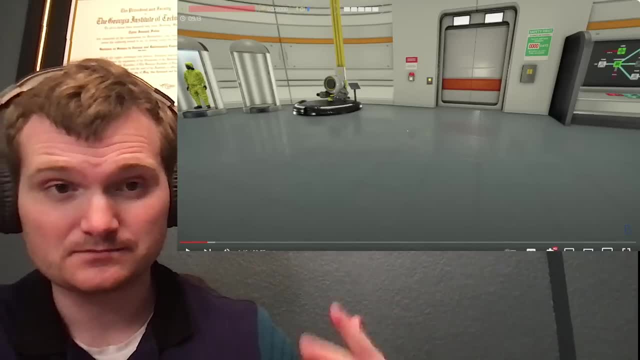 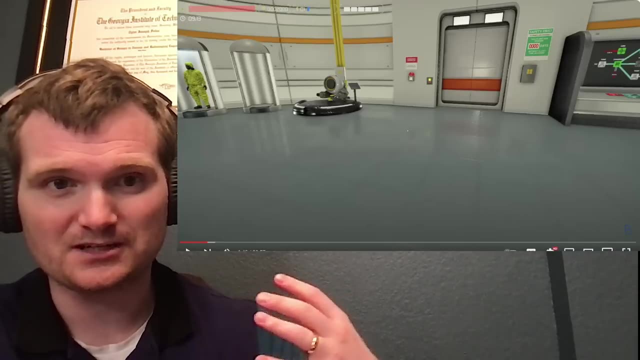 In other words, things are just going to get pushed out. So any contaminants that would affect the ventilation that would get into the air. that stuff is going to be pushed out by a back pressure in addition to a whole bunch of filters, in case any of it would slip through. 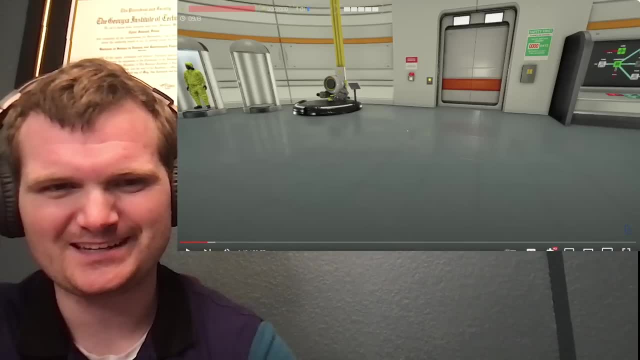 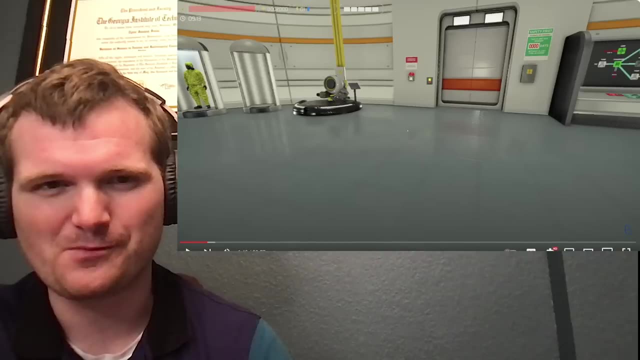 So you wouldn't need these in the control room, But I can tell they might have gotten some of this from seeing people working at Chernobyl, for instance. Well, Chernobyl is a horrible example, because they didn't even have a true containment building. 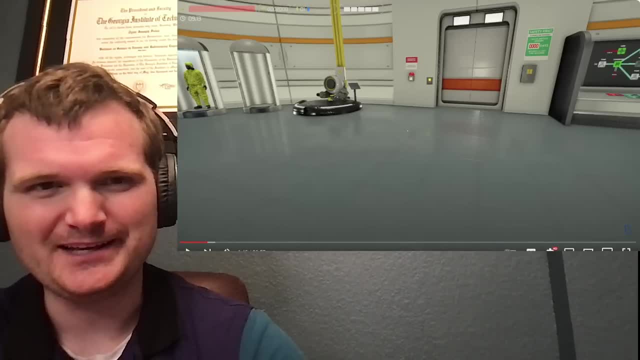 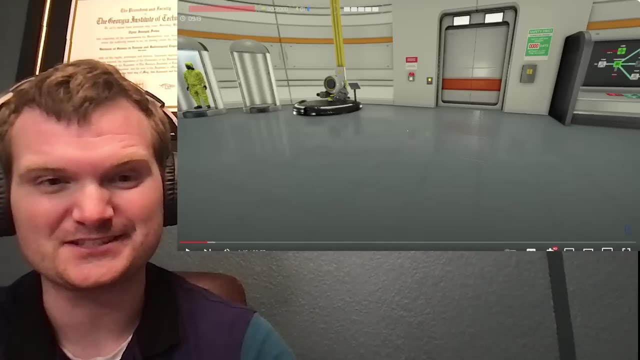 Right, So that's a whole mess. But even in radiological controlled areas I've never seen them on some type of display mannequin thing. They're typically in a pile just like any other laundry. It's an organized pile sorted by size. 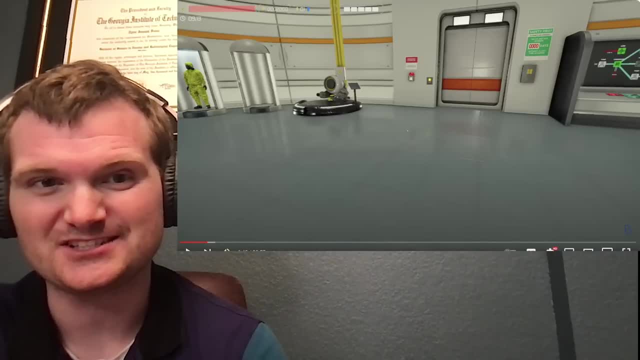 But you typically go through there and you pick which size that you need. So my first stop here, of course, is I'm going to run upstairs And then we're going to go take a look at the backup generator here. Oh, there's an upstairs. 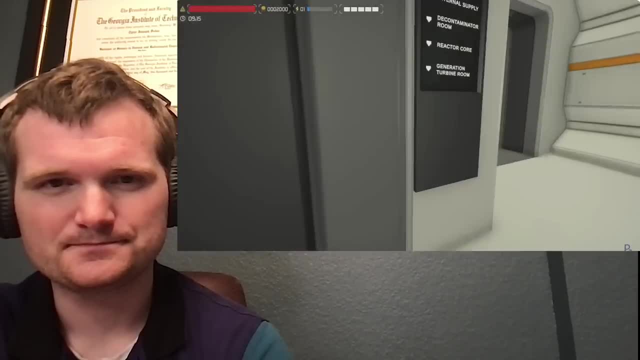 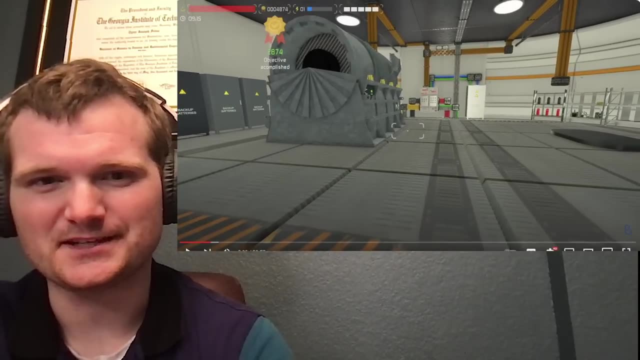 The way that this plan works- and again, I ignore my little bishop movement here, but look at how fast you go, Like this. So first thing we take a look at- of course that is something that's actually considered- is operator response times in their, their speed. 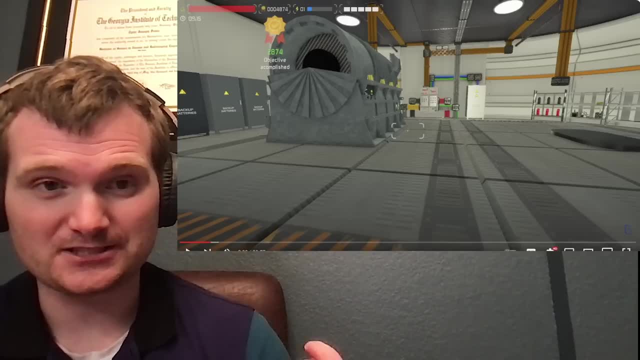 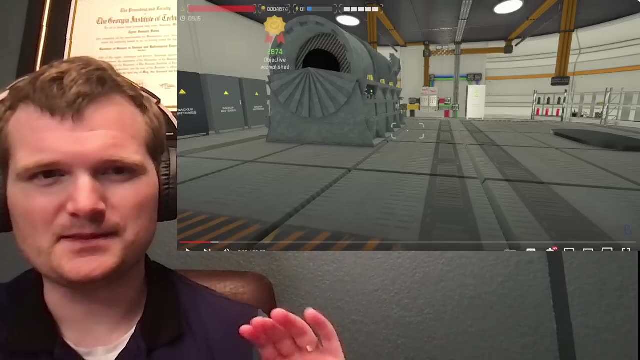 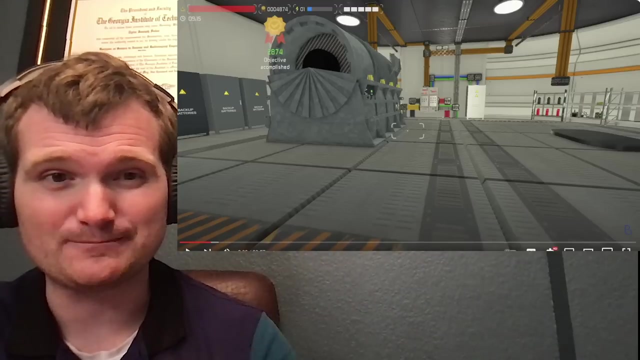 So being able to walk to certain parts of the plant to do important local actions that are important to safe shutdown. These are timed Now. this is now keep in mind. these actions are not required to be done to shut down the plant under normal conditions or even under a typical accident. 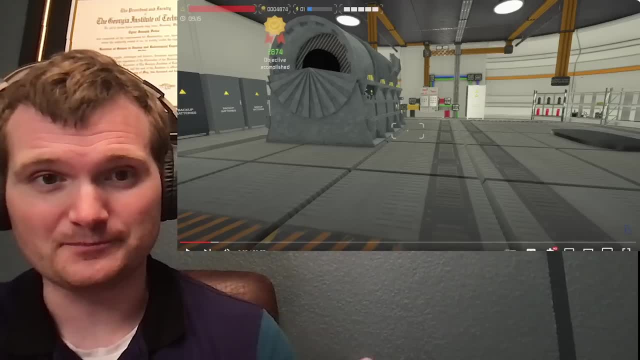 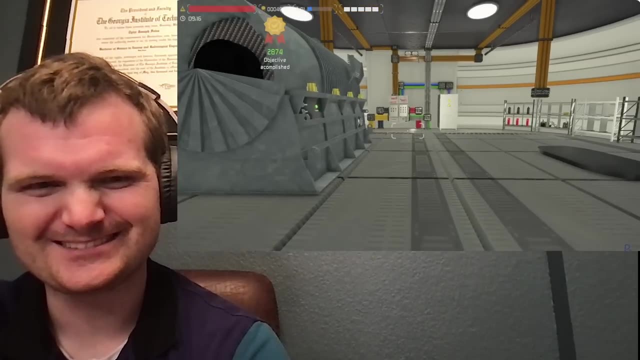 These are extreme scenarios. These are extreme scenarios where you'd have to do anything locally, But this person would probably set a record. I've never seen an operator scurrying up the stairs that quickly Is your internal supply room. This is where your backup generator is. You can actually buy up to two of these at a time. Now, the cool thing with the backup generator, of course, is it basically keeps you going while everything else is. You can buy up to two of these. You're going to want at least two. The plant that I worked at had three, And keep in mind each one of these had powered, everything you needed to safely shut down the plant, And the idea of just having one or two of these. you're going to want at least two. 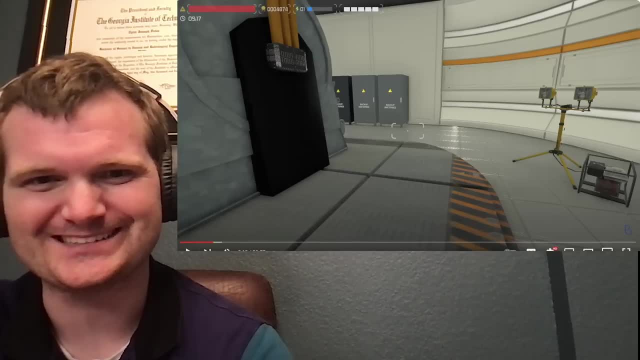 And the idea of just having one or two of these- you're going to want at least two- And the idea of just having one. No, that wouldn't fly today, Completely broken, so to speak. You also have these packs of backup batteries. 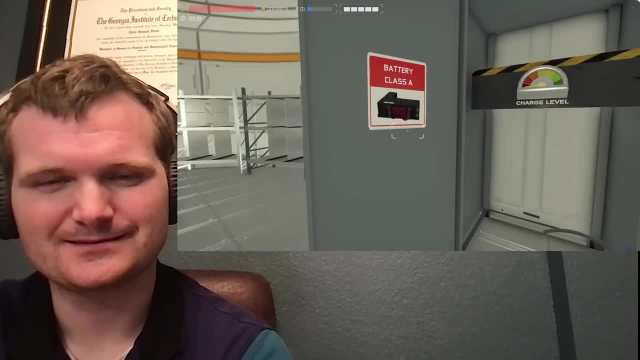 If you were to run over here and open one of these things, you'll notice there's none in here. The reason being is all of our batteries right now. If you wanted like 20 of these, you could store them, But realistically all your batteries are actually stored right here. 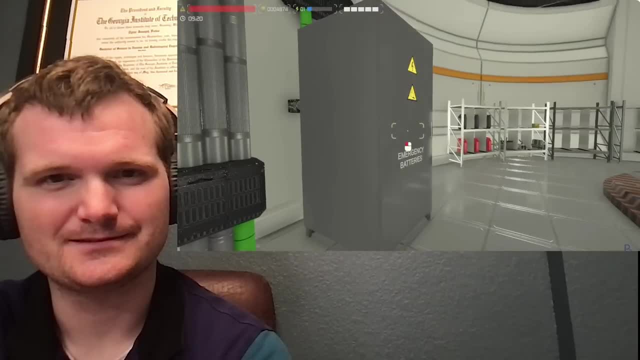 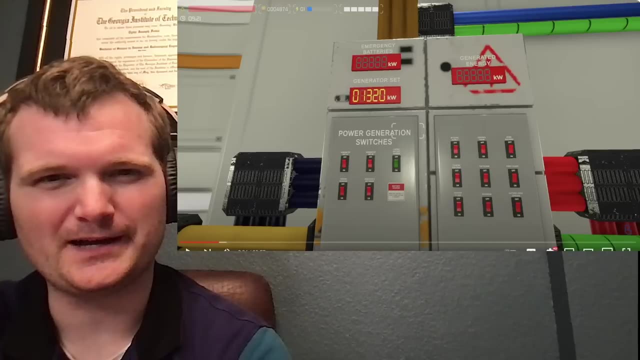 And you can tell by the charge level that they're doing well And we're not actually running anything off the backup batteries right now. Swinging here. this is your master breaker for this entire facility. here That sure means by backup batteries. he's talking specifically. 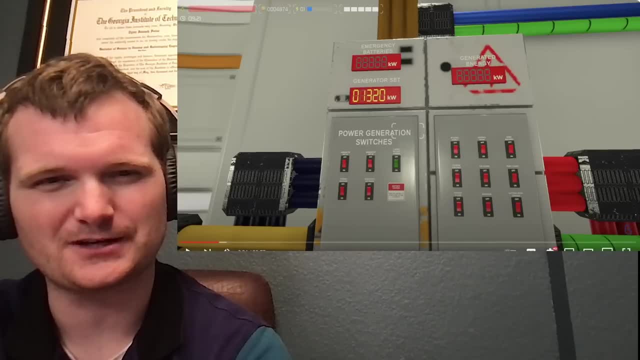 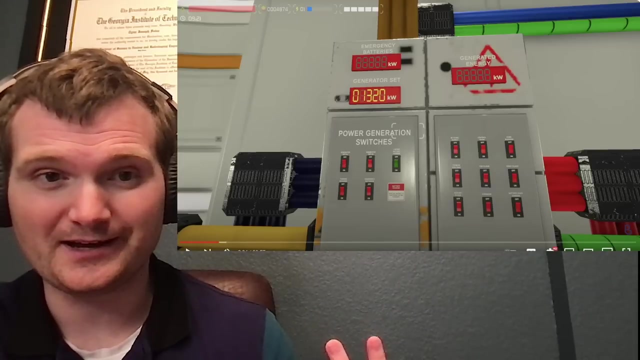 for the diesel, for like starting the diesel, Or if he's talking about batteries for the instrumentation, Because batteries for the instrumentation you typically have again a couple of options available, just like the diesels, And batteries would be in an uninterruptible power supply configuration. 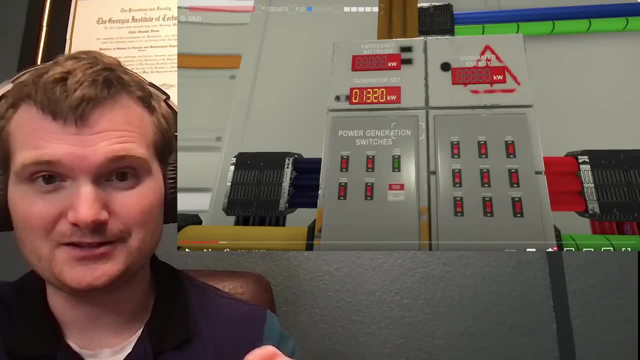 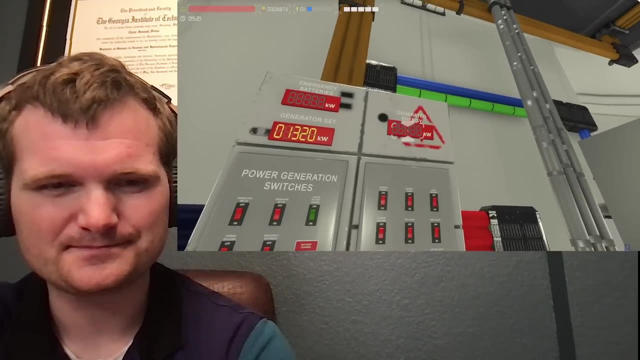 So if you do lose power, then you're still going to have access to your instrumentation, And then the diesel will start in about eight seconds. One of the things you'll see here is how much energy we're generating. You also have the power supply. 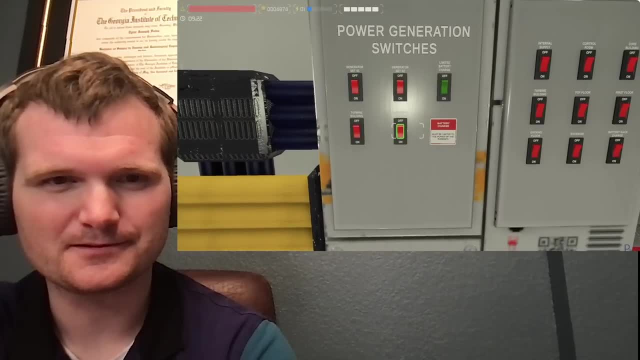 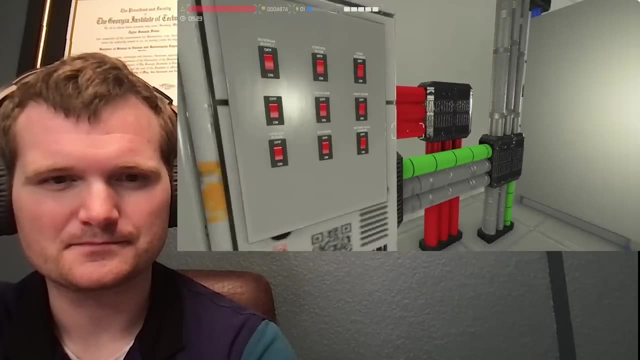 You also have the power supply Switches to turn everything on or off, should you need it, Like, if I want to cut down everything, I can cut the whole system off if I needed to. And again, if you're really, really, really dying for power, you might have to come up here. 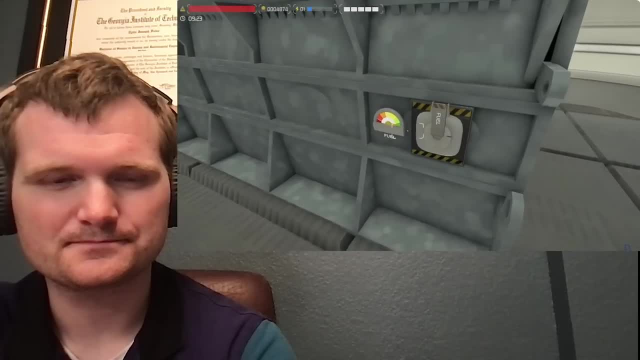 But generally, I don't think I've had to change that yet. One thing I do want to point out, though, is this thing does burn fuel pretty quick. This is, you know, it's a big angry diesel engine kind of thing. 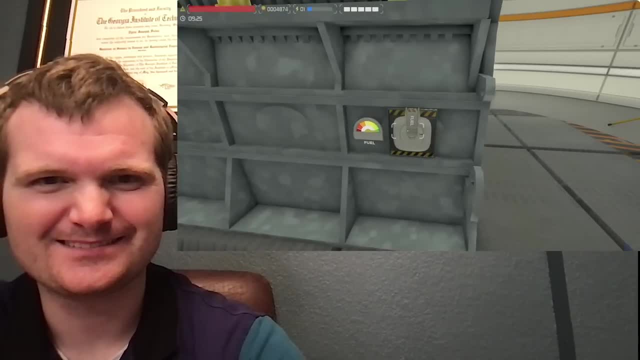 If you do want to put gas in it. a lot of people see this and they try to click like this and it doesn't work. The reason for that is you have to have a fuel can in your hand And if you just kind of left, click on one of these. 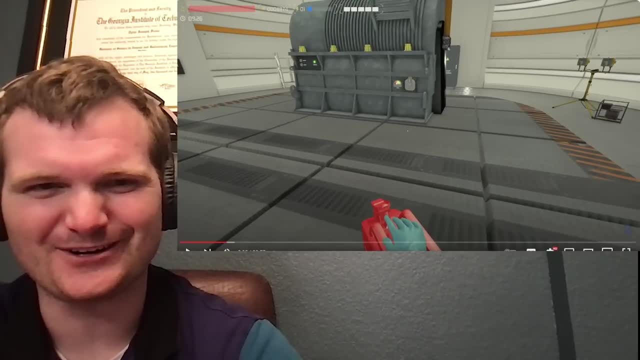 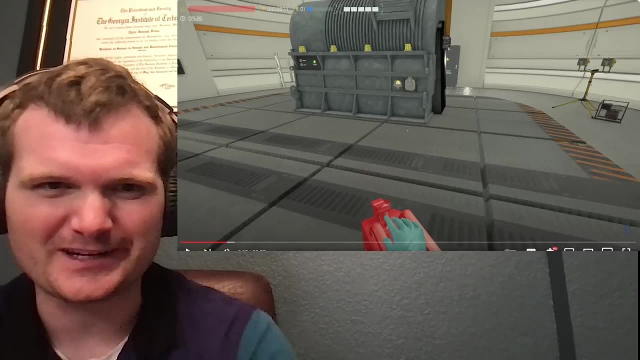 Oh, that's going to eat through those tiny things. So, so quickly. this will be for one. the diesel is a bit smaller than normal, but it's possible. this is a smaller reactor and you just might not need as many of the larger. support systems, but it's going to burn through gas cans. He's right about that. super quickly, to give you the sense of scale, The diesel storage tanks- each one- would last designed to last the diesel for about a week- over 60,000 gallons. 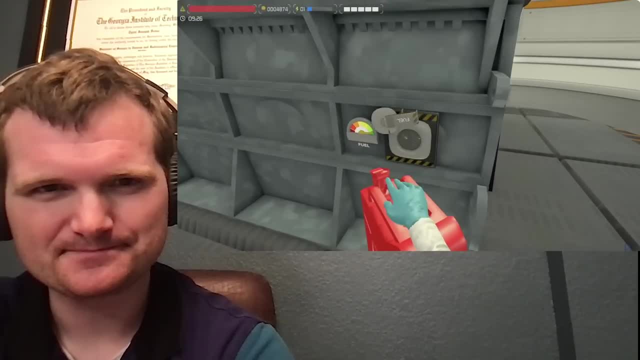 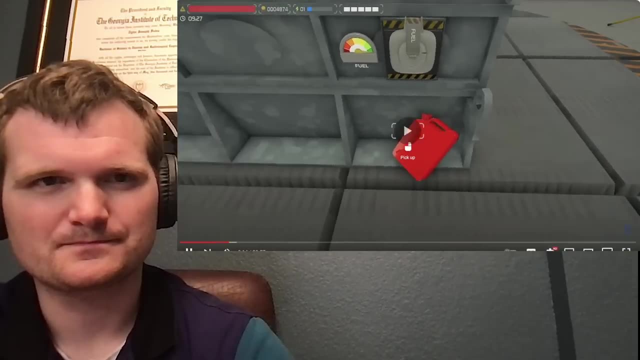 Yeah, of course, And run over And actually then press and hold. You'll see that he sits there and just splashes it in. Now, one of the cool things here is you see how this can is still red. That means it's still fuel in it. 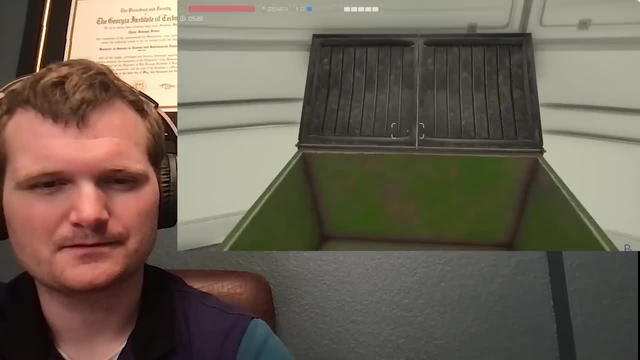 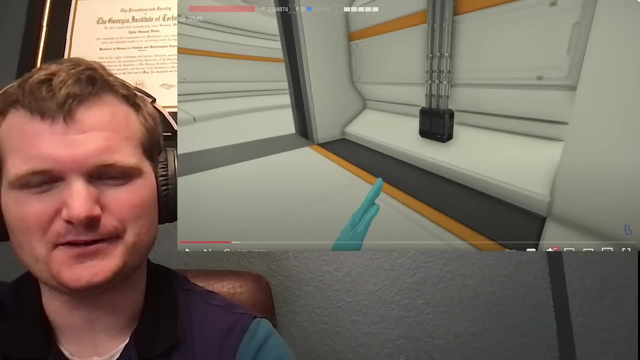 It'll change color as it runs out of gas And when it's completely empty, just run over here and dump it right in the dumpster And you're good to go. That's funny. The next stop, of course, the diesel would be filled. 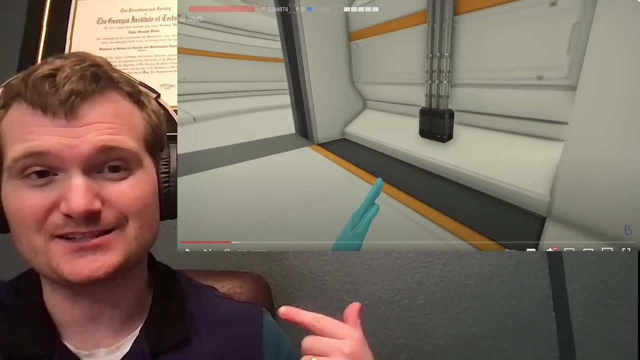 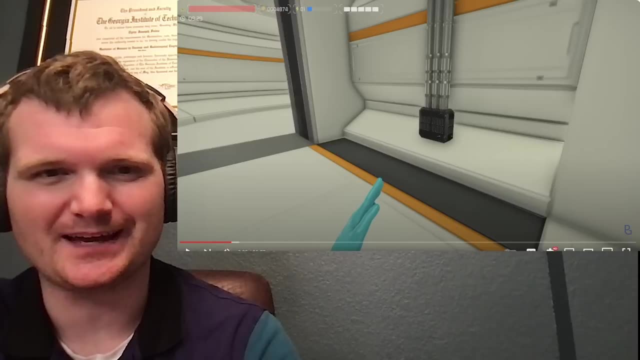 They would be pumped in, There would be an even larger tank. So I mentioned 60,000 gallon tank. There's a there'd be a bigger tank. That's I forget, but it's north of a half a million gallons. 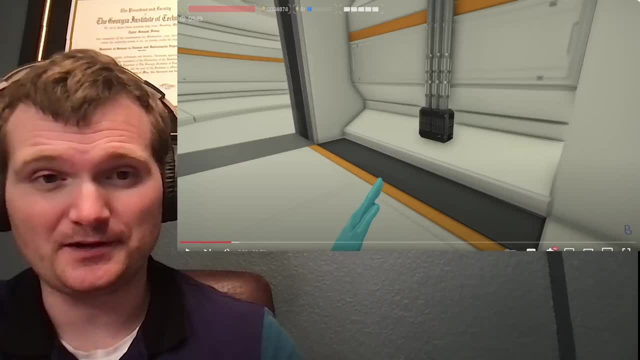 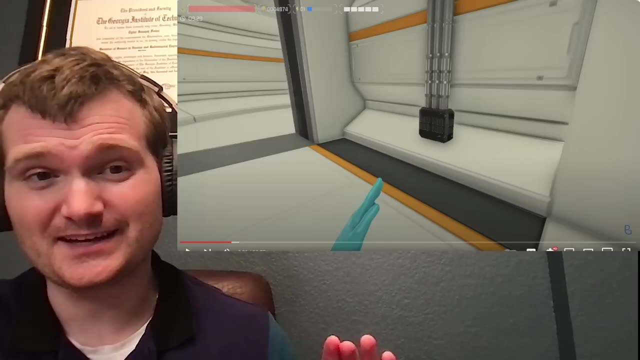 And you would just start pumps. You would pump it in through another tank. If you're having to fill diesels with fuel by hand, it's it's a bad day. They exist, These things exist, But what he's showing is probably similar to like a third string backup diesel that. 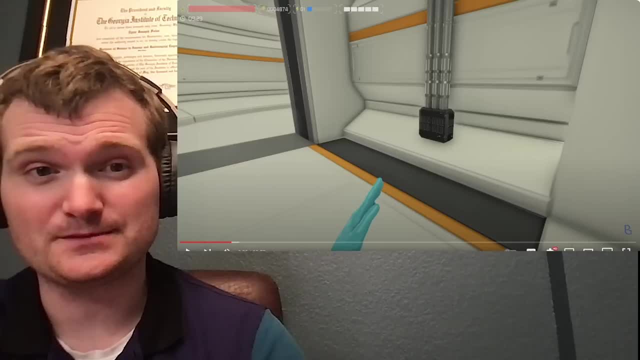 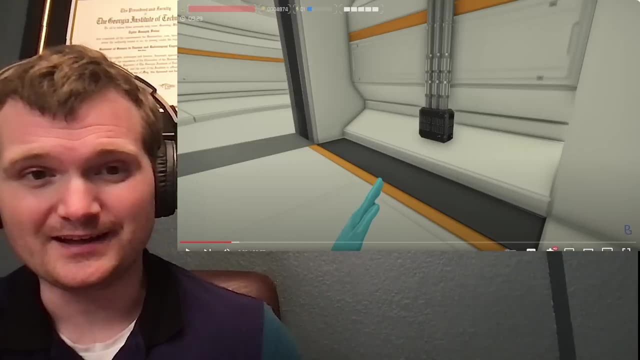 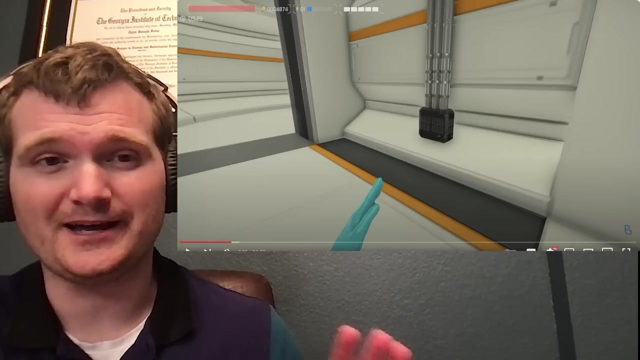 you would have in the event of a Fukushima type situation where all of your diesels fail and you need to bring in even more things and bring in hand supplies, piping, that sort of thing- But this wouldn't be Like in an in-house diesel generator after Fukushima happened. And the thing that happened there was the site lost all electric power, that including all of the onsite backup. So what was done in the US was we set up an additional remote facility that could bring in supplies such as diesels and fuel and is located far away from other sites. 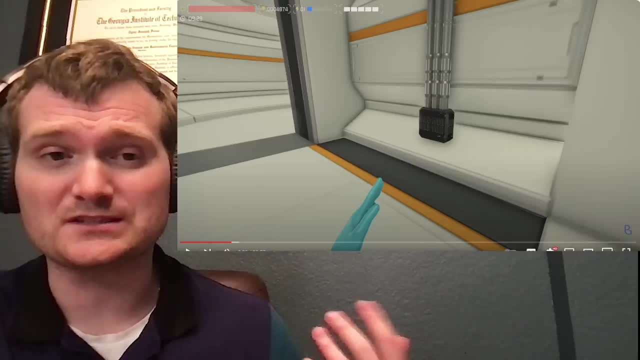 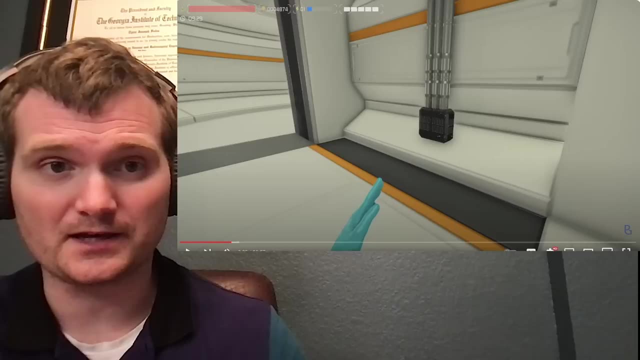 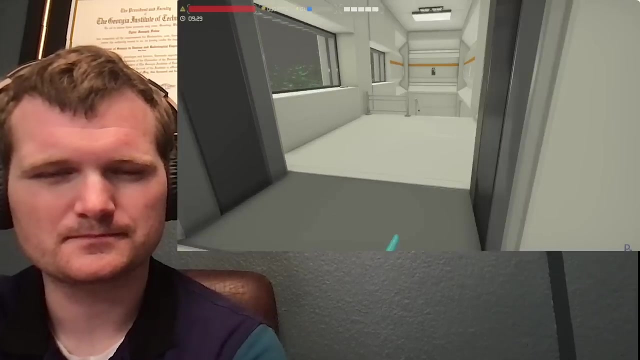 So in the event of an accident, or, Or Or A natural disaster, such as an earthquake or a hurricane, or something happens at a site and destroys everything, you could bring in additional equipment to to protect the reactor. Well, like I said, hilarious movement here. 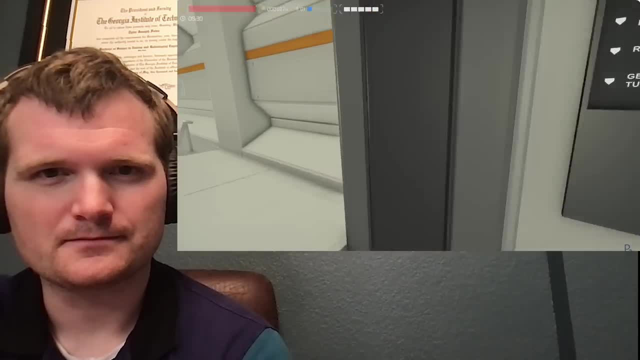 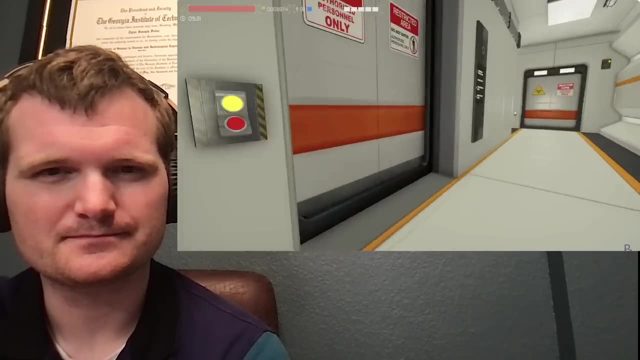 I'm sure the game developer is going to watch this one. This is a relatively tight-knit fast- and he's going to go: oh I should fix that. Please don't fix it. I like it the way it is. So we're going to run in here now and take a look at a couple more points. 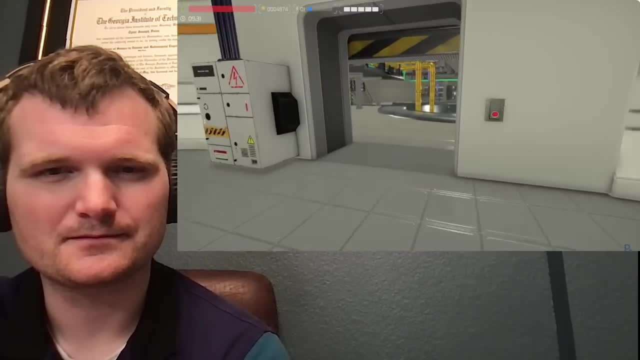 Right through here, of course, is going to be. our reactor is going to be through here And this is the reactor, Yeah, And you can stand right up here in the edge and look down into it if you want, if you want to be silly. 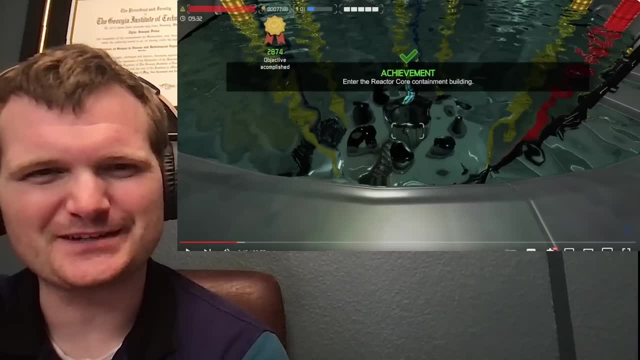 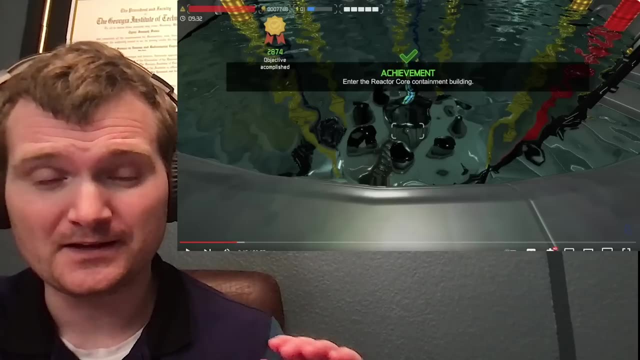 Enter the reactor core containment building. I don't know how much of a containment building this is. if the door is wide open, There would be an airlock to this thing, and a true containment building isn't just. you know, you can't go in here. 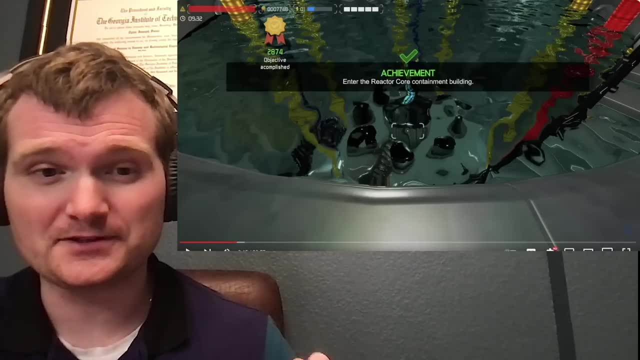 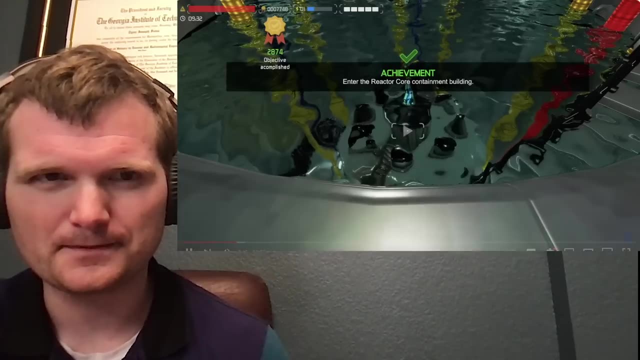 That would be more of a confinement building. A containment building is can withstand pressures, So the entrance is going to be an airlock, similar to what you would see on a spacecraft. Got no radiation points, No poison or anything. We're not generating anything. 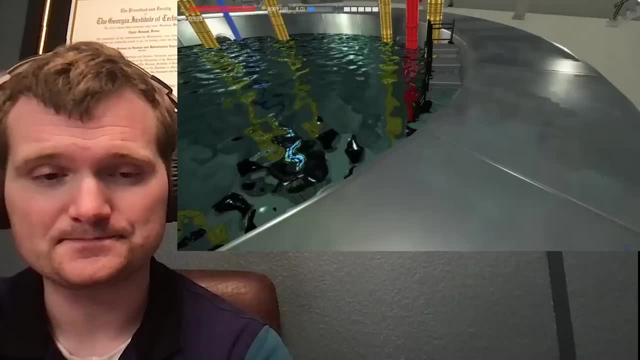 This water, by the way, you can't. They are shut down. So if you do something really stupid and just take a step into the water, you've just killed yourself, And in this game there's no what I call responding, if that makes sense. 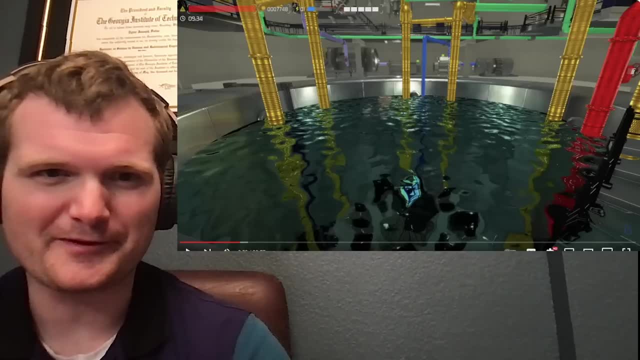 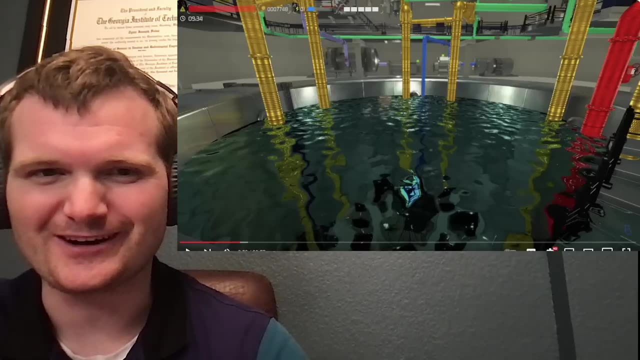 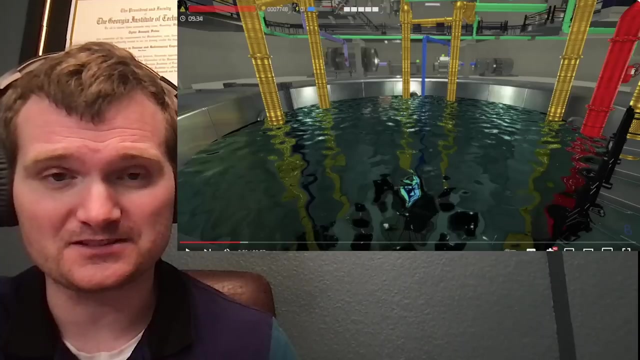 OK, this must just be a video game mechanic. There have been other video games that you talk: take a step into the water. You wouldn't bet. I've seen it kills your character off. but you could go in the water Now you still don't want to get too close to the fuel assembly. 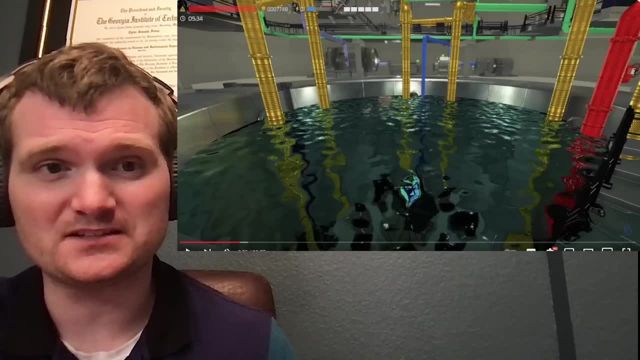 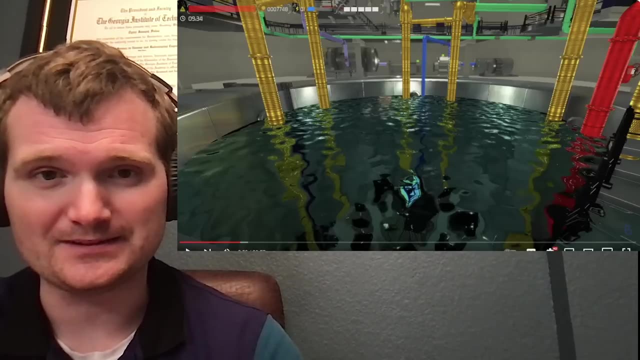 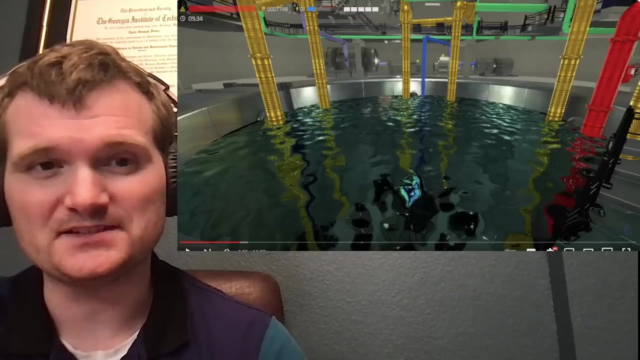 It's the Nuclear Regulatory Commission. The standard is 23 feet above the top of the fuel assemblies. is how much water between you and Ed? And this looks considerably lower if those are indeed the tops of fuel assemblies, Not to say it will become unsafe if you get less than 23 feet but you don't want to go. 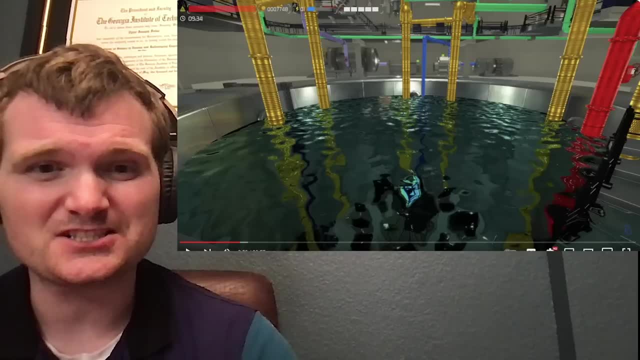 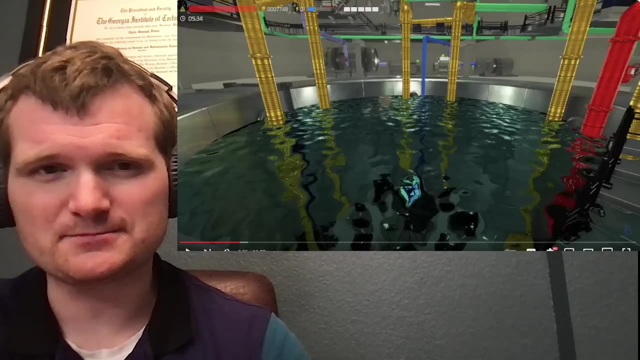 under there and bear hug one of these, because even though, while the reactor is shut down, unless it's entirely fresh, fuel You're still going to have, you're still going to be exposed to the fission products. A lot of times this fuel is is recycled and there's still subcritical multiplication. that 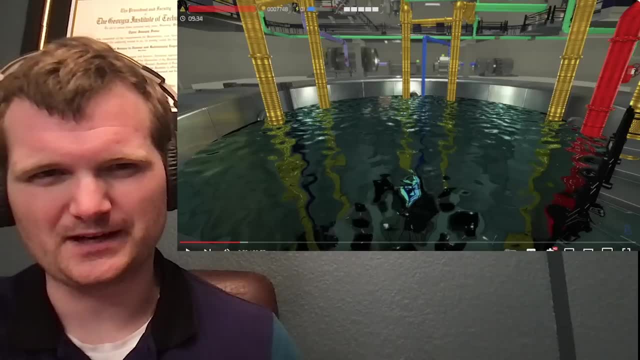 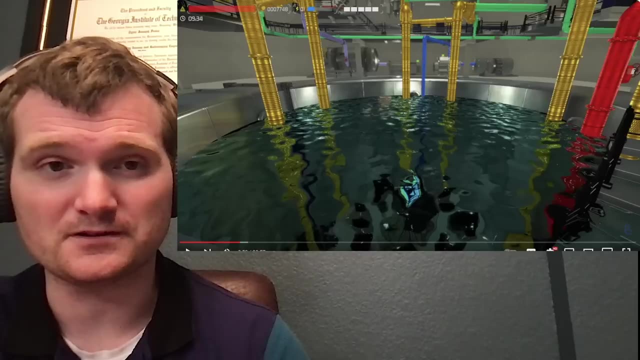 occurs. So some fissions are happening, but not enough to create a self-sustaining reaction. But yeah, you could potentially be exposed to a lethal dose if you were to go under and bear hug a fuel assembly somehow. If you mess up, you messed up. 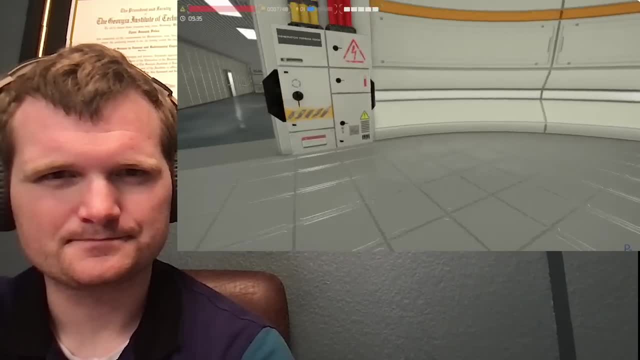 So it's just something you got to kind of keep in the back of your head. If you come down this hallway over here, you know it's going to take you to the generator hall. And keep in mind we're level one right now, with no prestige points. 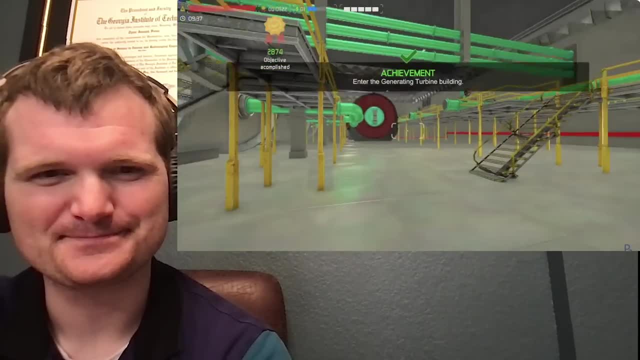 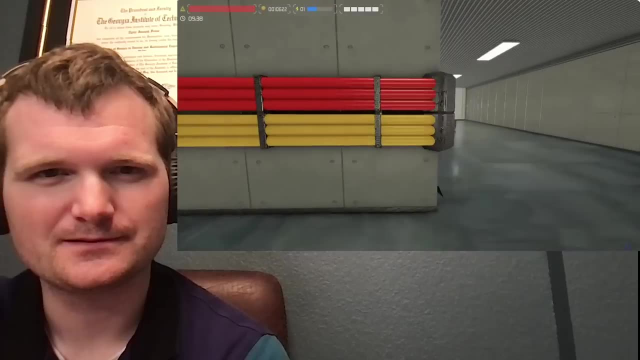 And now you can see this lovely room where our turbine generators will be, And with time you can actually add more generators to it. So like you're kind of version one of the reactor, if that makes sense, is really a version one of this reactor. 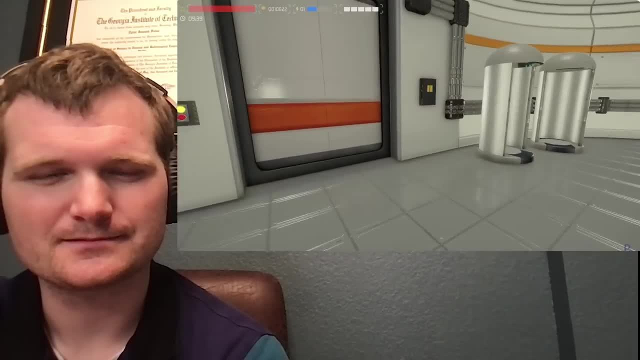 You know it's very much basic and you're going to add on to it over time And we'll take a look at how you do that. So this might be like SimCity or something where you upgrade your reactor by starting off like that. 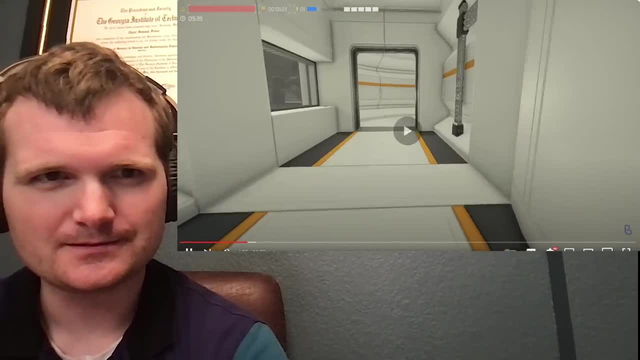 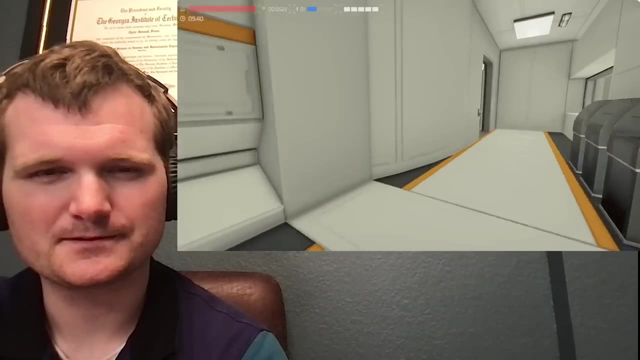 Maybe you can upgrade and have an actual container Containment building. Wow. So let's head up to the control room and start getting this thing rolling here. It doesn't take too much to get it going And, fortunately, the way they designed it is like you're going to be busy to say the 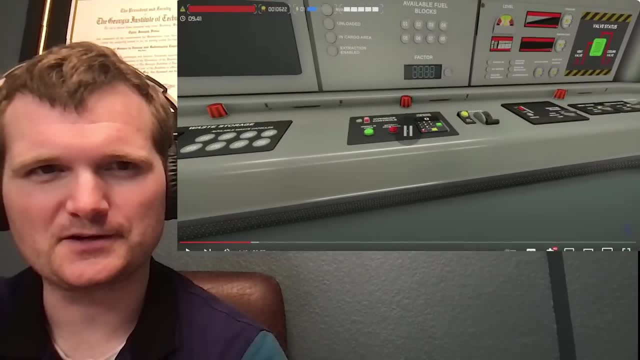 least. So the first thing we do is we're going to come climbing in here and we're going to hit. If you're going to have to do a reactor startup, you're going to probably have, at least within the control room, maybe four or five reactor operators. 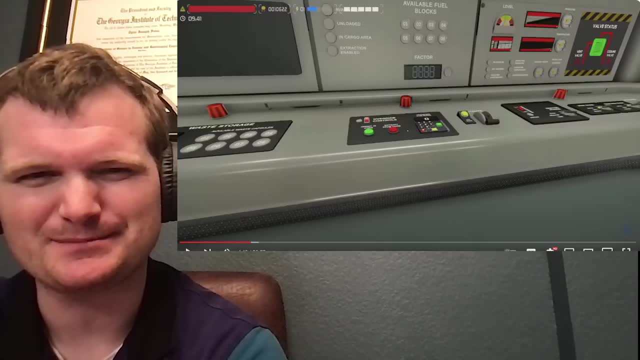 Technically you only need two, But at least at the plant I worked at I've seen about that many: Two or three supervisors, maybe even a couple of shift managers. You're going to have a ton of plant operators, basically guys that do things outside of the 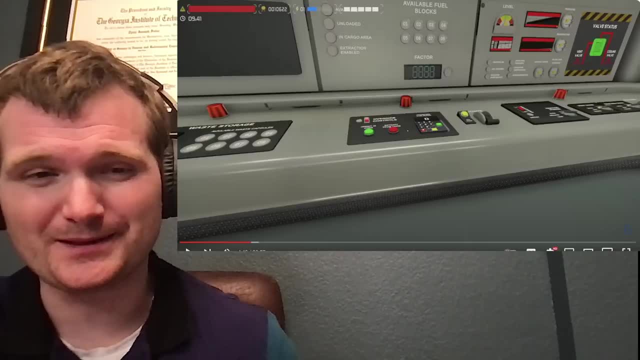 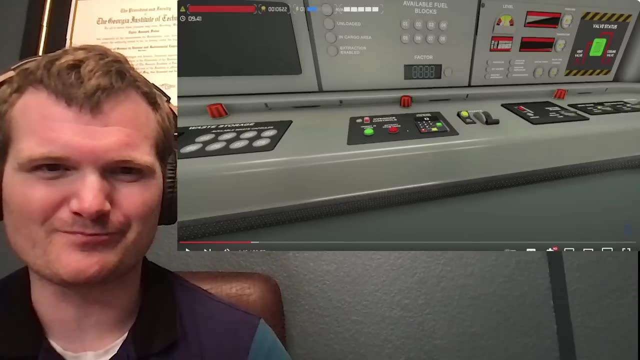 control room Easily easily 20.. And that mainly just because there's- but there's probably- a lot of things in this game that you're not, that they're going to skip just because it's less fun and more of sit up or just hurry up and wait. 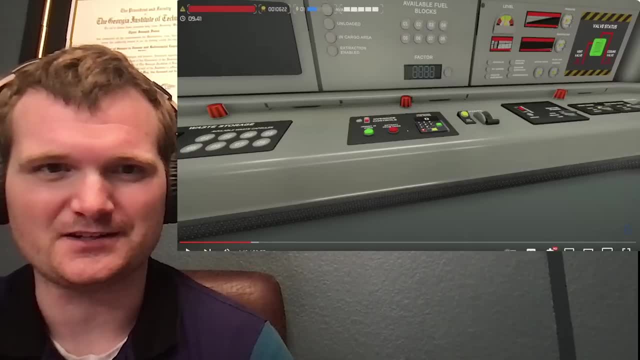 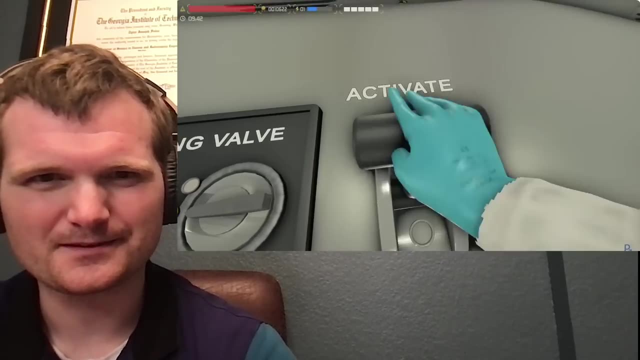 Like I doubt, this game includes doing a fill and vent of a heat exchanger in the turbine building, for instance. You're going to have a lot of switches and again, each one of these systems is going to have its own little switch on the side to activate it. 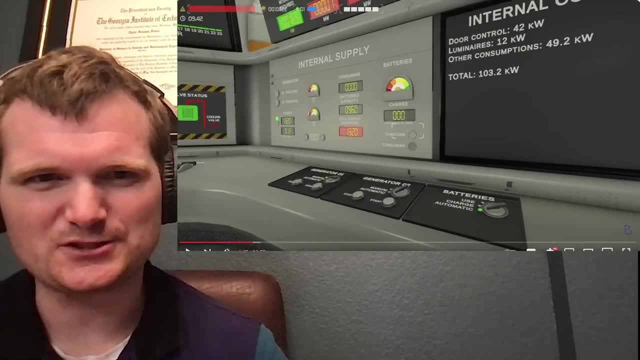 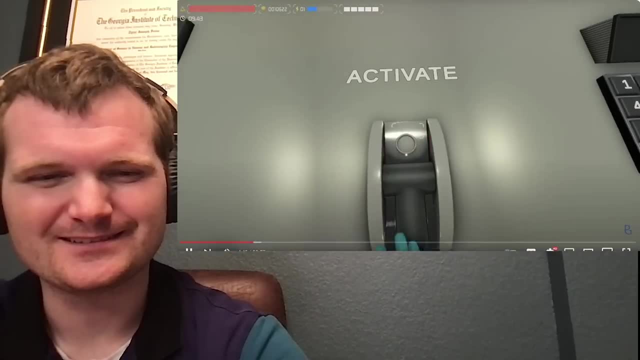 You want to make sure you set all these in turn. I've never seen switches that you push all the way forward like that. That's a little. that's a little different. Leave the batteries alone, Kind of a thing like that. Again, just come over here, activate it. 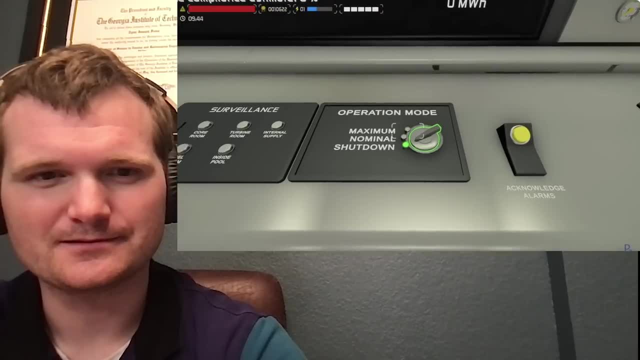 One thing I want to do- I'm over here- is I'm actually going to put the reactor on to standby mode. See this operational mode. I'm just going to, like that, Pop it over to nominal Nothing Operation. I've seen mode selector switches. 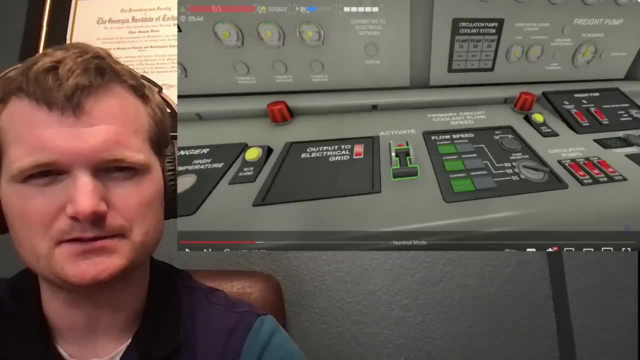 I mean. so that's at least taking something. Never seen the word nominal, though That'll happen, Don't worry. Go ahead and push that right there. That's going to click on. I'm going to go ahead and push that right there. 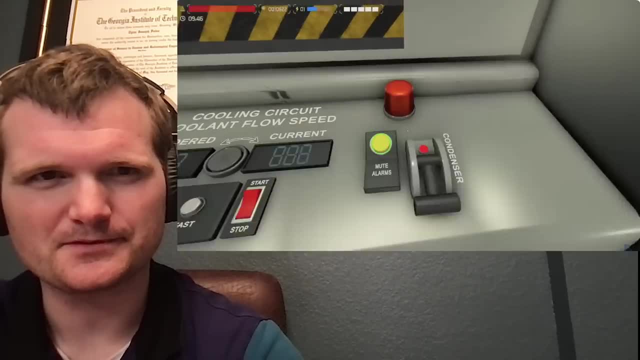 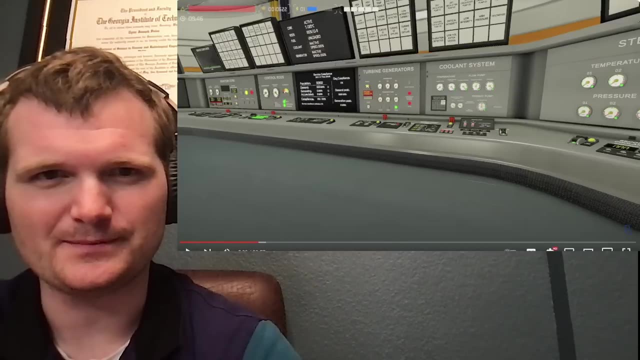 Snap that on as well. Here's our coolant flow, And again we'll talk about what all these are in just turning on the control panel here. You wouldn't turn them off per se, but I guess maybe he's probably going to get a bunch of. 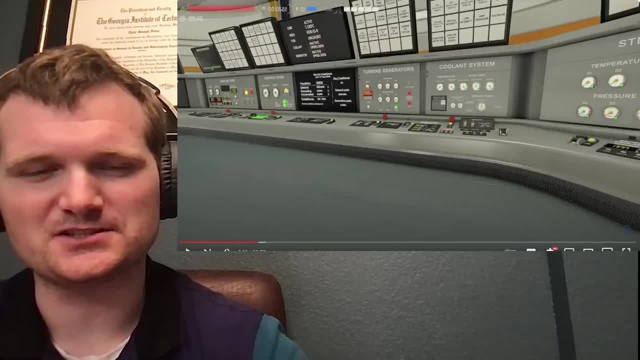 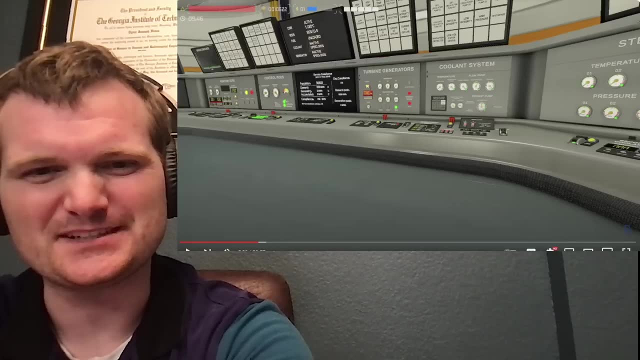 alarms now, since you know he's a lot of conditions, as, if I'm guessing, these panels assume you're at power and while you're not, so it's probably going to sense some things are out of way. Yeah, We have here is this whole panel is basically broken into multiple sections. 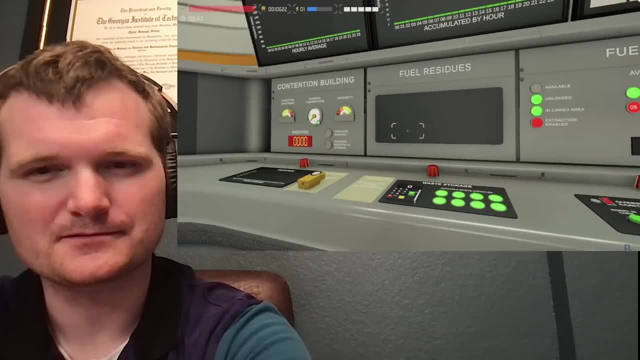 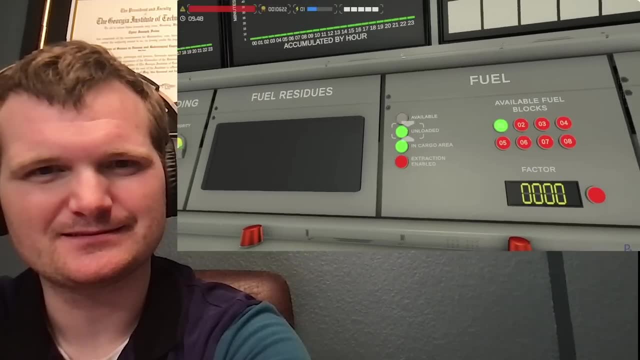 This is kind of- I sort of consider this to be the um, how was the best way to fuel? side of things, And, honestly, you're not going to spend a lot of time over here. The one thing we do do, though, is notice how it says it's unloaded, and remember how I pointed. 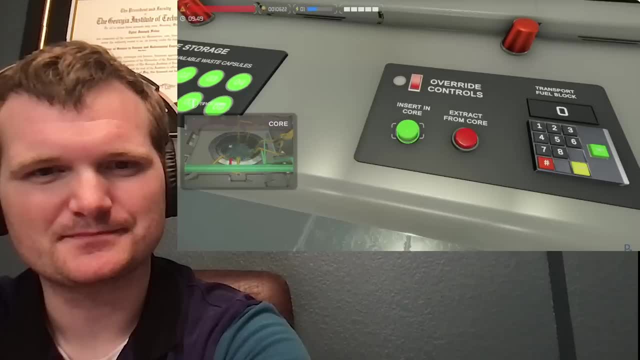 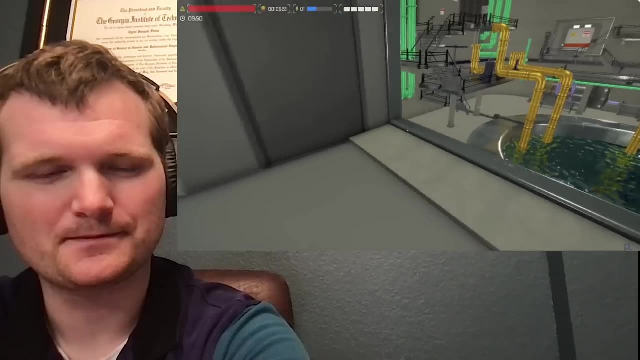 out that the core was still poking out of the reactor. You can actually come over here and push that button that plays this little nice video If you can actually watch the core be pushed in. And if you look at the top now, you can see that the core is now in the center of the 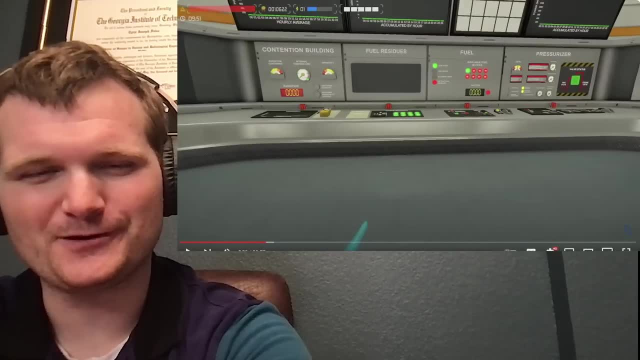 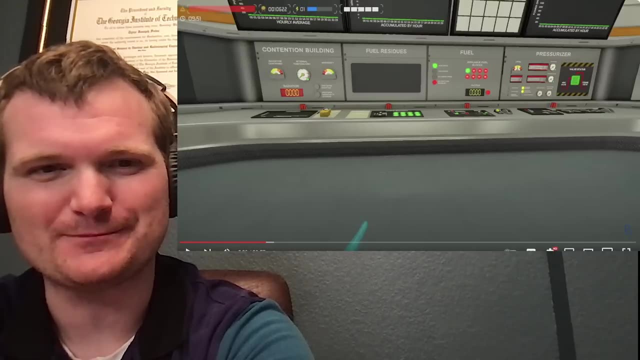 reactor vessel itself. So Yeah, Uh, that would. I've never seen. that would be so cool If you could just do that. usually it's a bunch of highly trained people um operating cranes and delicate, uh, lifting equipment. 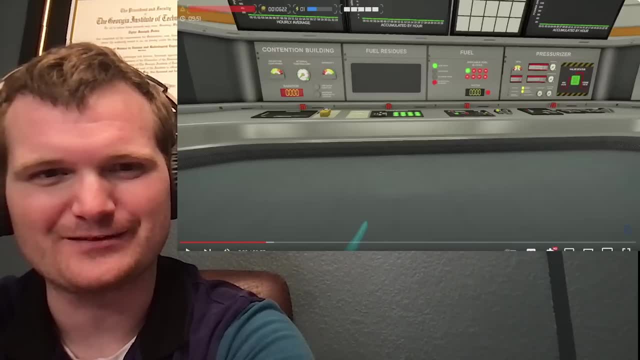 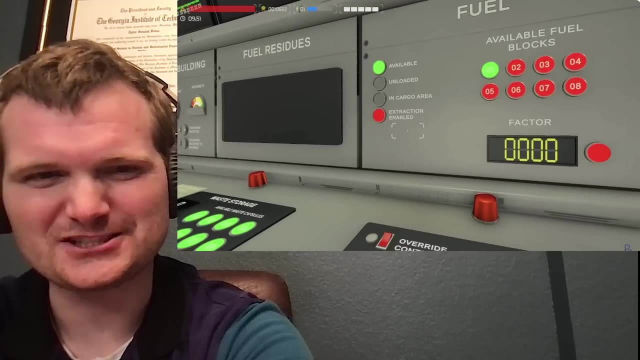 And this sort of operation of putting the core's head and everything back together can take several shifts during an outage Need to go If we needed to extract. that, of course, keep in mind you can't pull a dead reactor core out. 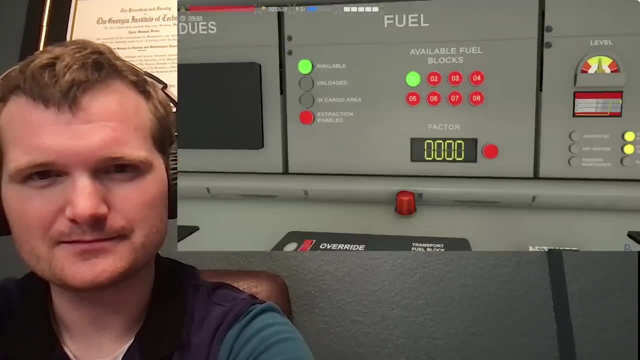 Again, these things will last for days of game time, So don't worry about ripping it out just yet. But keep in mind, if you did want to do that, we'd have to actually empty the whole reactor, and it's such a process. 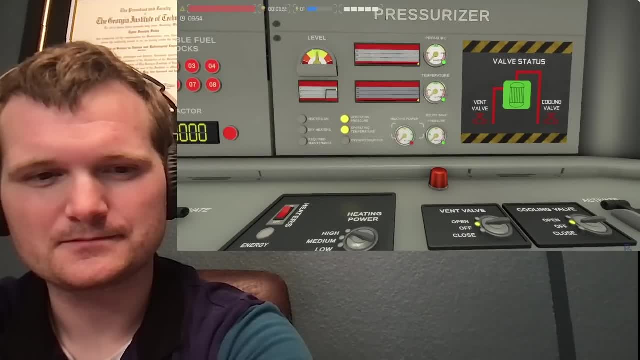 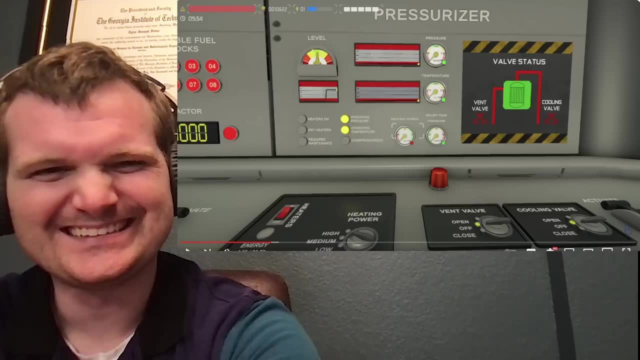 So this guy right here is our pressurizer. This is a pressurized water reactor, Basically Okay. If it's pressurized, how it? why is it vented to atmosphere? That's what it needs: to be bottled up inside of a vessel. 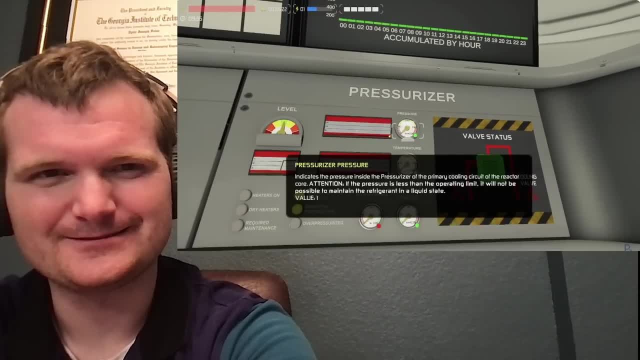 This is going to do is it's going to build up enough pressure to kind of keep things going And notice what it says. If you don't keep the pressure up high enough, you can't keep the refrigerant, you know the coolant, the water and basically in a state that's liquid it'll do other things. 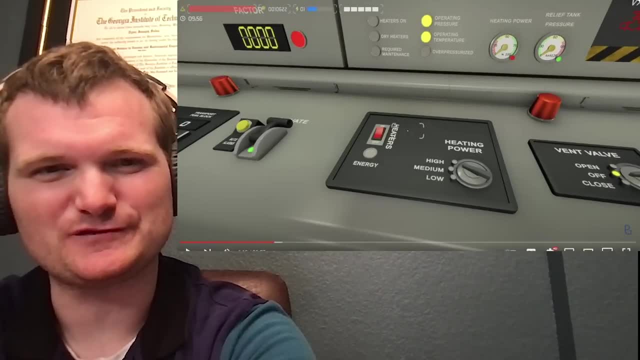 So never heard anyone refer to it as a refrigerant. No, it's a, it's a coolant. Now, boiling doesn't occur in a pressurized water reactor, but it doesn't within the normal reactor coolant system, but it does within the pressurized. 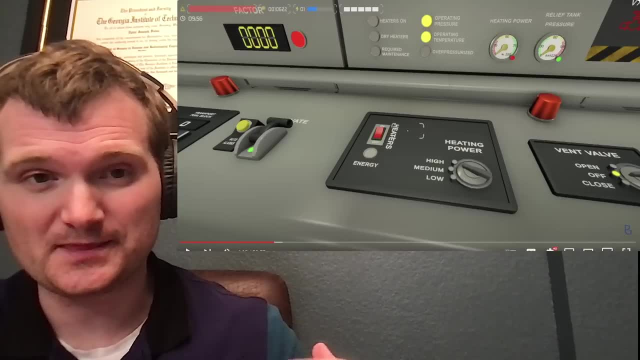 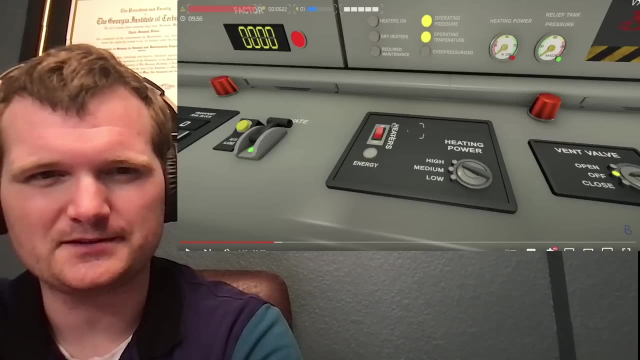 And that's how it. it basically creates a bubble that pushes down on the mass of water in order to bring it up to a higher pressure, And it's I'm not surprised that they're using a pressurized water reactor, Cause I'm assuming again, nuclear is Portuguese. 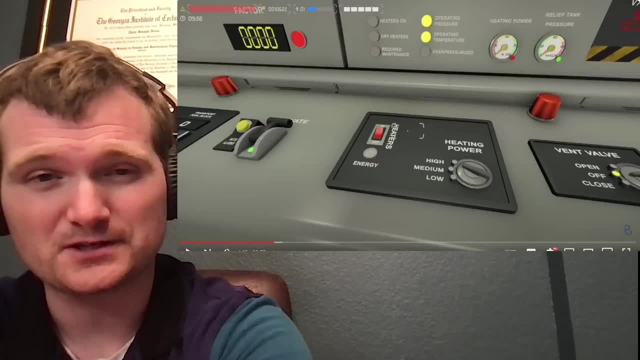 Portugal doesn't have any and Brazil's two reactors are both pressurized water reactors, So that kind of makes sense. But again, unless they show that um, the reactor being bottled up, I don't see how you're going to have a pressurized water reactor. 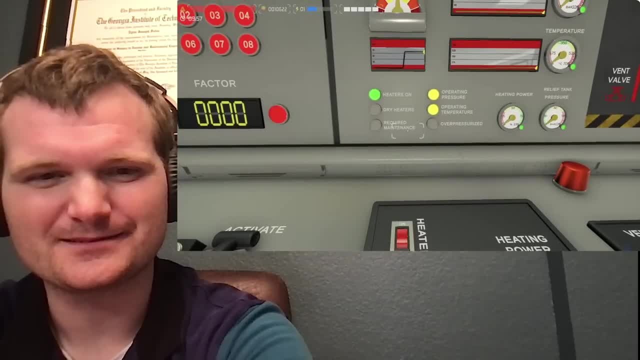 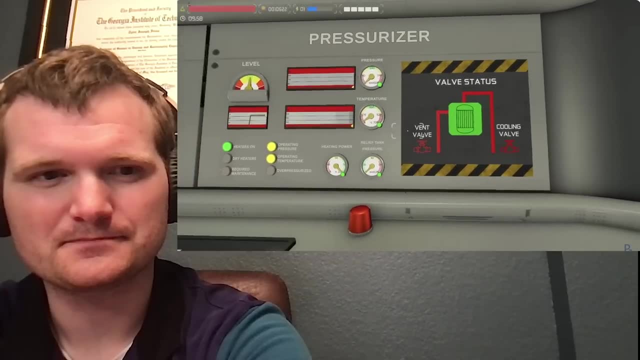 We're going to do is we're just going to flip this sucker on real quick And this is going to start using quite a bit of electricity. What it will actually start to do is it'll start heating up the whole pressurizer side of the reactor. 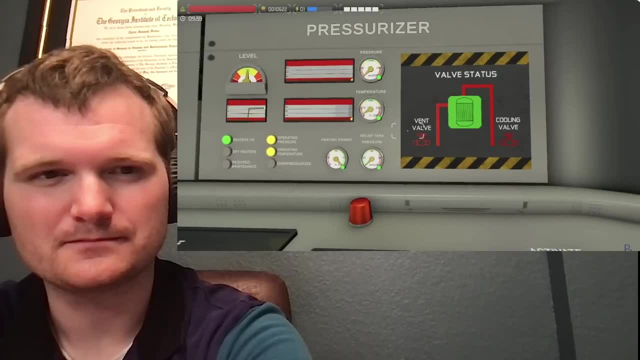 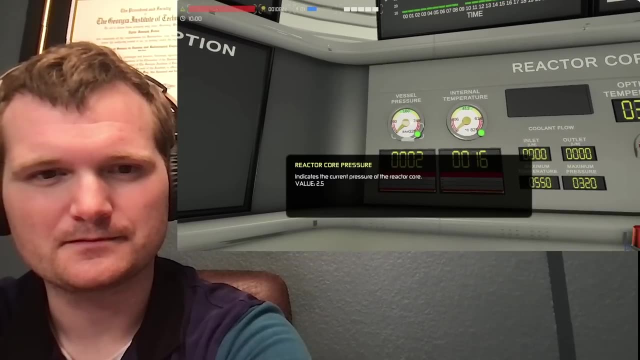 Now we need this to be warm to generate any power, And we also need this to be warm to basically get things cycling. This thing heat up the reactor. come over here and look. you can actually see how the pressure is starting to build up on its own. 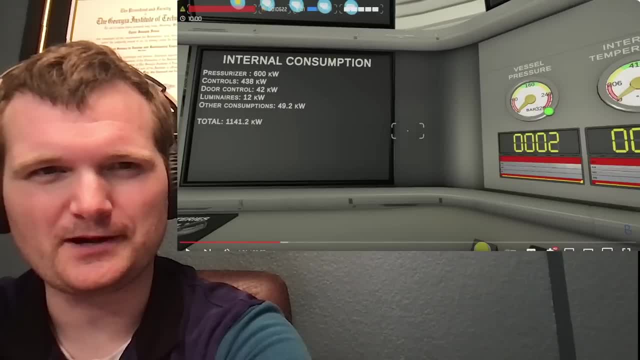 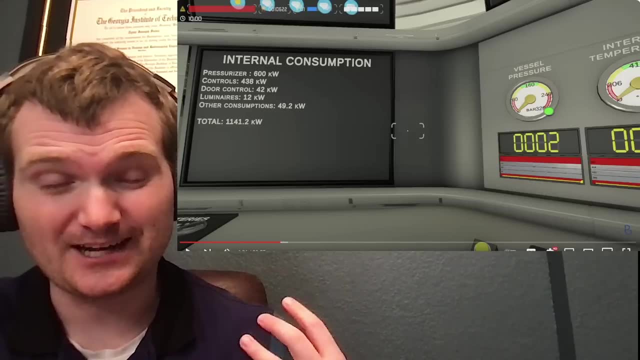 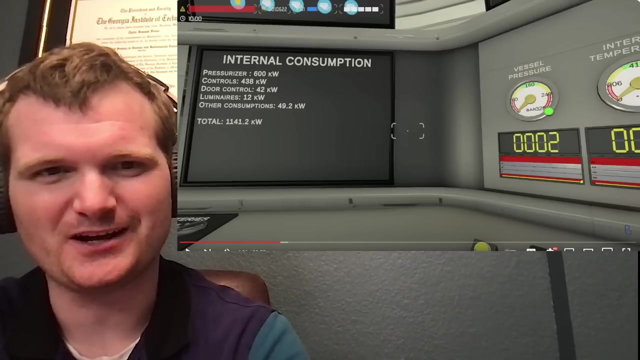 Even though the reactor itself- we haven't even set the reactor off, So apparently it is- the vessel is close. Maybe the vessel is just submerged in water, Like the water is outside of the vessel and the pipes are going in. I've never seen that, because otherwise, yeah, if you're turning on heaters and the pressurizer. 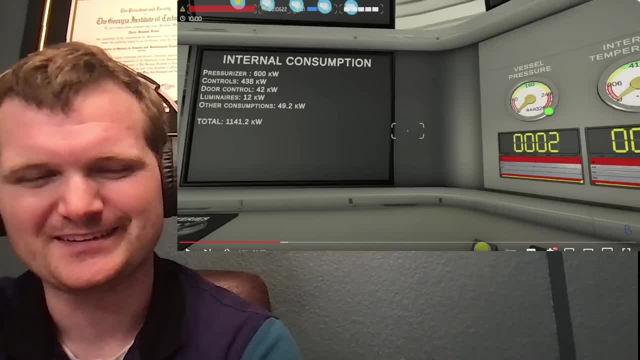 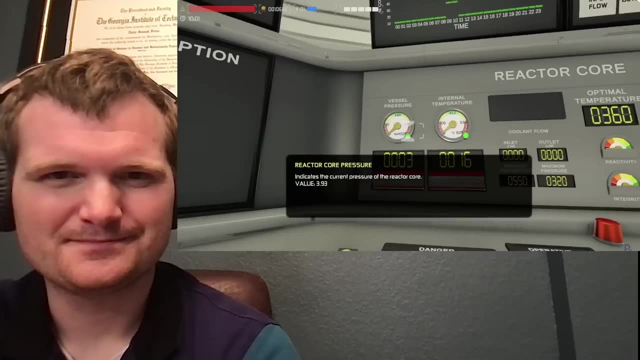 without the reactor system being put back together. It's not going to do you any good. So no problem there. This does take a while. It's considered kind of bad form to get this up to temperature before this has got a little bit of pressure and temperature. but the good news again is we're just running off the internal. 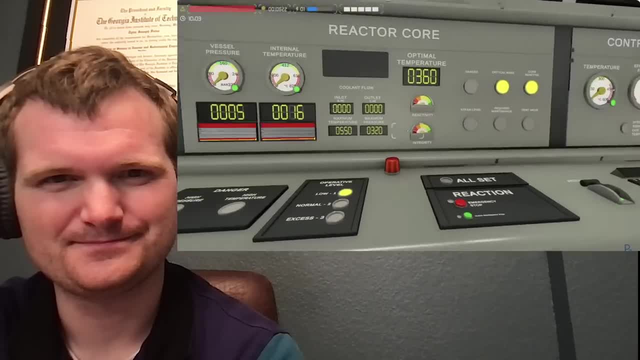 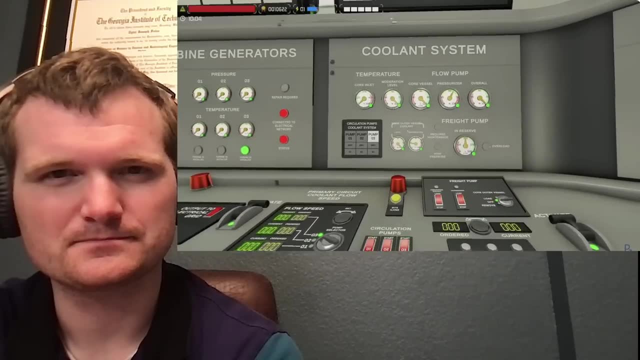 right now And, by the way you can see, we're just burning down right now, So I'm gonna leave this alone for now. We have the control rods- We'll get back to that in a second- And then, of course, we have our turbine generators, which we're going to leave alone for a second. 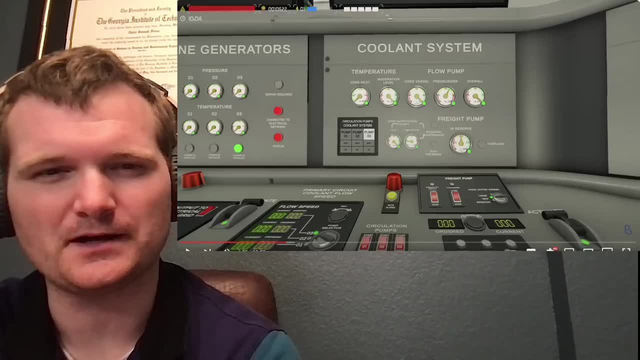 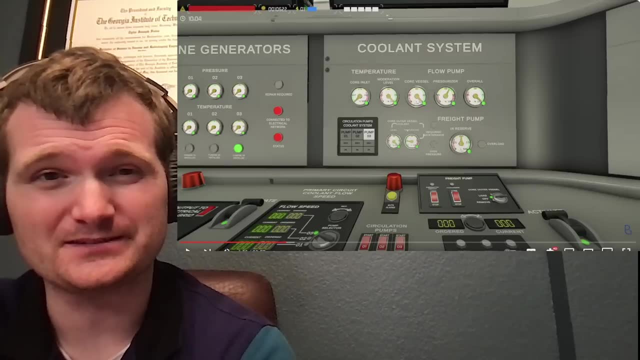 but now we're going to float over to the corner. Oh, it's floral, So he has multiple generators. So the plan I had had- Yeah, It's just one, really, really big one, but it's not unheard of. Nuclear power plants do produce a lot of electricity, so you can have multiple turbines, multiple. 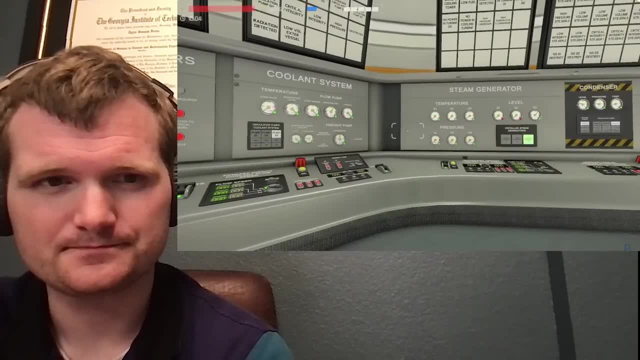 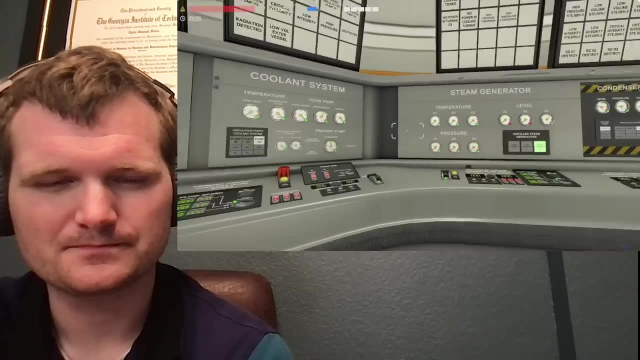 generator systems set up into the system. So basically I'm gonna kind of put my head here. I wish I had a little mouse I can show you kind of what's going on here. but our coolant system takes heat away from the reactor. 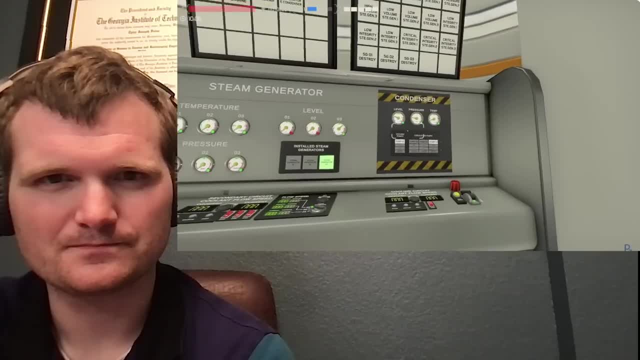 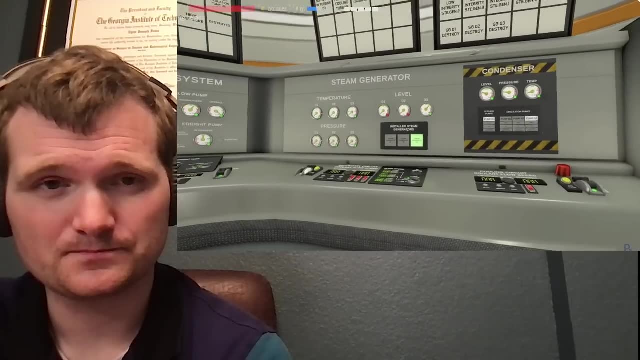 Our steam generator takes heat out of the coolant and our condenser cools everything back down so that this process here can be cycled. That's exactly right. This side of things is basically one giant loop. This is the one that's actually going to be pulling heat out of the reactor for the 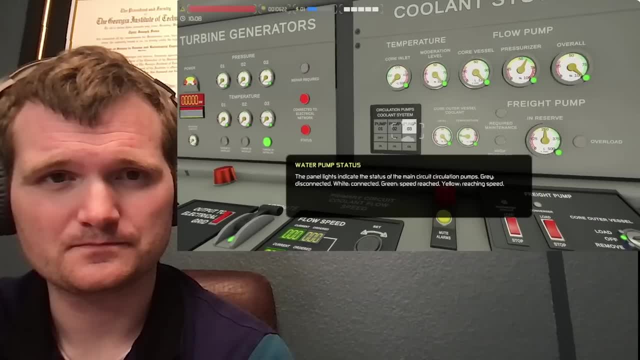 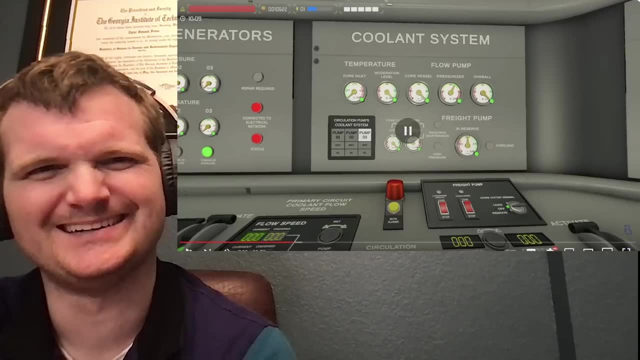 purposes of getting work done. You know, you can notice right now in this game we only have pump three. You know, once you spend your prestige points, you'll have three pumps here, and it makes a huge difference as far as how hard you can. 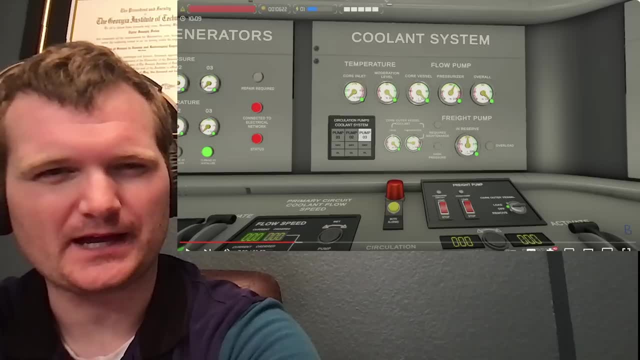 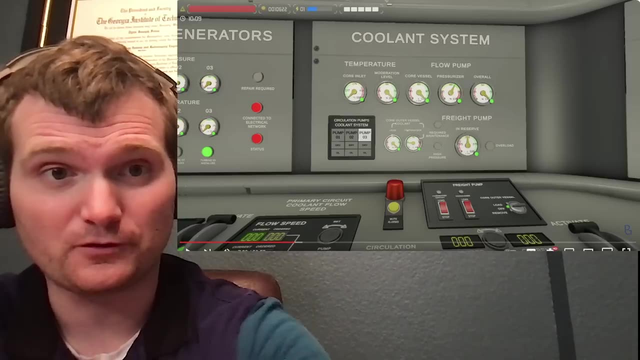 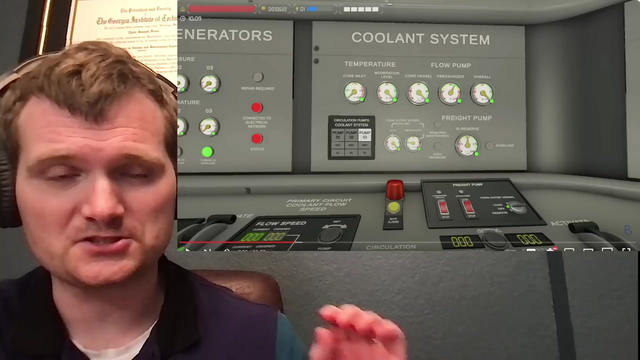 Prestige points. So never seen it where a reactor is done incrementally. So the plan I worked at had four loops, So four reactor coolant pumps, four reactor coolant loops, four steam generators, though they would all The pipes would all combine into into one header, go to the, go to the main turbine. 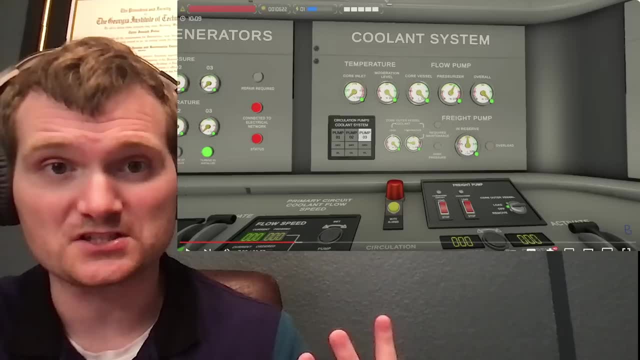 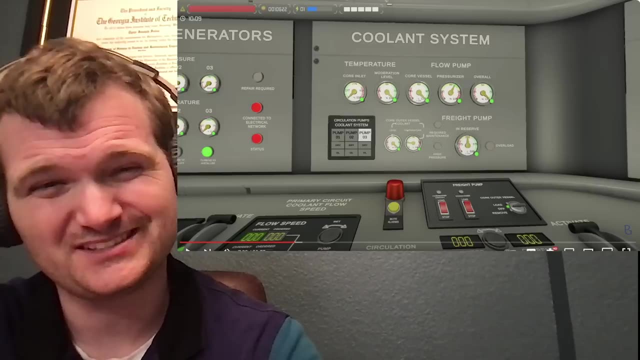 to the condenser through the feed water system and then back around, just like you said. But it never started off as like a one loop plan, a two loop plan, a three loop plan. So this was a three loop plan, which is, I see, what I did there. 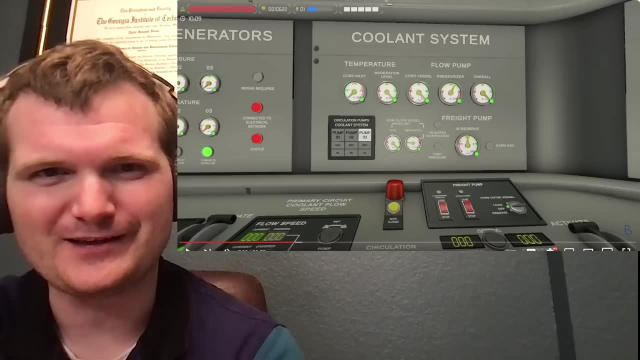 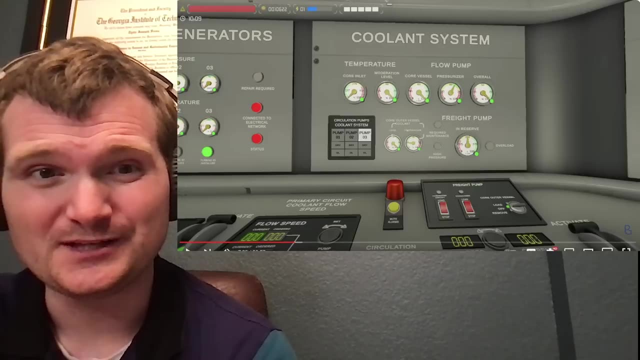 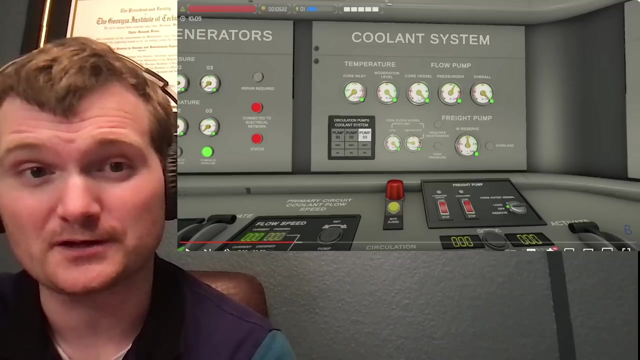 But yeah, I've never. I've never heard of that. If you were to do something like this, it would involve complicated licensing processes where you would probably spend just as much on engineering and design calculations as you would on the actual materials to upgrade your power plant. 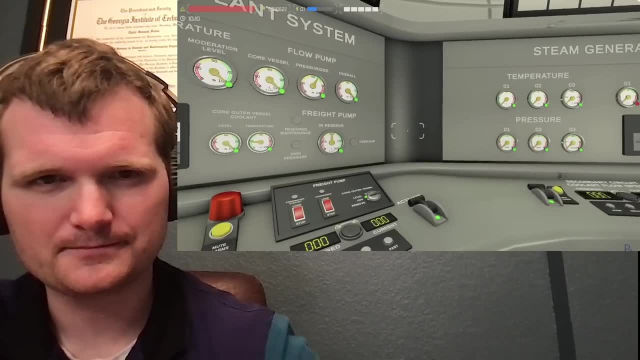 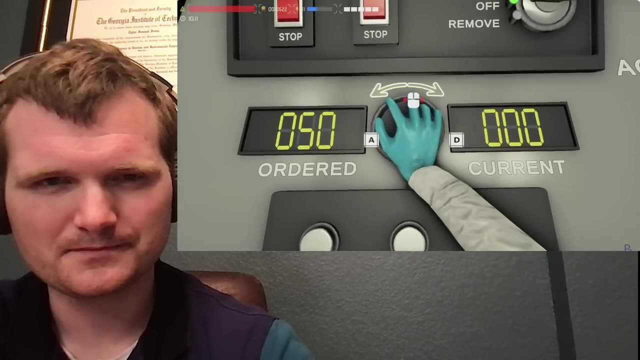 Run this and I'll hot. You can get everything at the beginning of the game. We're pretty basic here, but what we want to do is you do want to start to get some cool and going. Now. a lot of people, of course, like the mangle, that button is set to 49%, just like. 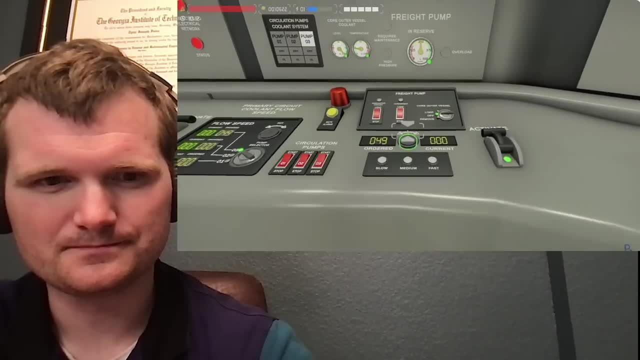 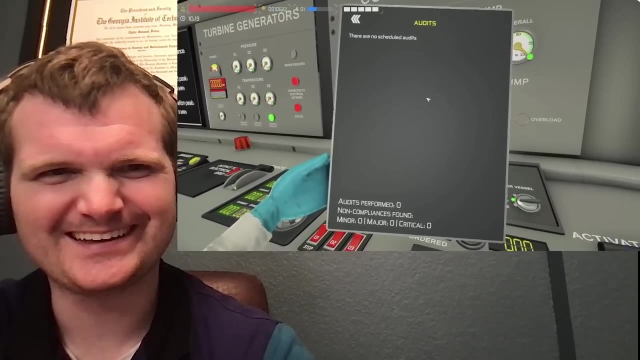 that, Um, people like: wait why? And of course it's one of those things where you don't worry about it that much. You have these things called audits at the tab. Oh, that's fun Once in a while. You must do this or you must do that. 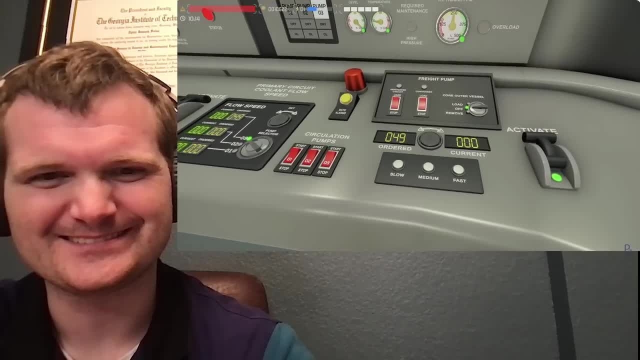 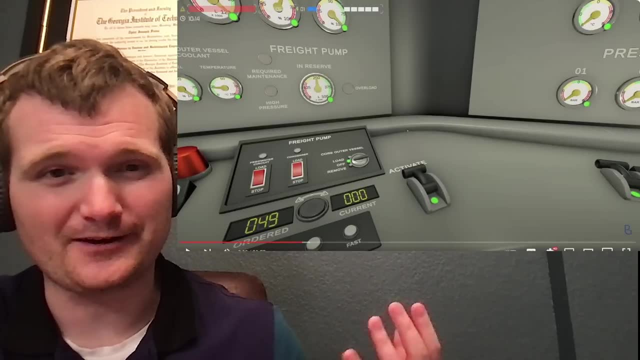 You must get a percentage, And this is something that people try to do is like just to kind of like almost get ahead of the game, But it really doesn't matter. So a lot of procedures are very specific about how you go up in both in terms of a plant. 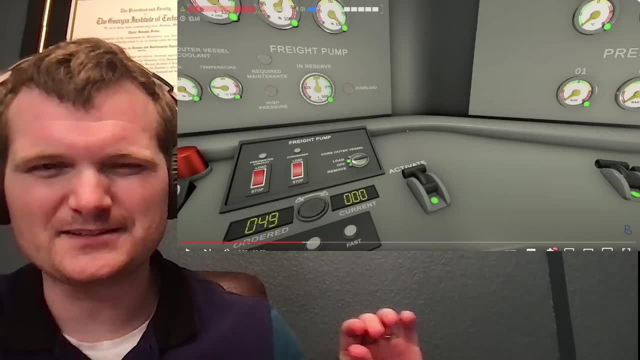 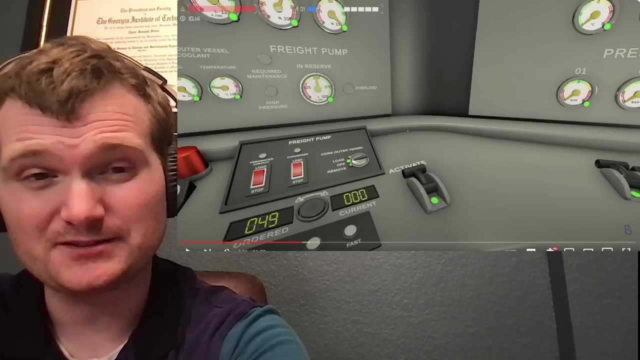 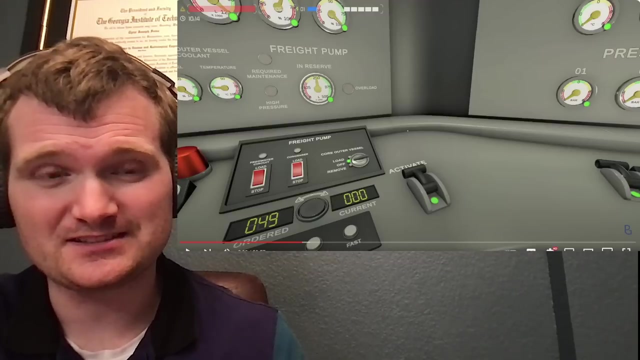 heat up and a plant startup and what things you put in the secondary plan at certain power levels. But at least in terms of the reactor cooling pumps they just had one speed And when you turn the first pump on You would actually see it would just go straight up to 100% coolant flow for that individual. 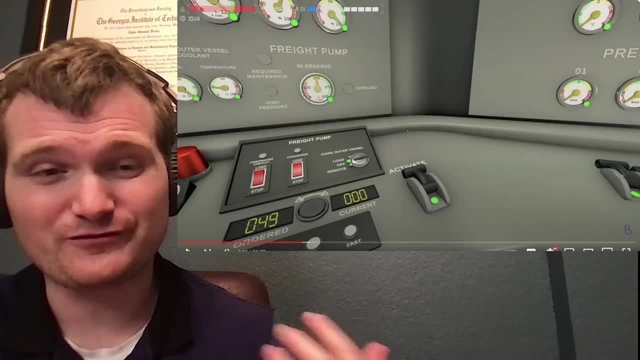 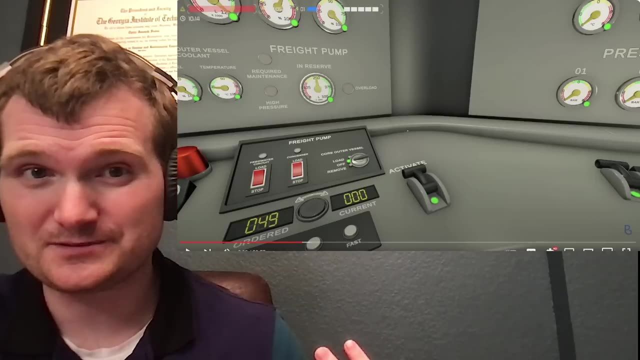 loop. Now what's interesting is, because it's all, it's four loops connected. you're actually going to have flow in the opposite direction at a much lower rate going through the other three loops. So I don't know if these other loops haven't been installed yet. 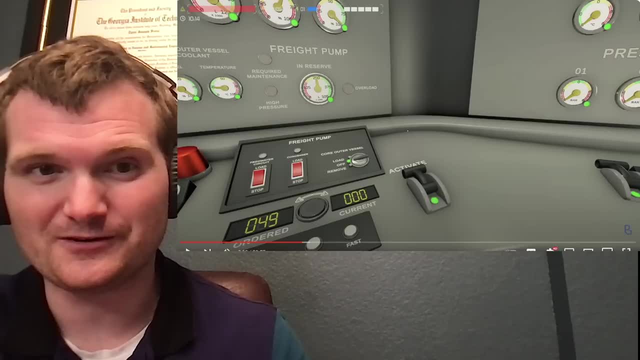 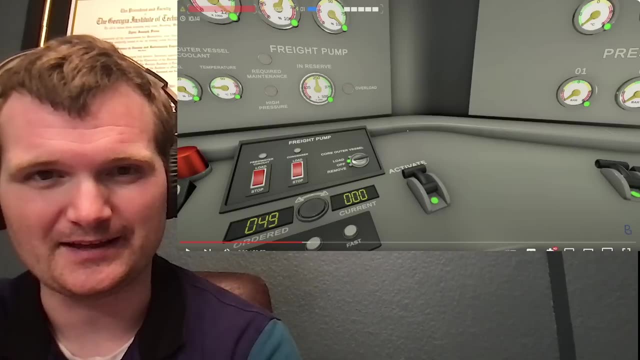 What you should see is, when you turn on a pump, it's going to cause flow in one of the loops and then backflow and the other loop or other two loops or however many loops this this plant has, But ours didn't have the ability to adjust speeds. 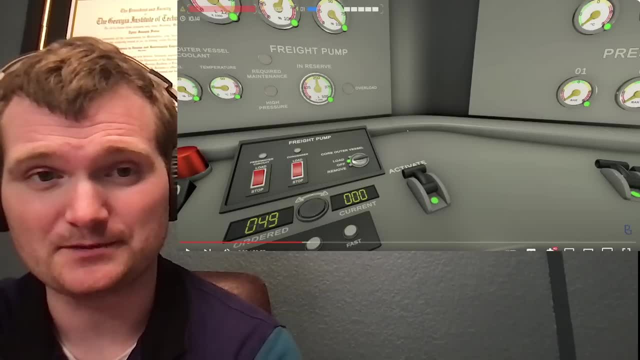 But that's not to say one couldn't be designed that way. I mean, I'm good with that. So we're going to go ahead and get that started. I'm just going to reach over there. set the speed, start circulating it now, because we 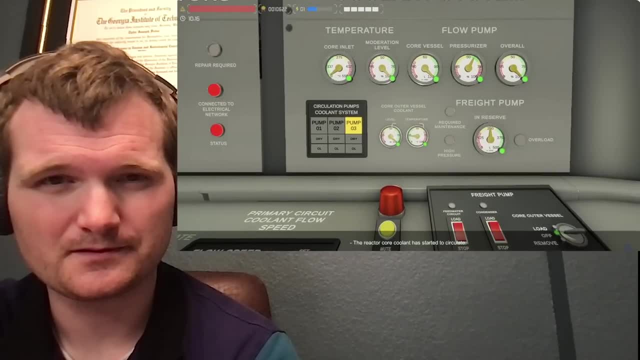 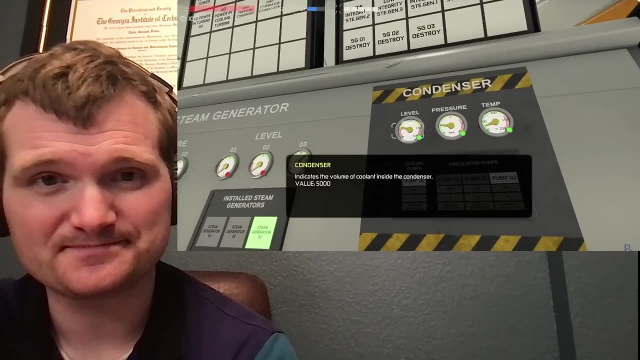 do want to get that circulating right away. Of course, as this is going, you're going to get a little warning on the bottom to say, hey, you're starting to move some coolant around. Is that intentional? The next thing we want to do is, if you come over, that's true, you want to see how it's. 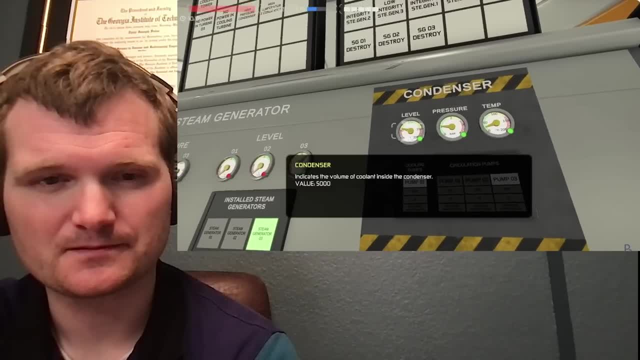 got a level. This level is very dangerously low. Once it starts turning into steam, You're going to get a little warning on the bottom to say, hey, you're starting to move steam, We're going to drop right off the bottom and then we're going to run into a problem. 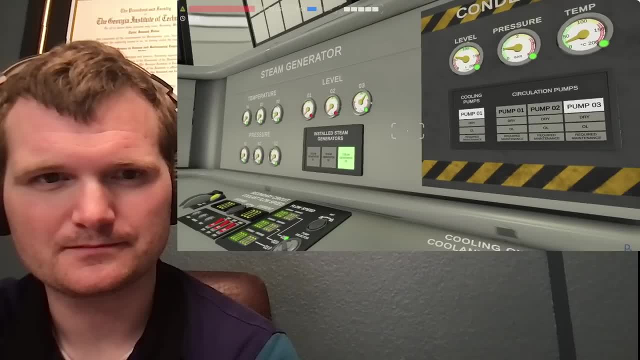 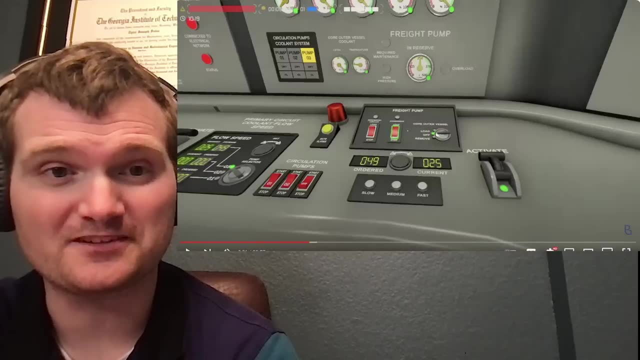 where you're going to get this fun little racing condition, where you're going to pop the breakers off. Don't do that. So instead we're going to. basically, you don't want your condenser to get too low because then the condensate pumps which feed the feedwater loop to continue that cycle going. would trip on low level because they wouldn't have enough suction to work properly. At least they should have an automatic trip function, like you said, Otherwise the pumps will just start to eat themselves because they don't have any water going into them. 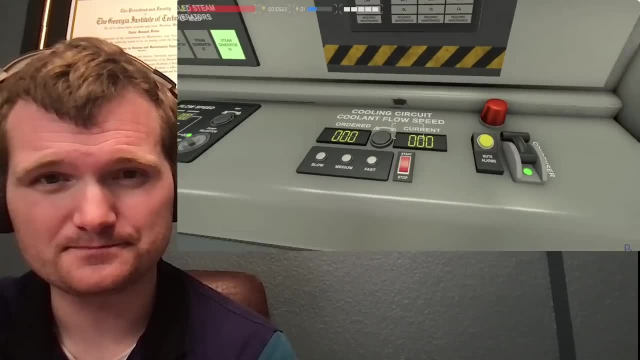 They're just going to come over here. We're going to hit load in the condenser and that's going to start flooding it up with some water. So while we do this- of course that's too fast, we'll do a medium speed here- 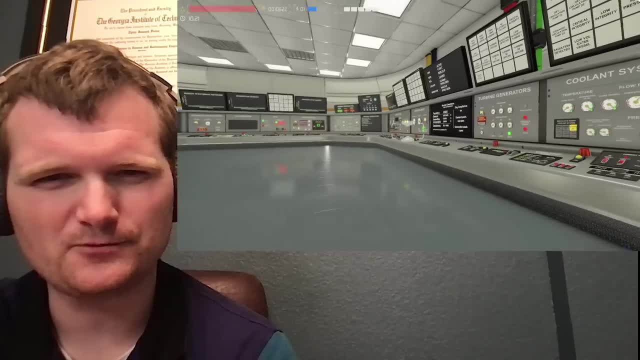 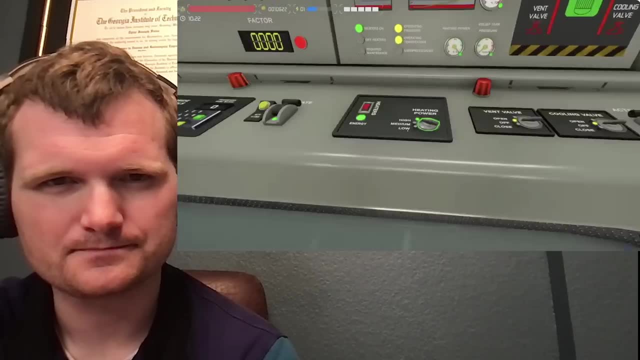 I'm just going to start circulating it. Remember, this is the thing that cools everything with adjustable speed. That's interesting, As we're starting to build that we'll start to do it. So we're starting to see that our vessel pressurizers are catching up pretty darn quick. 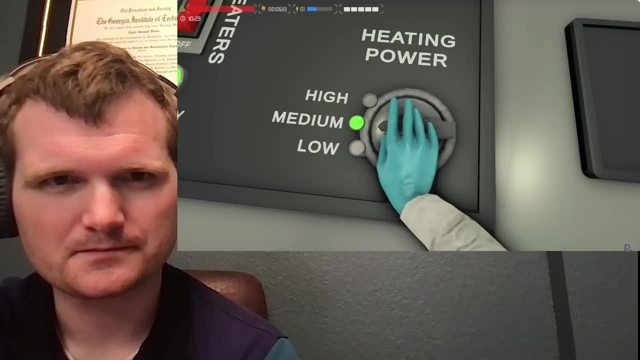 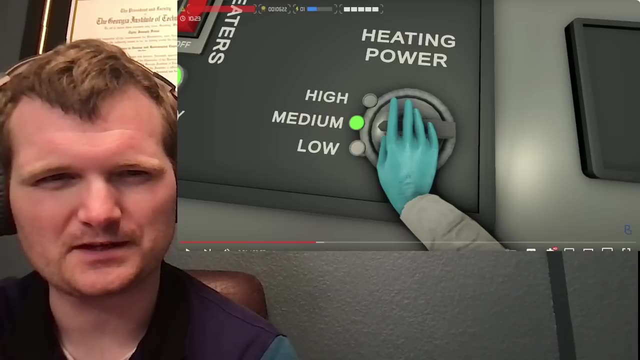 It's a good time, of course, to reduce my heating and temperature a little bit. Again, welcome to the control scheme here. This can be so awkward. Note Also: I don't know what this guy's wearing, but you wouldn't need to wear gloves to operate. 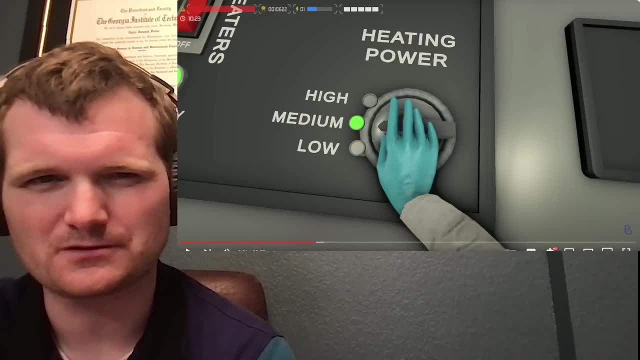 something And these look almost like surgical gloves in the control room, typically just bare handed. Now operating valves in the field or breakers in the field, you might need gloves, just cut resistant gloves or electrical safety gloves, but in a control room you don't really. 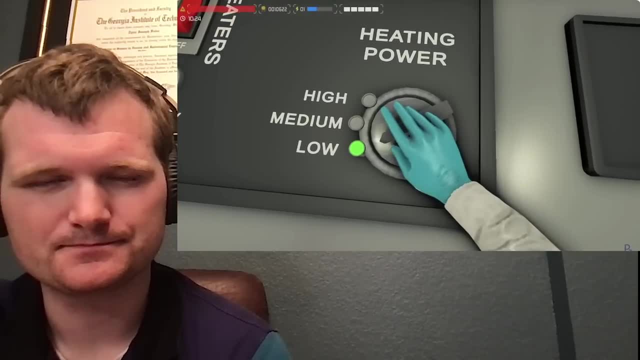 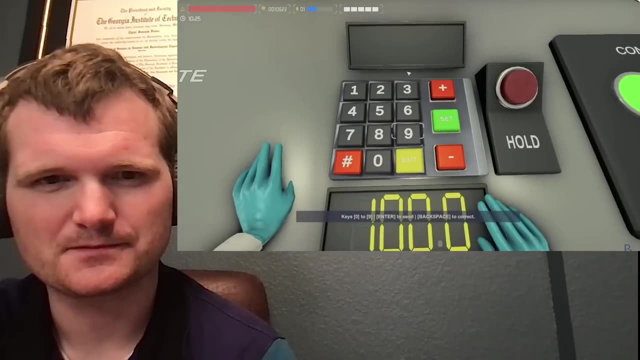 need to wear any PPE. Come on, This is so awkward. There we go. Perfect, That's going to start cooling itself down. So now we're ready to go ahead and pull some control rods and actually get this thing going. Now this controls the control rods. 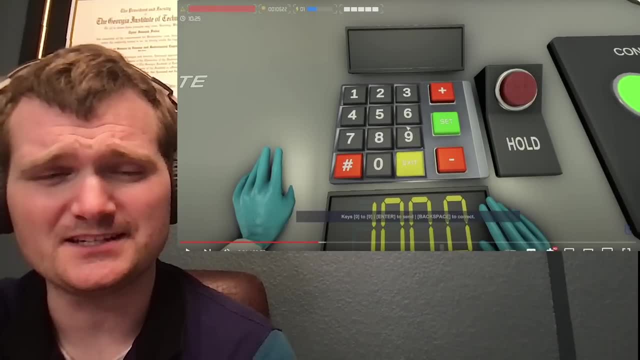 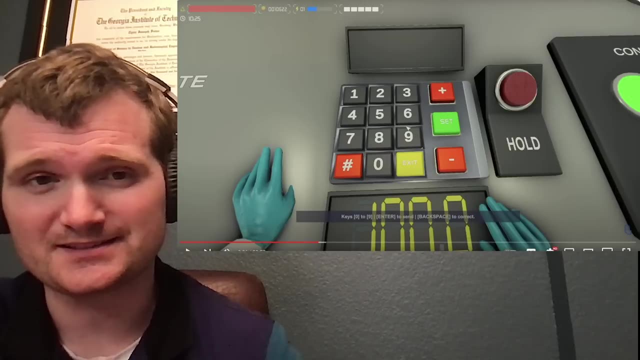 So we just skipped several steps. I don't know if he did some time compression Or not, but it can take several shifts to get the reactor both heated up and fully pressurized, and not to say many types of tests are done at each plateau in temperature and in pressure. 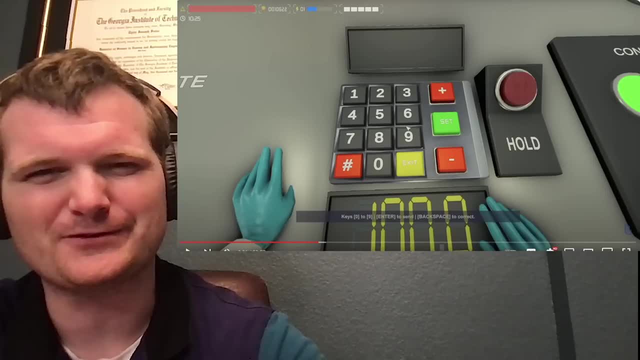 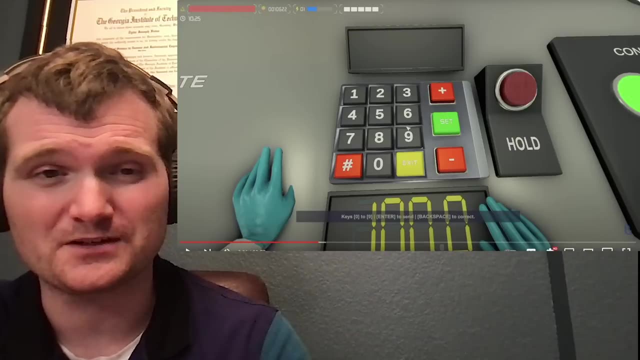 and power levels. So just keep all that in mind. but that wouldn't make for as good gameplay. So I can understand, you know. multiple shifts, time compression again to get us to the point where we actually want to start up. the reactor determines how much heat our core is going. 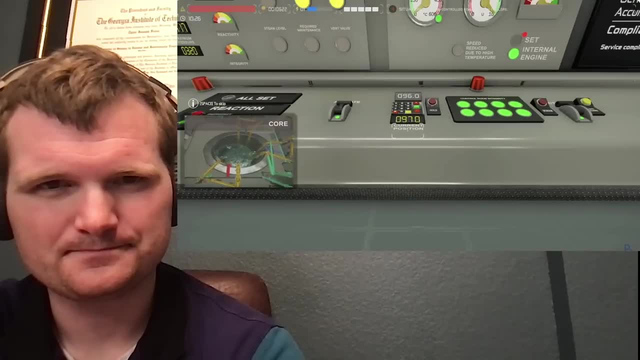 to produce. So if I set this to 96%, you can actually watch them. I'll show you a little video there that the control rods are going to slide up and they're going to allow the nuclear reaction to kick off, which is going to happen pretty much. 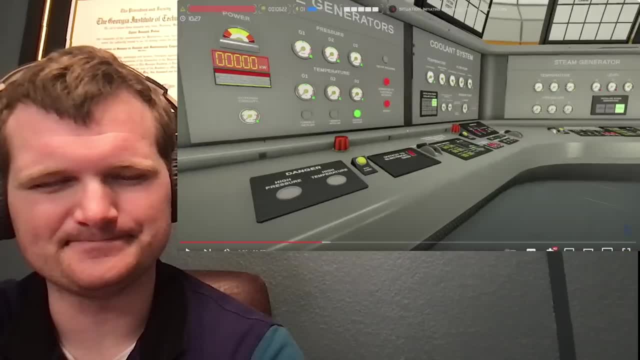 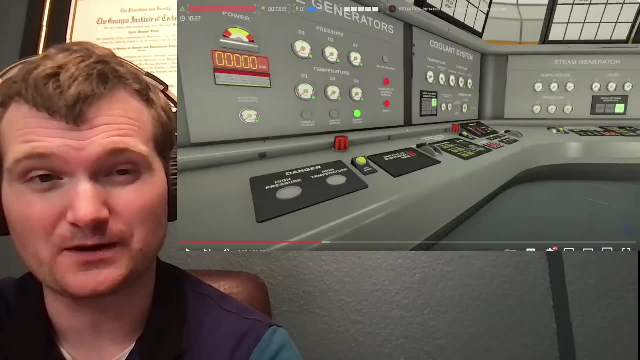 right away And you can see how this starts to heat up. No, you wouldn't. it wouldn't kick off right away because there are so, there's so much margin built into the control rod system and nuclear power plant in real life that it can. 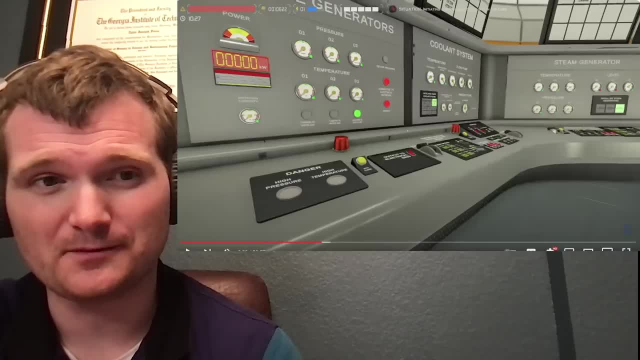 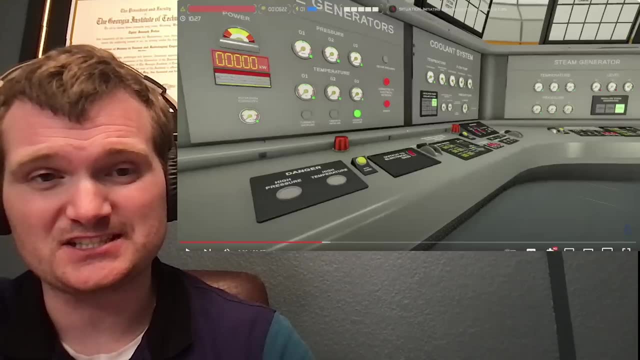 take a while to get the reactor to start up, because you have what's known as shut down banks, which which is known as shut down rods, which will keep the reactor running- Yeah, Yeah, It's going to keep you shut down- which are way more than you need to shut down. 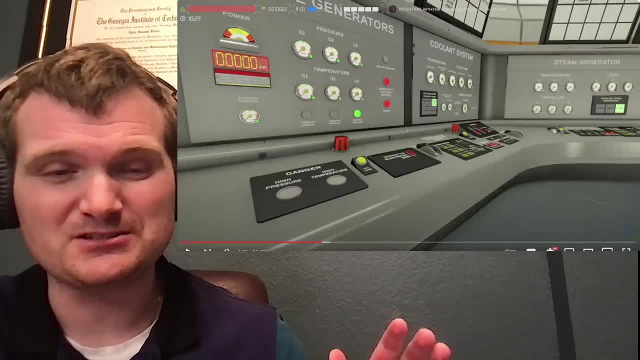 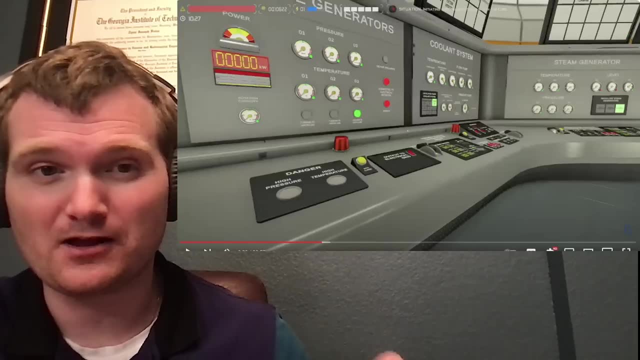 So you can pull all of the shutdown rods which, depending on the on the reactor design, can be half of the control rods in there. pull them all fully out. Reactors still shut down Now an operator. operators are trained to be ready to anticipate um criticality or the 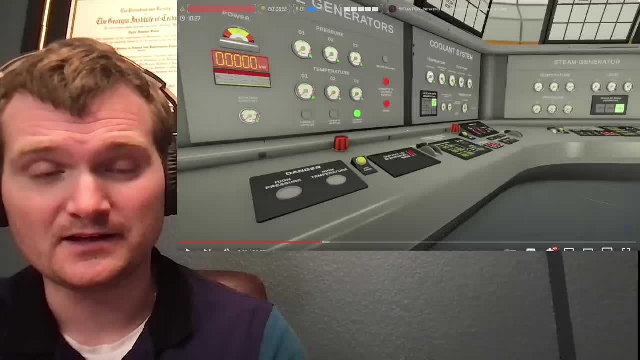 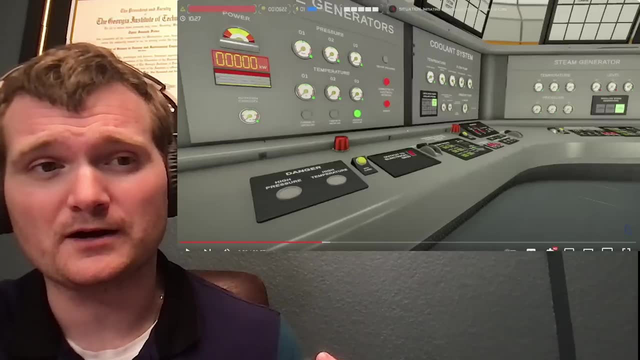 moment where the reactor is on and creating a self-sustaining vision reaction at any time, but you'd never see it just from pulling the shutdown rods. And then you get to the end. You get to the control rods and this is a heavily oversaw, regulated process. 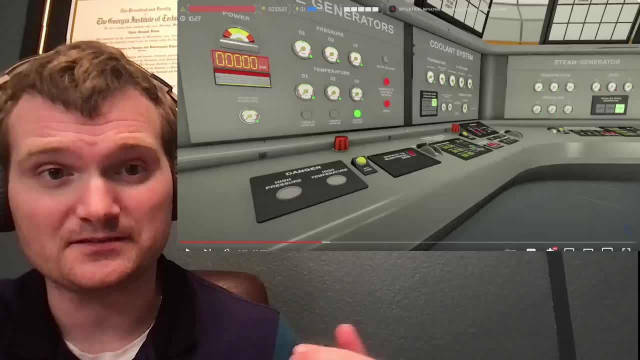 Even have reactor engineering specialists in there to assist you And it would be long briefings, calculations, analyses to tell you around when you would expect to be uh, to take the unit critical And yeah, so this is B, this is another long process. 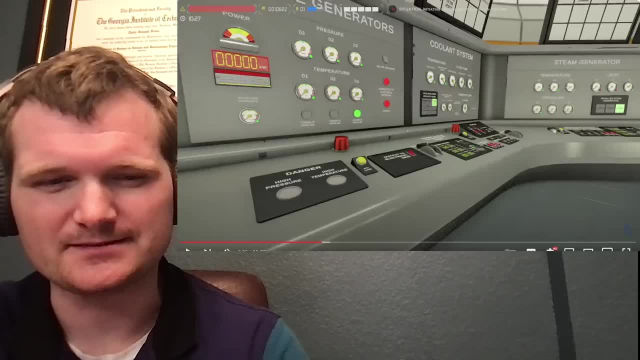 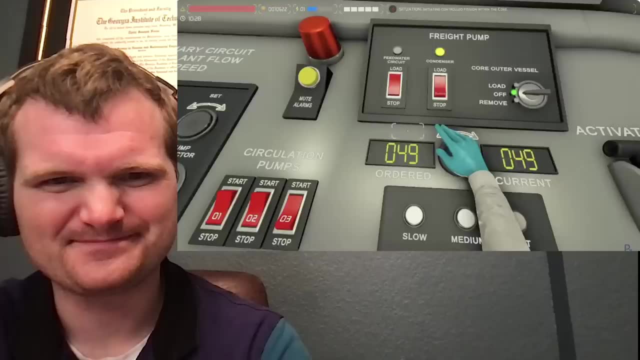 Now, this wouldn't take, this shouldn't take multiple shifts, but it's. there's a lot more. there's a lot more going on there, Yeah, Immediately. So I think we've got plenty of water right now. I'm actually gonna shut this off and you can see right over here how we're just starting. 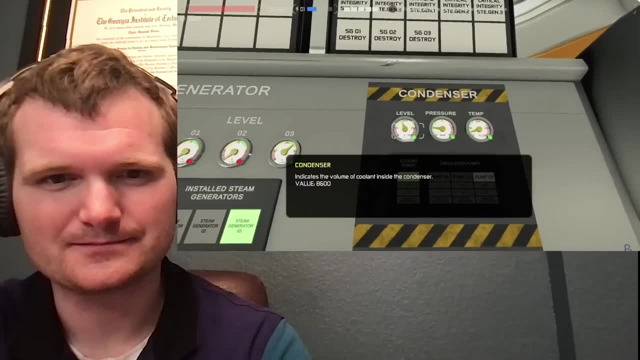 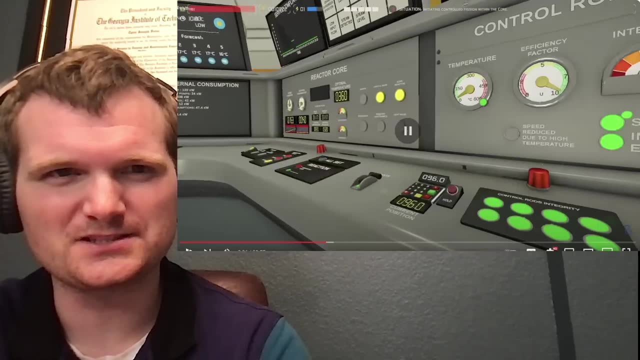 to kind of crash up here towards that 100 level. Uh, keep in mind, this thing will kind of balance itself out. as long as you get really close to a hundred, you really shouldn't have too much trouble here. So what's happening now? I usually see level as percent, but it could just be the height. 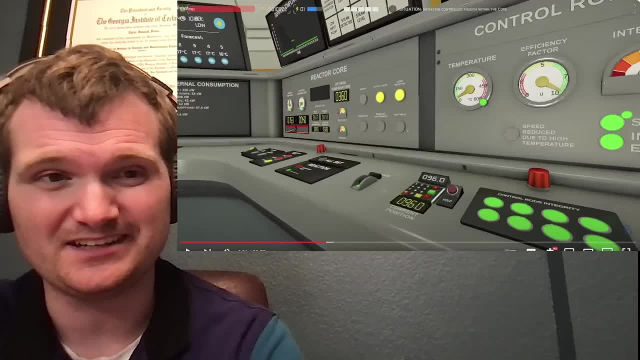 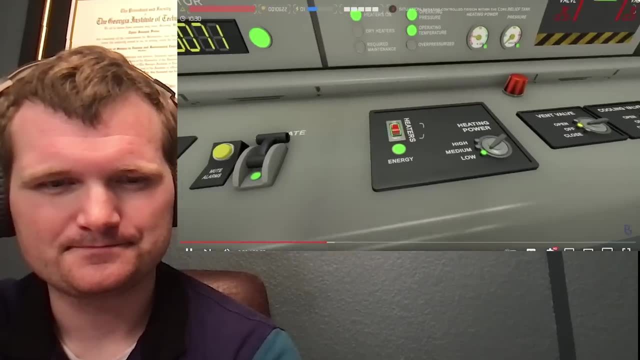 of the tank or or the condenser. What have you seen it in? you know feet, meters, centimeters, whichever is. I can see that are we're totally warmed up on the pressurizer. Let's go ahead and pop that off real quick. 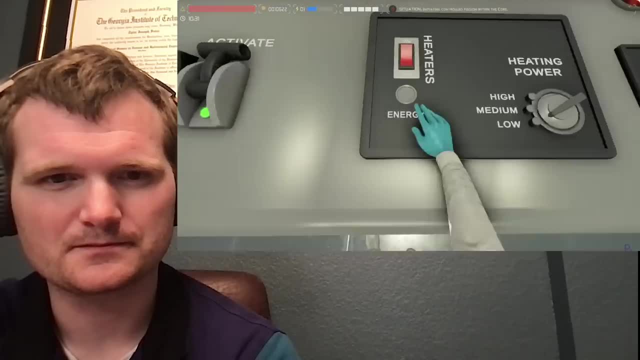 And again one 60, and you know we'll let it run a little longer here. One 60 is kind of the sweet spot, but you're gonna be playing with it and you can see my main reactor. I'm not seeing real fast. 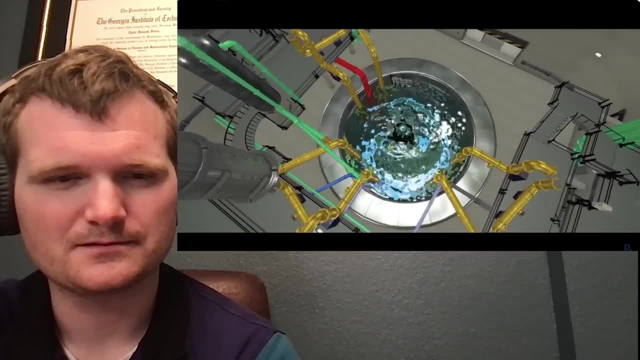 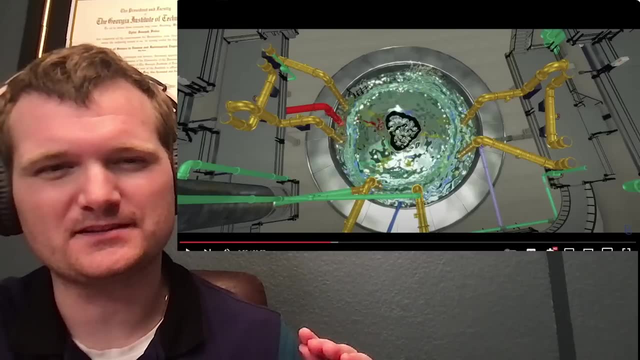 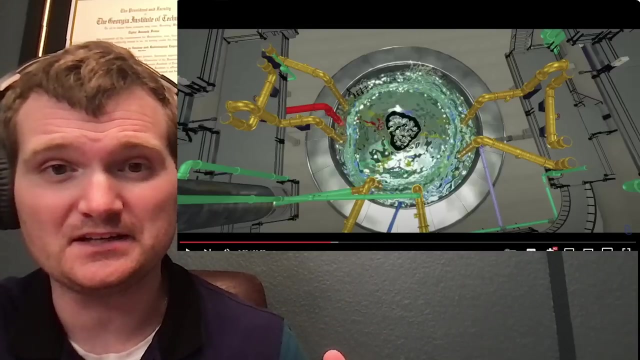 Units. This is fun to watch. Okay, I think I can tell what they're basing this on. They're basing this on like tests that you see in labs or um universities for those type of reactors. You're never going to see one pulse in real life for a full size commercial nuclear reactor. 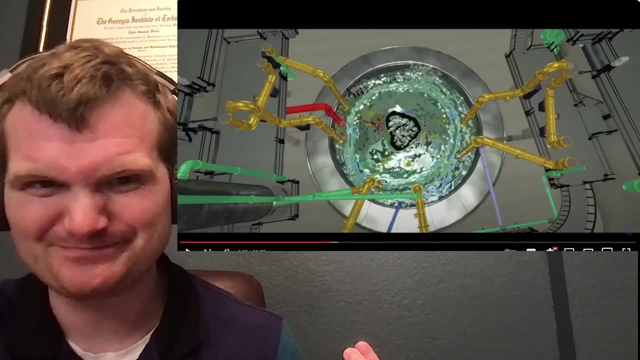 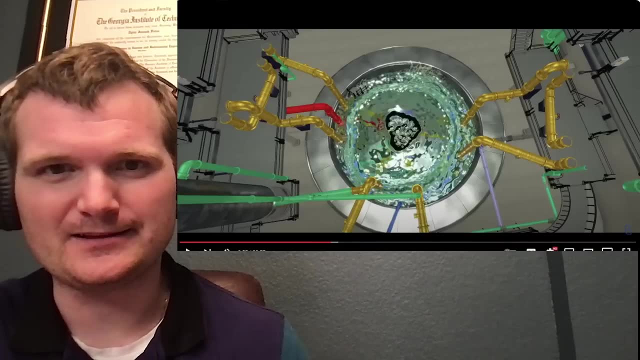 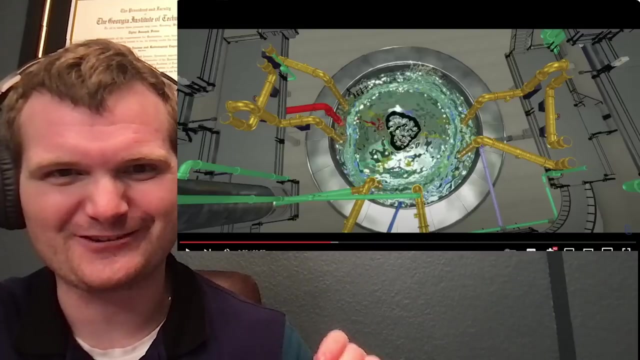 that produces a thousand megawatts. No, such a such a thing you'd you would never see that. that happening now. And I know this isn't supposed to be one of those, because they said pressurized water reactor, So, but it looks like they got the reactor vessel in a water tube. and if it was really 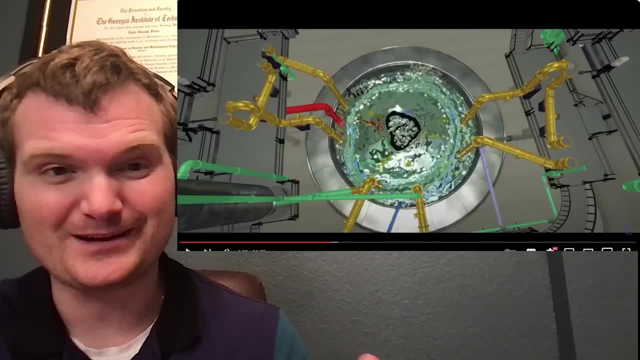 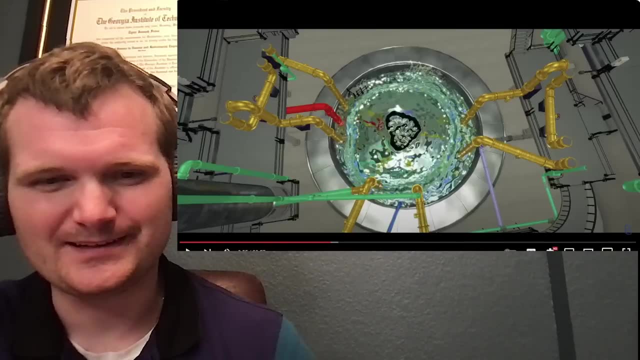 pressurized, you wouldn't see any flash or anything, because the vessel would keep anything secured, even if you were to uh somehow create those sort of uh pulsing conditions. But yeah, this is uh quite, this is quite inaccurate. 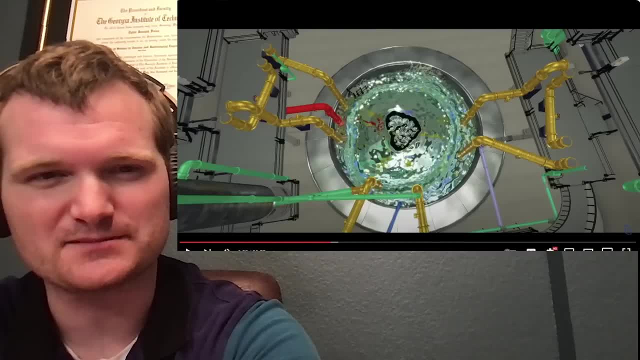 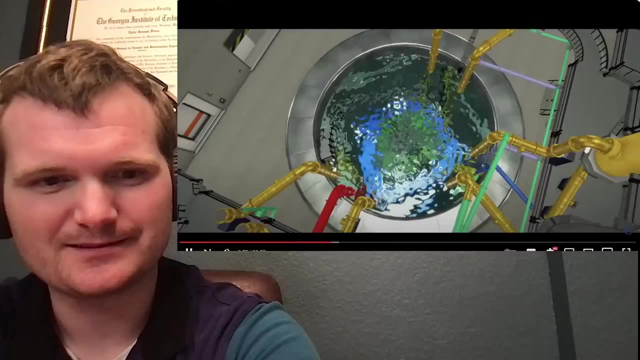 I can tell they've. I can tell whoever designed this got got inspired from some of the trigger pulse pulse reactors though. So there you have it. It's real fun If you want to have some, that's the reactor going critical there, by the way, that doesn't. 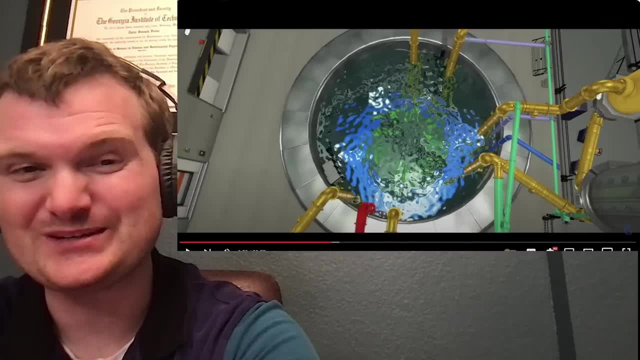 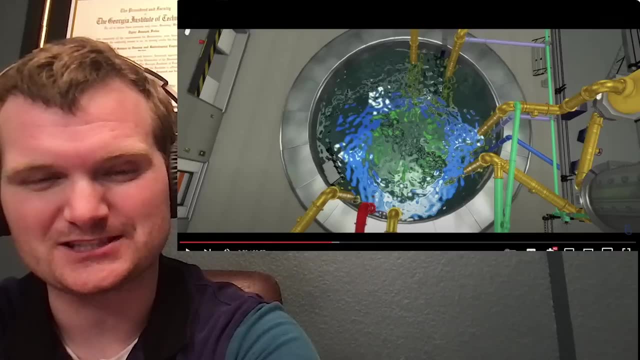 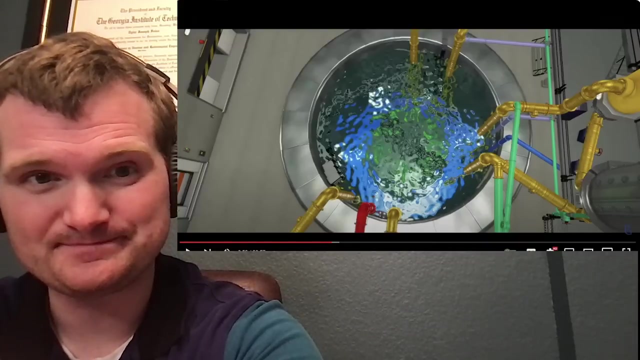 mean It's going to be going prompt, critical, which is what you would never want to see, because that was when the reactor goes from milliwatts to megawatts in a fraction of a second. Again based on fuel design, fuel loading, control, rod position, um. enrichment of the. 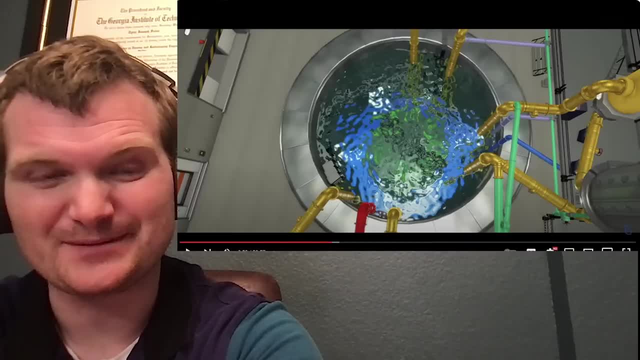 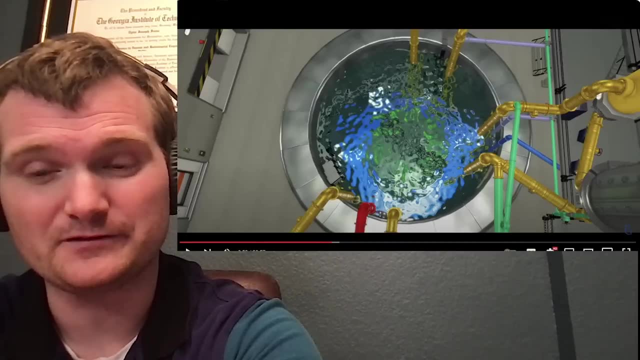 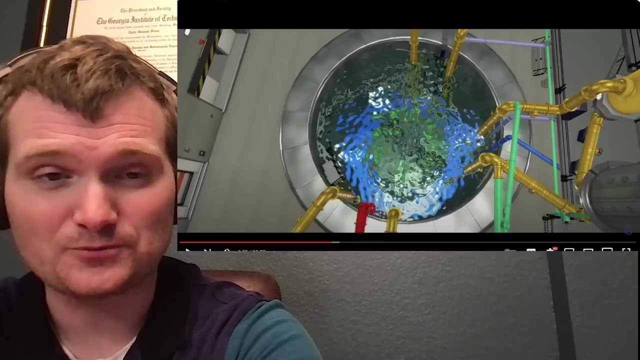 fuel and how it's placed in there. You would never see something like this, Not even at Chernobyl. Chernobyl put themselves into a condition like that, but that was because of Multiple Um param design parameters were exceeded and ignored, as well as from multiple different. 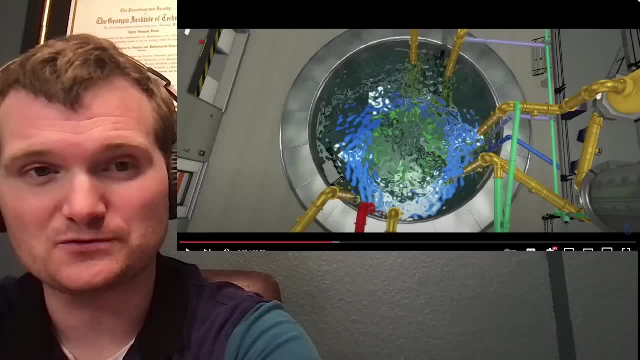 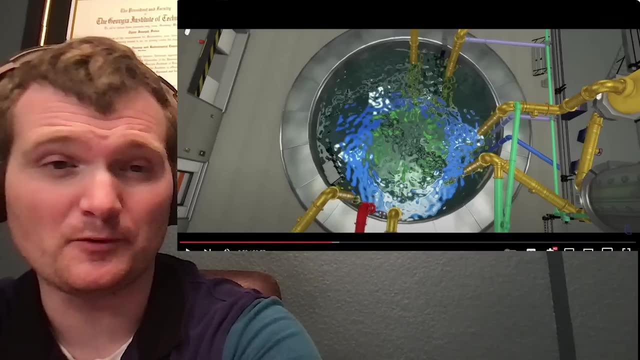 angles. I'll pin a comment with a more detailed review of what all happened there, but you would never see this in a pressurized water reactor. Chernobyl was not a pressurized water reactor, by the way, it was a it's. it was a weird. 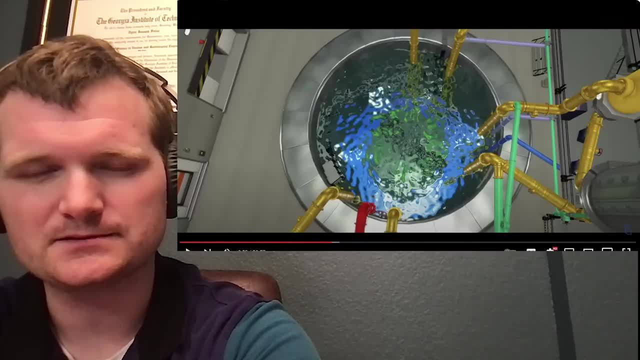 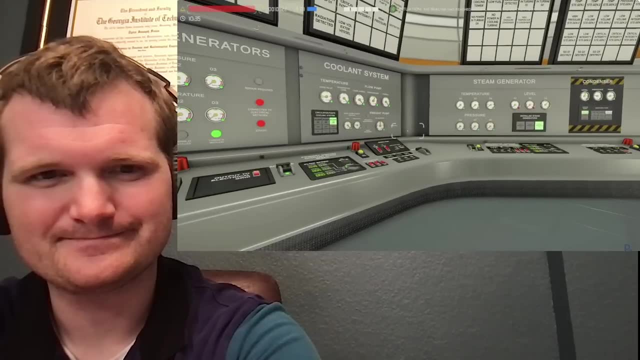 type of boiling water reactor known as an RBMK boom. That just means we're warming up, kind of a thing like that. And uh, we now have, We now have a reactive reactor. It just reacts. It's overreacting all the time. 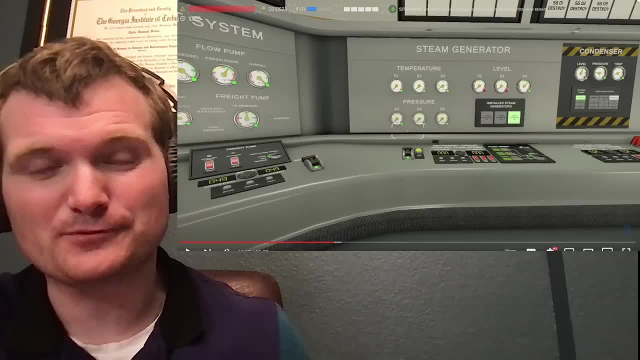 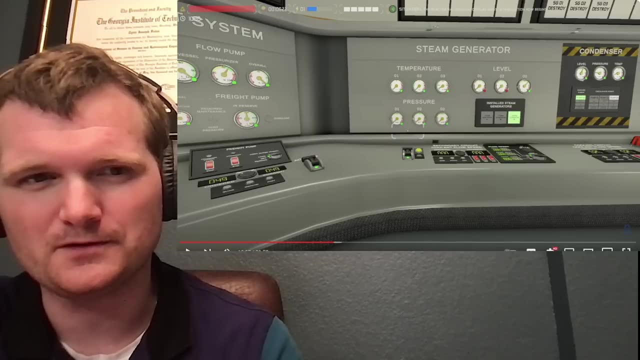 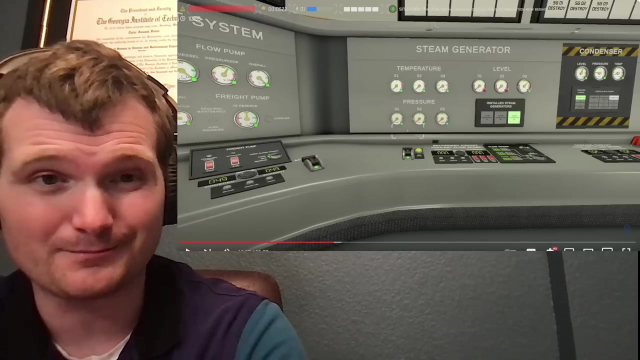 Now And if, if anything before, you'd even approach something like that, the reactor would shut itself down. even a slight, um, a slight overpower, The reactor would shut itself down. The control rods would fall in the reactor, Trip breakers would open and the control rods would fall in and hit the bottom in less than. 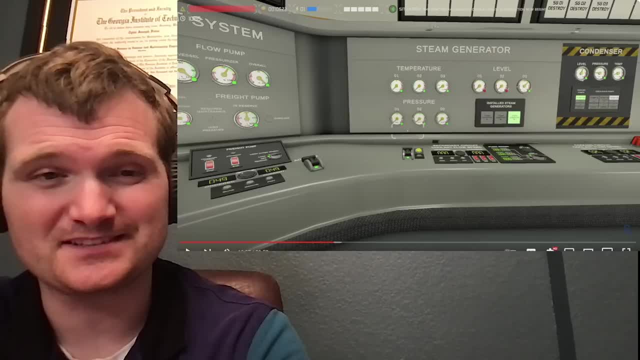 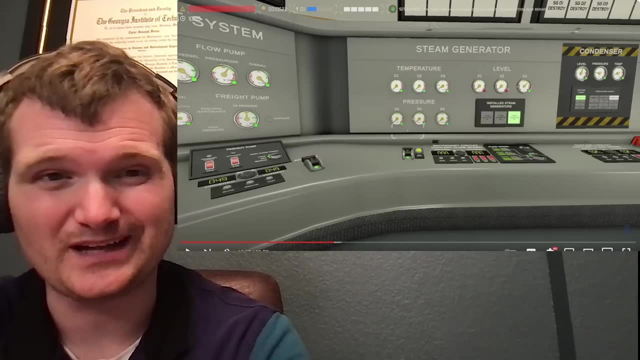 a couple of seconds, And especially in a pressurized water reactor. that system is highly robust. Um, basically, Basically, gravity would have to fail for the reactor protection system to not work. Oh, the cool thing here is, of course, uh, now that they're starting to produce some. 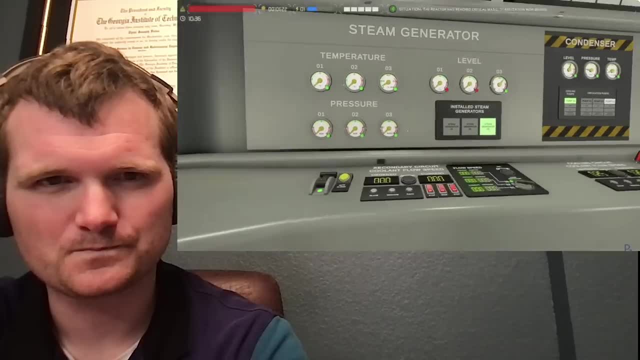 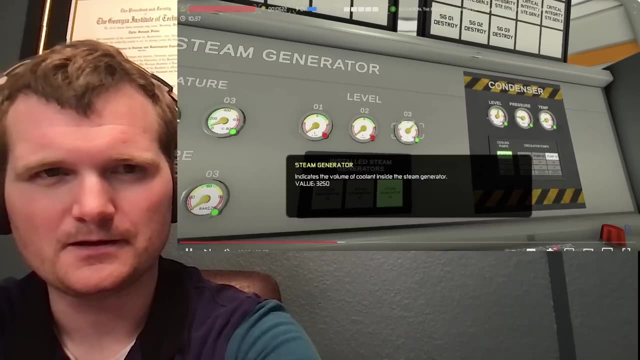 heat. here you're going to start causing some steam to be generated. Now, this thing is basically responsible for that. The most important value we have in this entire panel is this guy right here, which There's a one. there's a milestone called the point of adding heat, and heat is generated. 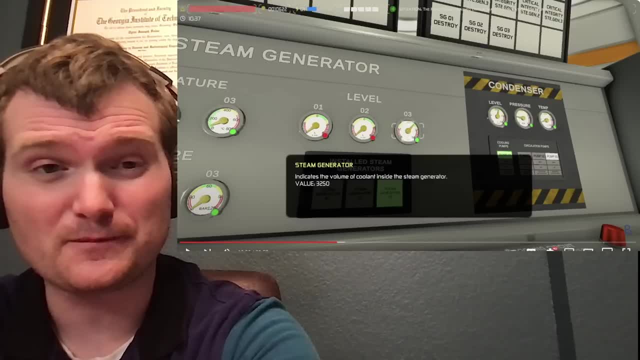 just from decay, heat from the pressurizer heaters, heat from the reactor coolant pumps. But when you get around 1% power, that's when you the heat is actually coming from the fission. I have no idea what power they're at the whole prompt critical thing. 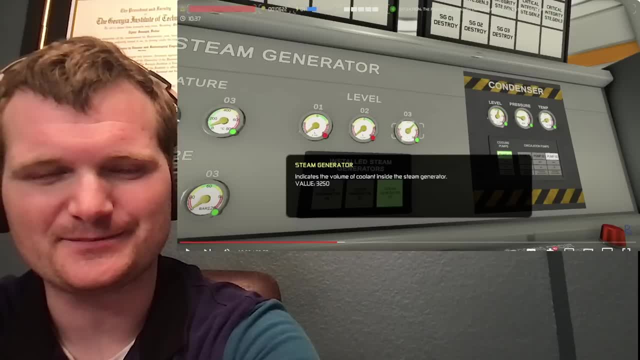 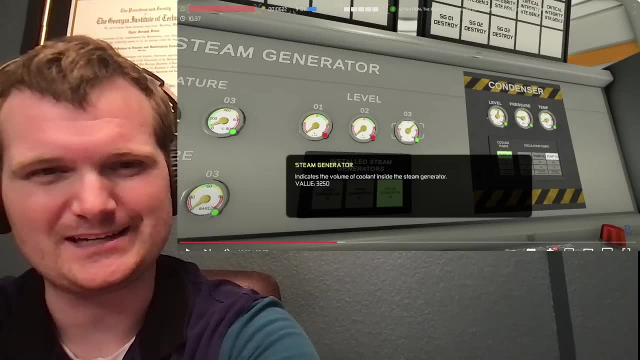 That means they were, they were in the megawatt range and then it shut themselves down a bit. If there is what would have happened, it would have been like a start and a shutdown If it happened to anything like those, uh, those pulse reactors. but here we're entering. 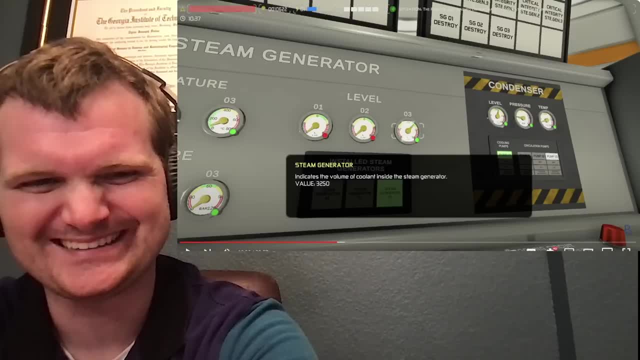 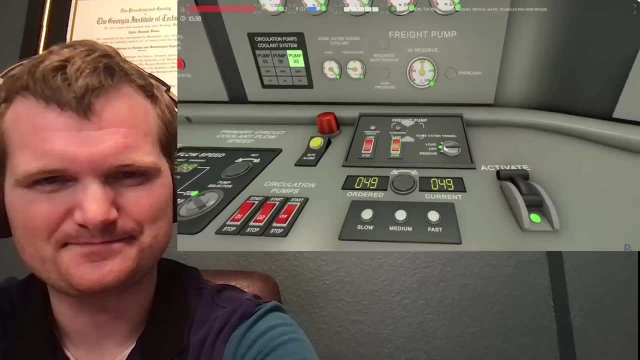 in uncharted and unrealistic territory. It means the amount of water- Yeah, That's cool And they're calling it here. That's inside the steam generator. As we produce more heat And as we start to increase the flow of heat we have to use- basically manipulate this knob. 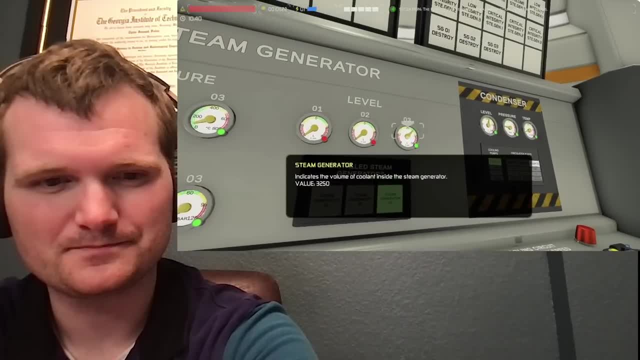 for the purposes of controlling the amount of steam we're generating. Now, if this value starts to get too high, we have no room for steam. You're going to trip the generator. If you allow this to get too low because you weren't keeping up with it, what's going? to happen is you'll trip the generator Again. not necessarily the case. There is a steam dump or a turbine bypass valve, which would basically Sten Sten instead of going to the turbine. there would just be a line that sends it straight. 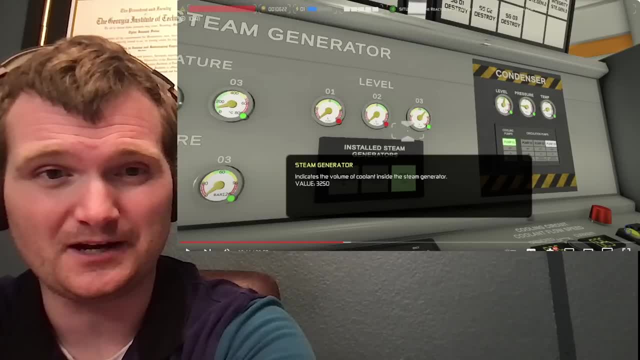 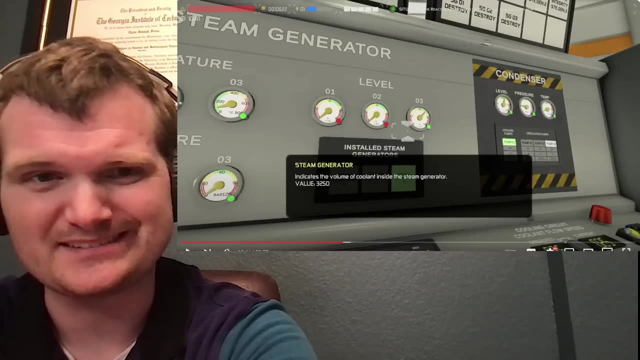 to the condenser: Um, it's not uncommon to have those valves um open to an extent while you're, while you're starting up, And now it's a very control and it's a very controlled process, Unlike what you saw with the uh prompt critical thing. but I've never heard of a situation. 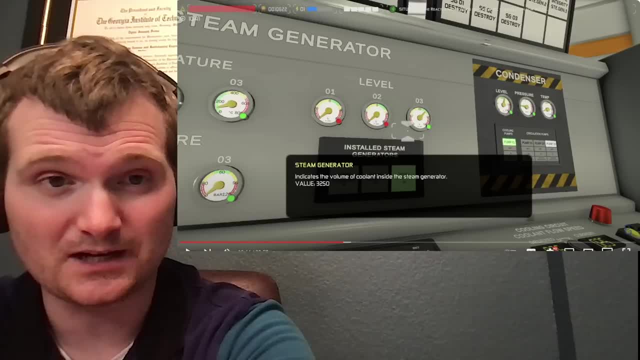 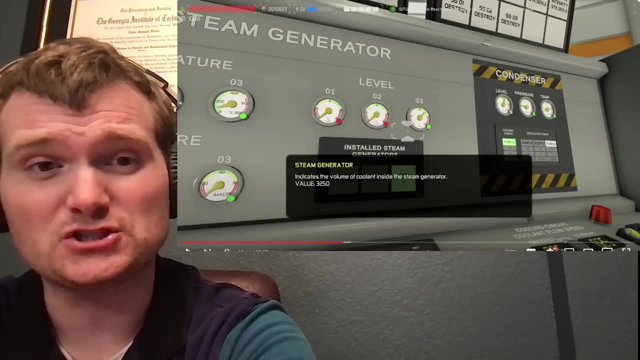 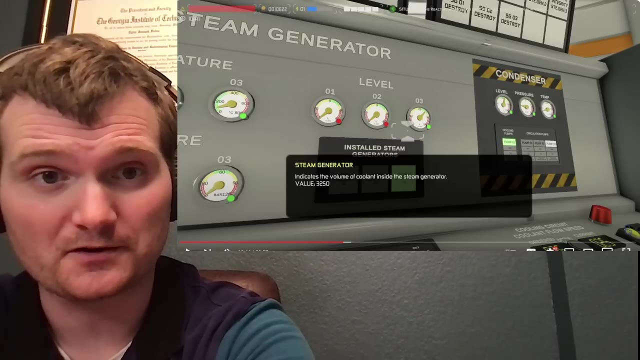 where excessive steam demand um by itself resulted in a generator trip. Now, What steam demand will do, was it? will It actually Drive reactor power? There's a saying that um reactor power follows steam demand in pressurized water reactors. 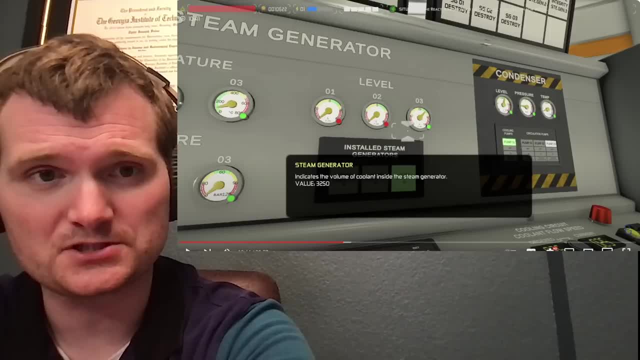 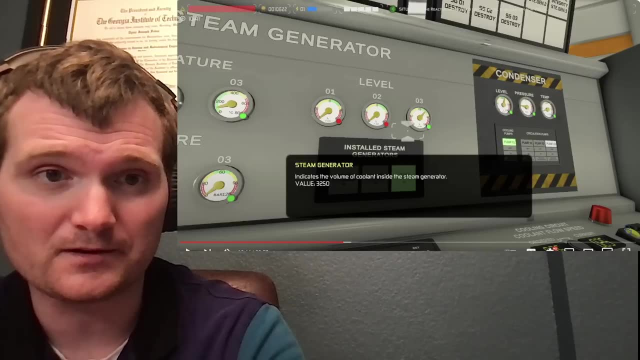 because raised steam flow will lower temp temperature. lowering temperature will actually increase reactor power And then they'll reach another equilibrium state at a higher power level. And the main reason when you do that- and typically when you do that, if you just add: 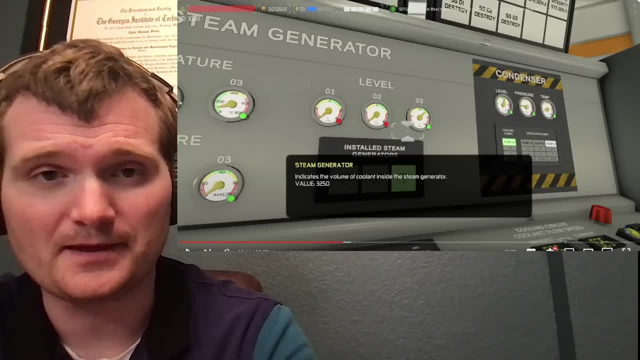 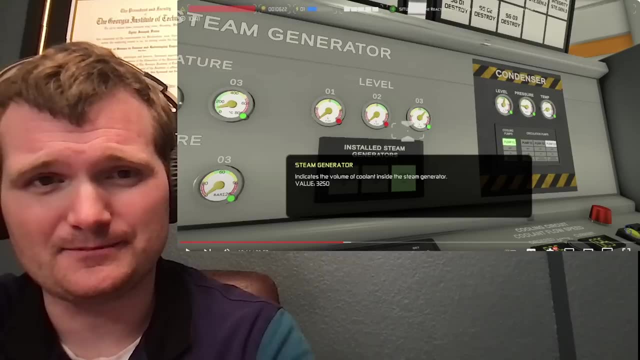 load to the uh, to the generator, and that will uh cause that system to occur. that will also happen If you see a steam leak, though, But if you haven't any, um off normal procedure where you have an excessive steam demand. 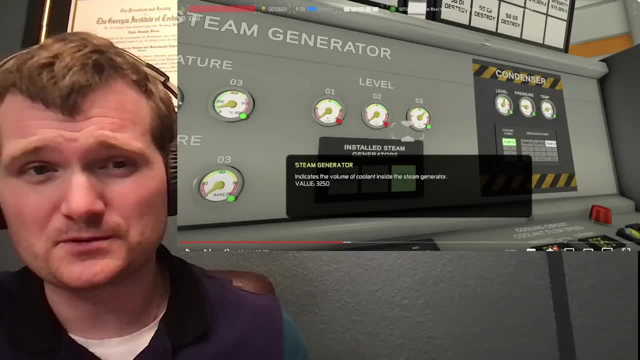 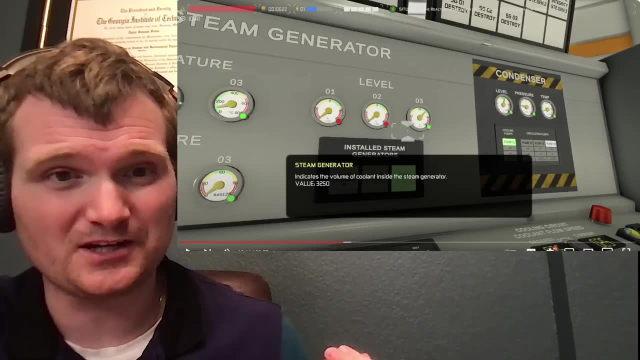 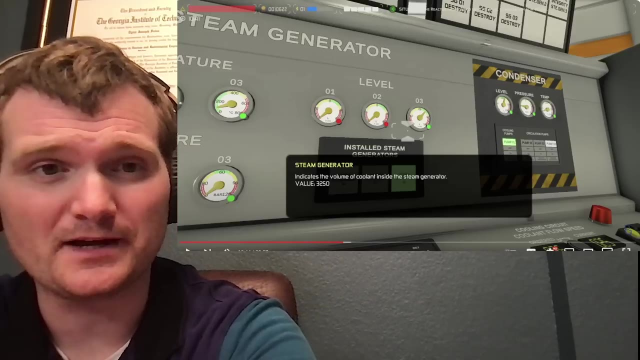 you would actually end up shutting down the reactor. If, again, if the reactor protection system doesn't shut down itself and it would be on low pressure cause, lowering temperature is going to lower pressure in the primary uh the reactor systems and then it's gonna gonna shut itself down, or then the reactor 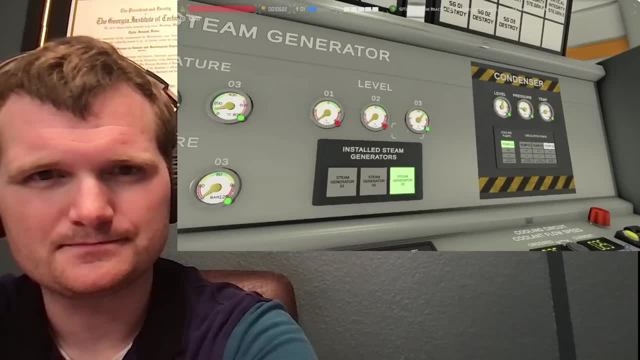 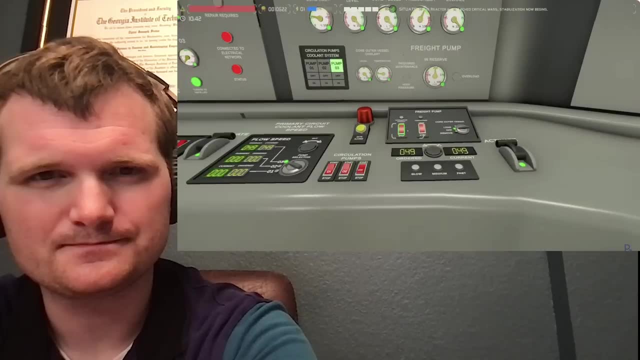 protection system would engage, Cause your steam pressure will basically drop, Yeah, And it's gonna pull off. This little gauge right here is basically your magic thing to tell you what amount of speed we need on this, which, of course, is indicative of how much heat you're pulling. 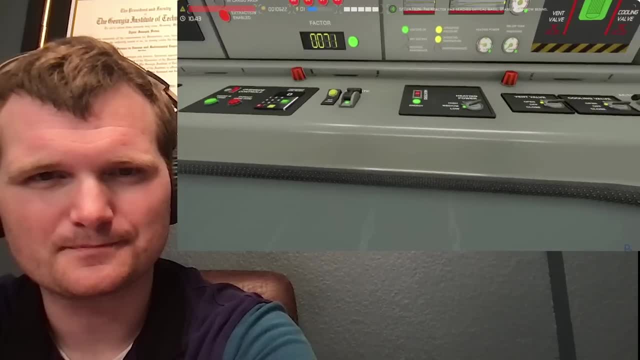 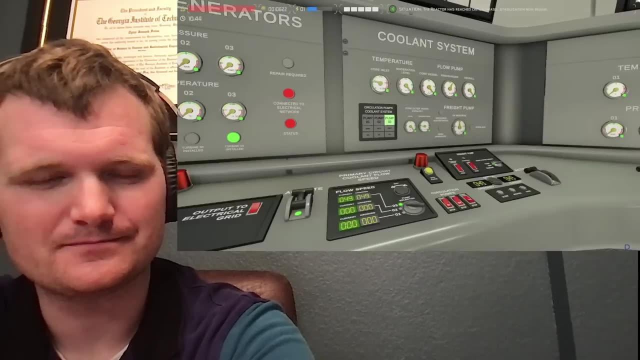 off the reactor itself. So if you flip back over here you can see, uh, we're getting real, real high with the pressurizer. I'm gonna shut this off. We don't need that to be that high. And my reactor itself is overboiling, uh, which now means that's a good sign. 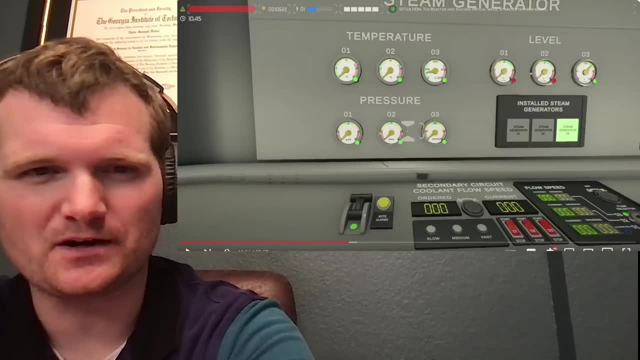 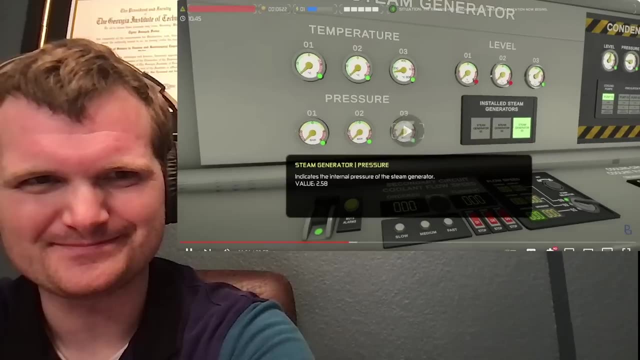 And we're gonna start Boiling of anything in a pressurized water reactor is never a good sign. If this was a boiling water reactor, then sure, But no, just no Pressure. As a matter of fact, if I hold my mouse right here, do you see how pressure is starting? 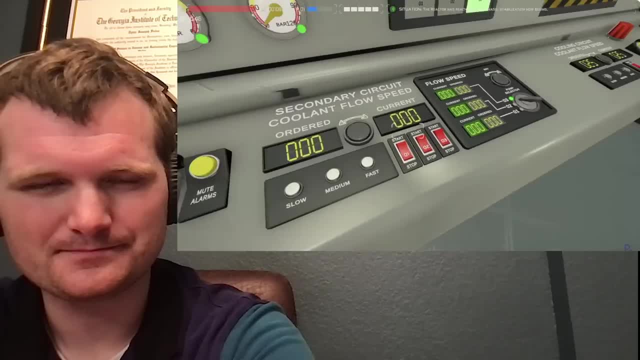 to be generated, but also notice that this is starting to creep downwards. So what I'm gonna do is I'm gonna go ahead and slam that to slow and we're gonna go ahead and start it up. So what this is going to start doing now is it's going to be start pulling, basically water. 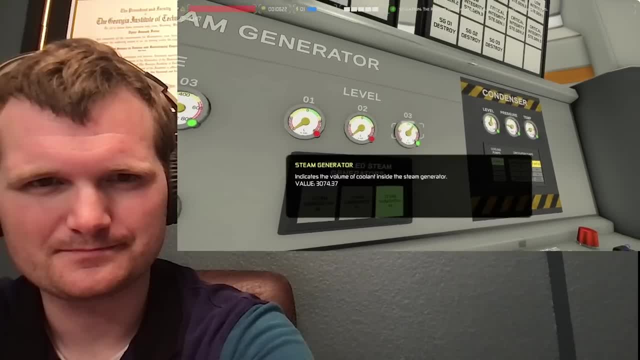 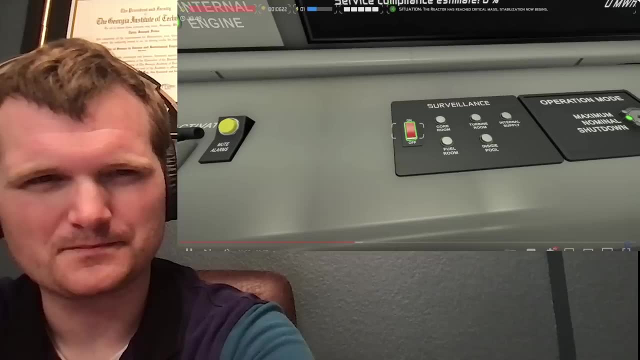 out of this side of things, shoving it in here, boiling it off, and then it's gonna take what's boiled off and it's gonna send it over to our buddy, the turbine generator. Now the turbine generator itself is not going to be moving very fast. 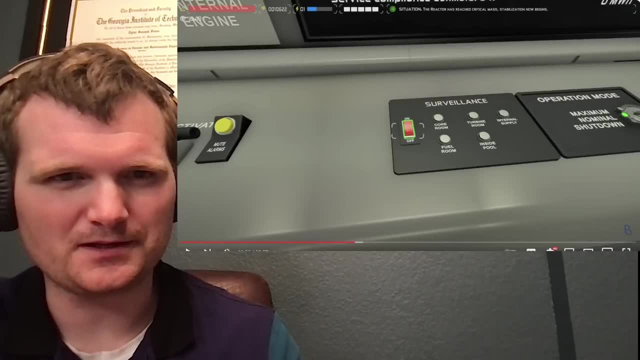 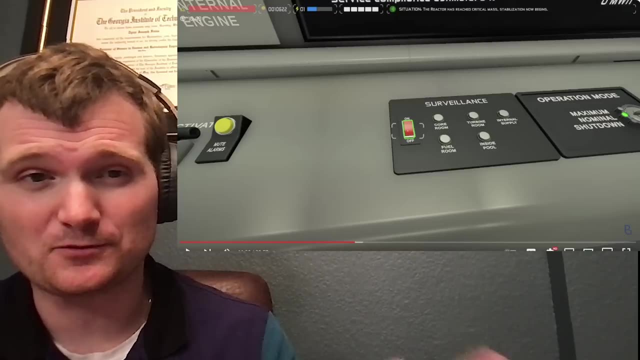 Interesting that you have to go to that and then go back over to the turbine generator. Yeah, So the turbine generator panel- usually things are- the control panels are almost in order where the turbine generator would be on the right side- Again, a minor thing, but there is some ergonomics to be taken into consideration especially. 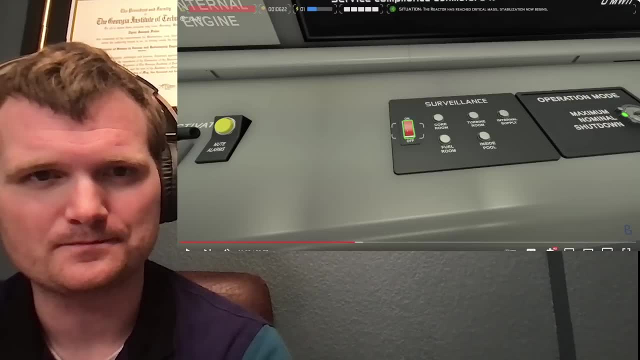 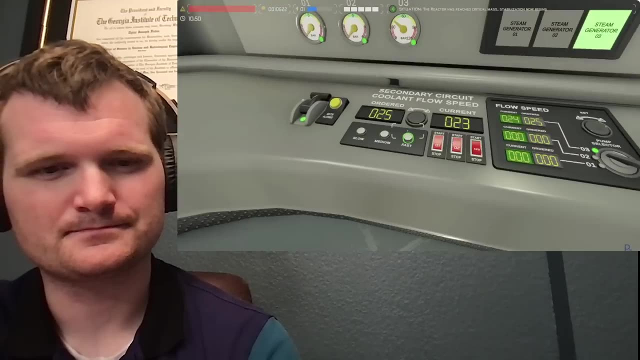 when you have a limited number of reactor operators to work with And you'll see this thing barely starting to spin up in a few moments here, And when that starts to do that, we're actually producing some power here. Now notice here that I'm starting to get very low on the clip means the speed here is too. 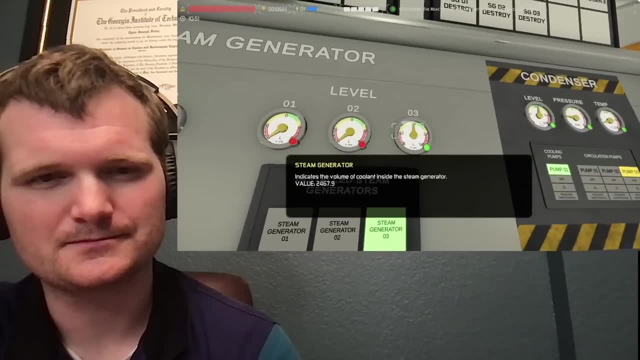 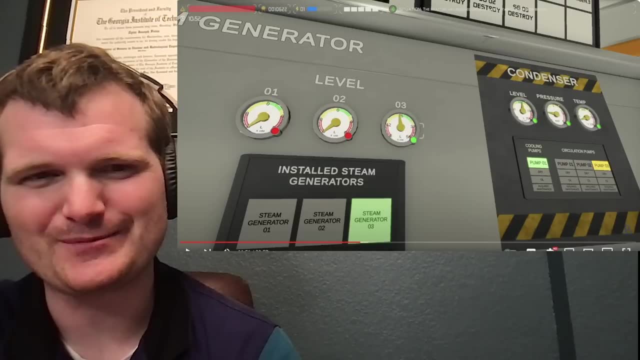 low, So I'm gonna crank this up to about 40.. And what you're gonna see is you're gonna see this needle come down as we boil all that steam and then it's gonna start shifting back up On the note of these controllers. so a lot of these you don't have to operate. 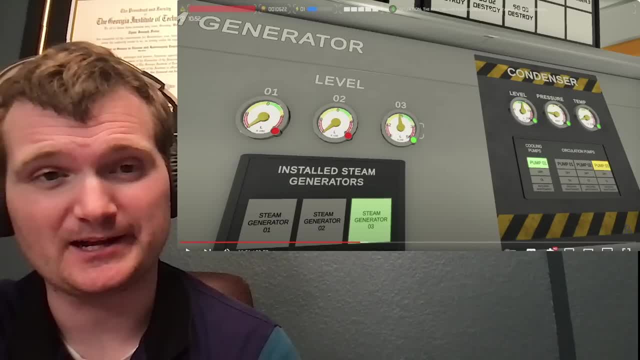 them manually, like the speeds and like the steam flows, and like how fast the pumps are going. Well, the pumps, well, it wouldn't be the pump speed, but it would be the valve, It would be a valve position to tell you how much flow is actually going back into feed. 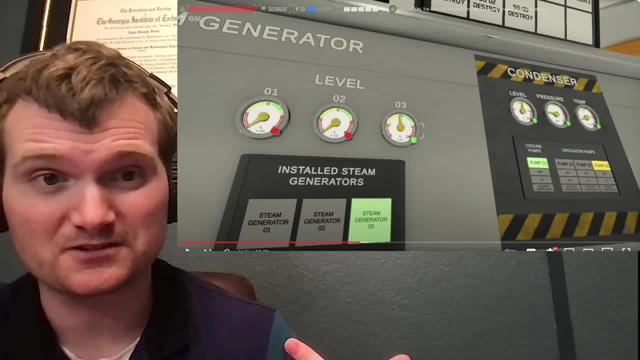 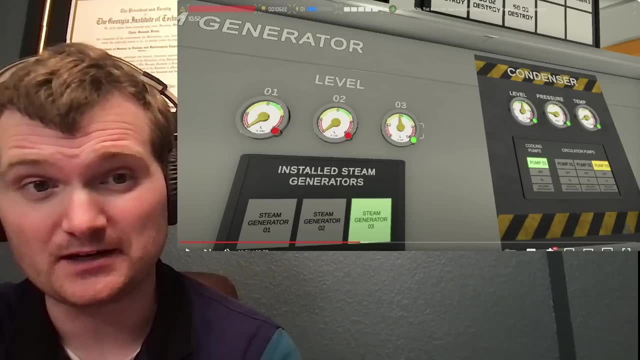 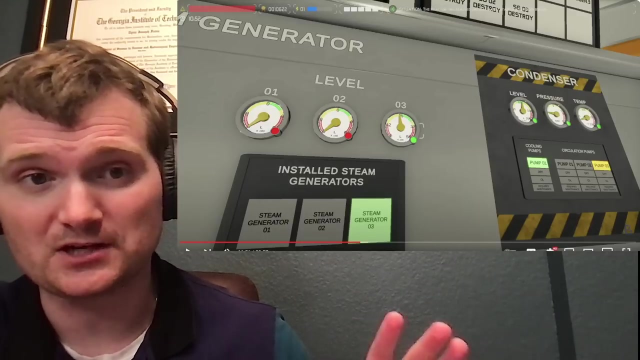 water versus how much flow is just gonna be on recirculation. A lot of these would be an automatic, So you don't necessarily have to babysit the controllers as much Now. you would still monitor and verify they respond properly in automatic And if something does malfunction you know the operator would need to take manual control. 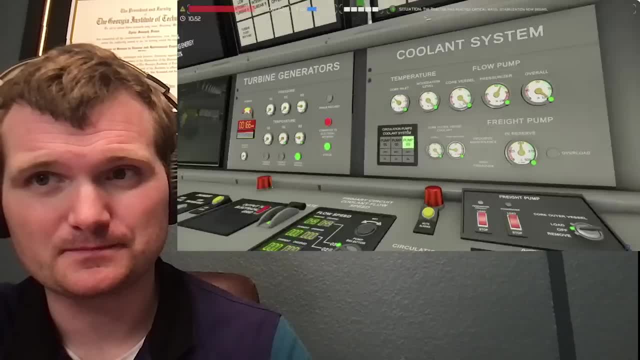 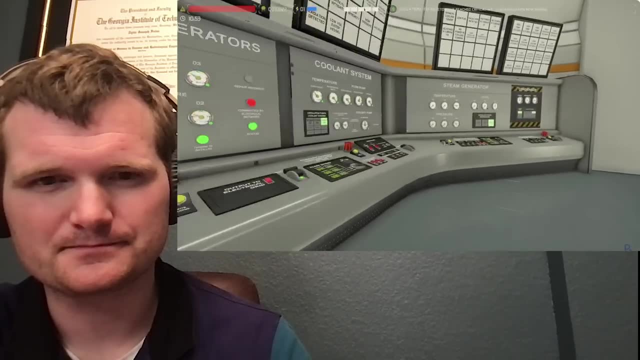 but typically you can let it go in auto. Now the interesting thing here is: if I run back over here, you can see my reactor is still only 180 degrees. You know we're barely boiling anything right now, But again, boiling is not the. if you're pressurized, you should never be at a point where you're. 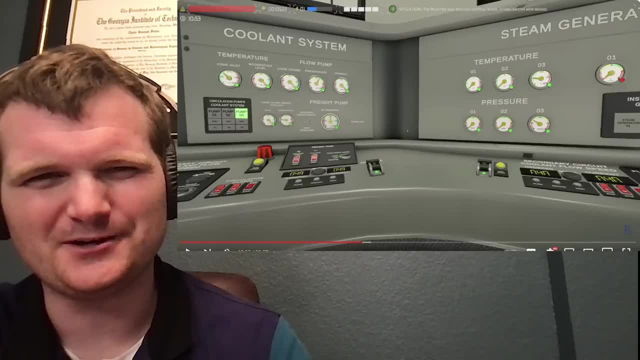 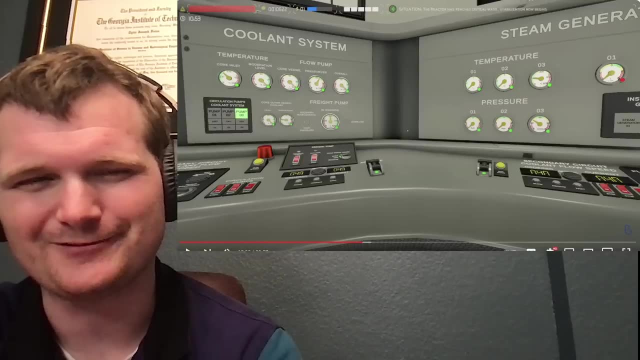 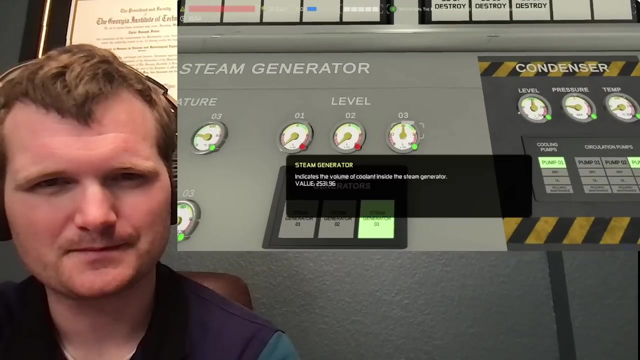 boiling And 180 degrees. even if he's talking, that's low. even if you're talking Celsius you should be. the average temperature should be around 600 Fahrenheit. So yeah, 183 Celsius is still super cold. This gives you an idea of just the tremendous amount of thermal power of these reactors. 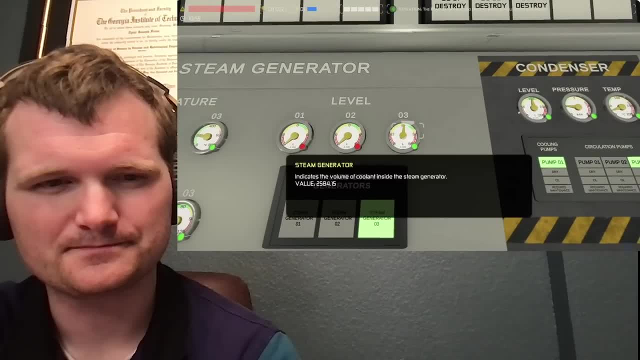 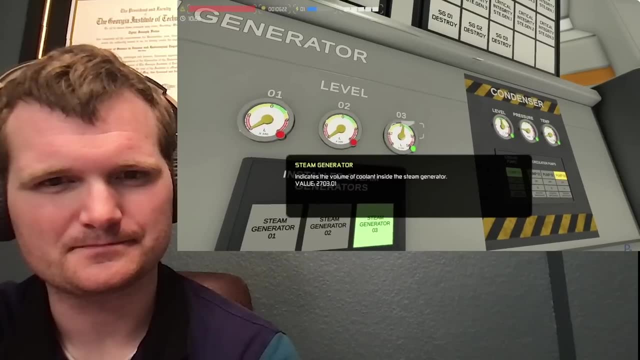 Now, if I swing over here, you can see that my steam generators start to sneak back up. That means we're providing too much water. So we're just gonna come here and crank this back down a little bit and you'll see how it starts to decrease, how fast by the whole way. 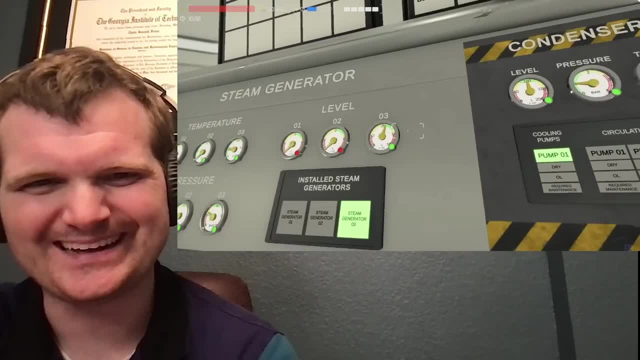 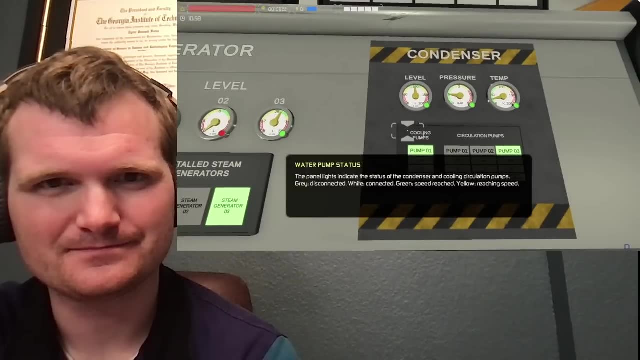 Hold right click here You have speed regulating valves to help you with that. Now, something important here is, when we produce steam, our condenser here, if you want to think about this, as the giant cooling towers- is going to try to take that steam and convert. 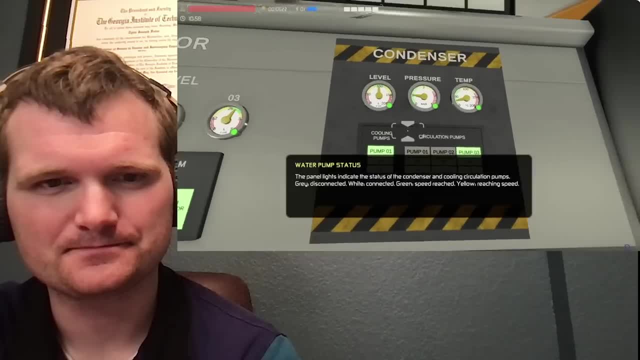 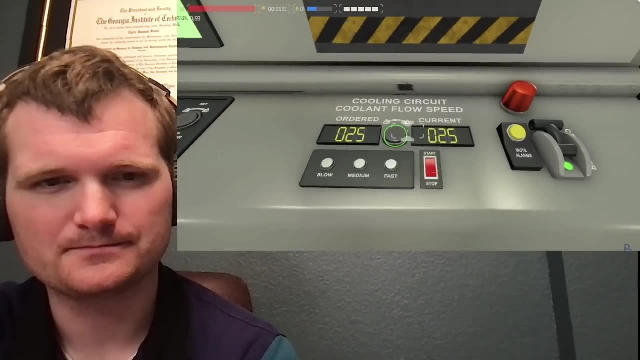 it back into water and basically eject the heat energy from it. When it does that, it's going to warm up. Now this is when things get interesting for us. That means that this speed, this little handle right here, is determining how much heat we 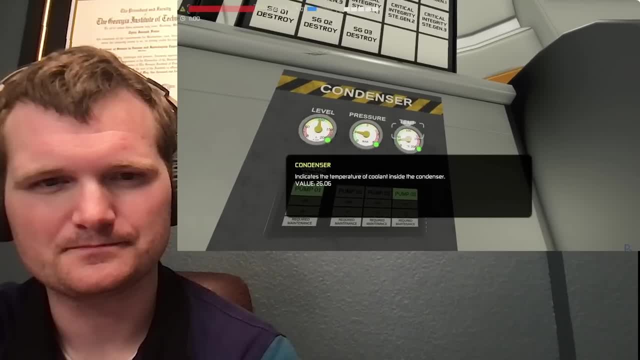 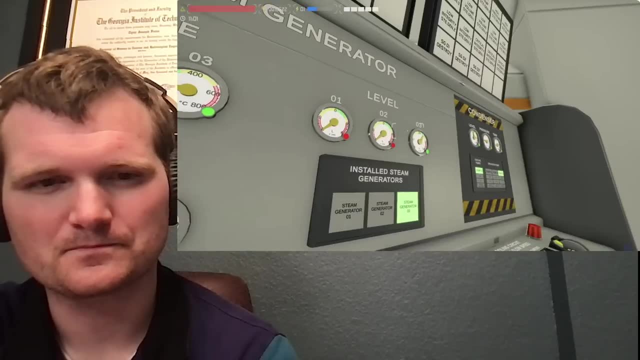 can essentially reject. So what's gonna happen is, if we cross this magic 100 threshold, that means we're going to start boiling off our cooling. That will cool things down. Yes, Also notice, by the way, how this Keep in mind- he's referring to the sec. 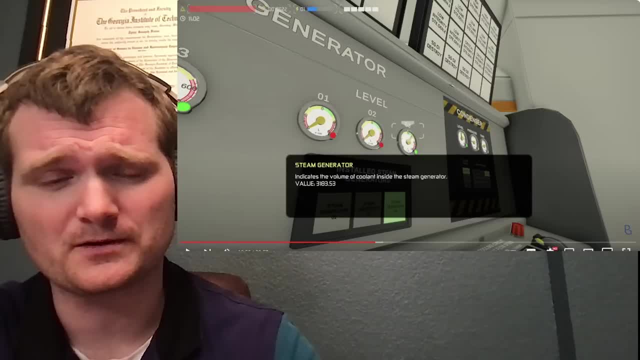 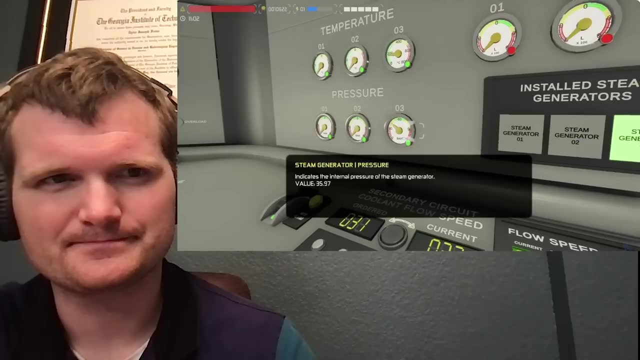 He's referring to the secondary loop. This is not referring to the actual reactor coolant system. It's running away on us already, So I'm just gonna grab this and crank it down a couple notches Again. we don't want it to get too high, but also notice how much pressure we're generating. 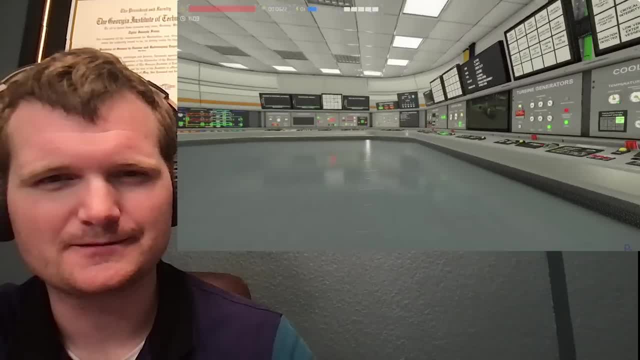 already. It's like just like that: A lot of controller babysitting. So let's go run back over to our system. here You can see a pressurizer is a little high, Not bad. Our temperature is 250.. It's warming up real quick. 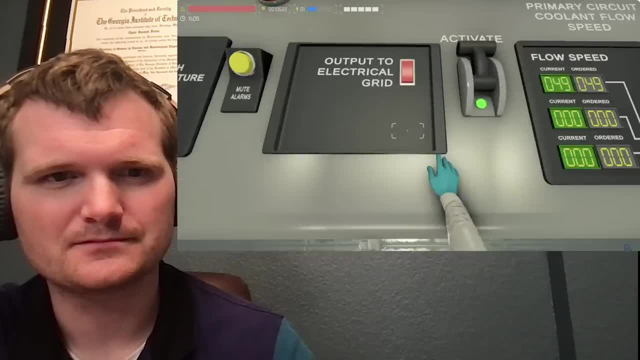 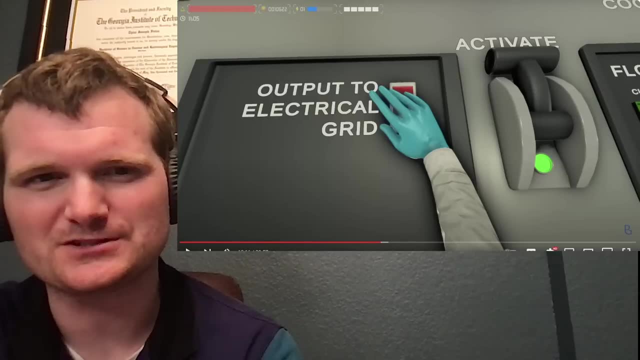 What are the units in pressure? We're producing electricity, So we're actually ready to go ahead and switch this. You're producing electricity, Have you not? have you not synced it yet? Or okay, or he's, or it means he's about to produce electricity. 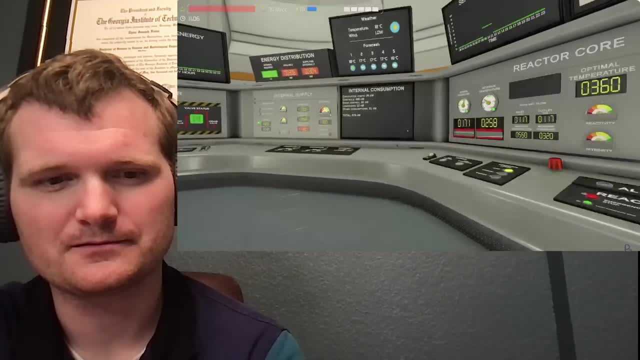 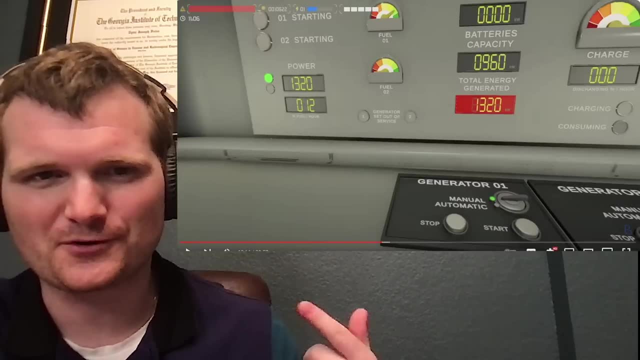 Off to the electrical grid Once that's on, of course, so we can go ahead and shut off our generator. So that's gonna be a delicate timing process because you're gonna need to use a synchroscope in order to see if the generator is in phase with the rest of the grid. 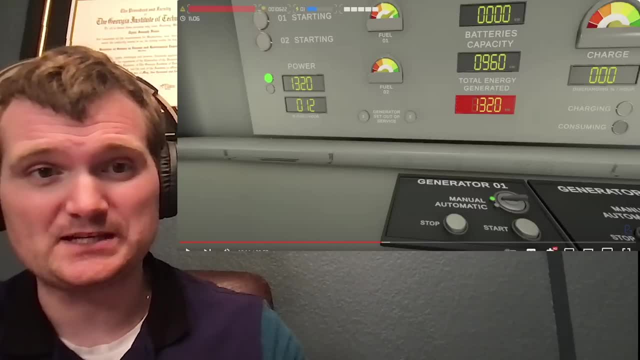 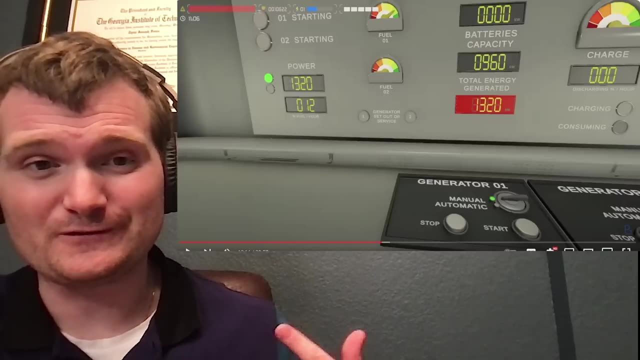 While nuclear power plants produce a lot of power, They're still tiny compared to the entire rest of the grid. that's, that's going on, And you- just you- really want to make sure you're in phase, otherwise you could break your generator. 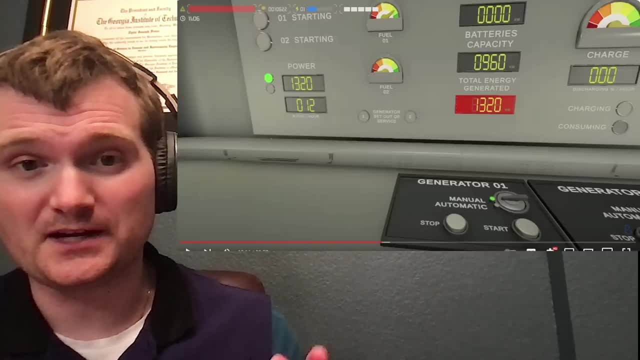 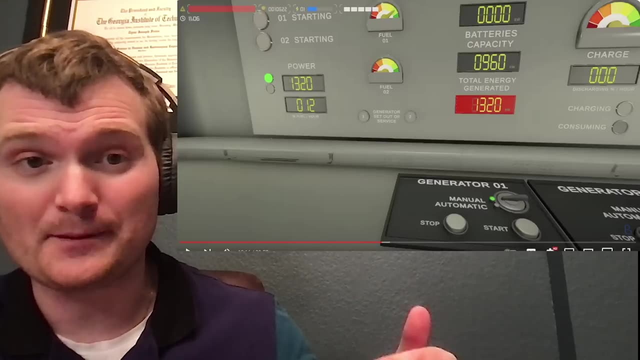 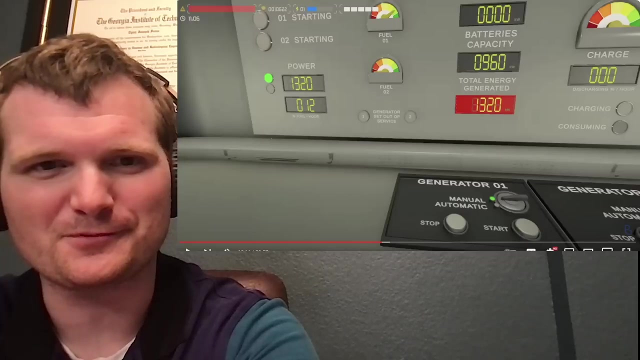 And when I say in phase, I'm referring to alternating current uh the uh. make sure your peaks are matched with the peaks of what's uh, of what's happening in the grid. So to compare it to a uh, another video game, like in a super Mario brothers. 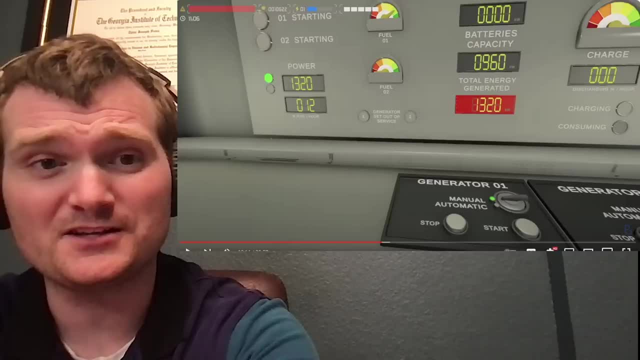 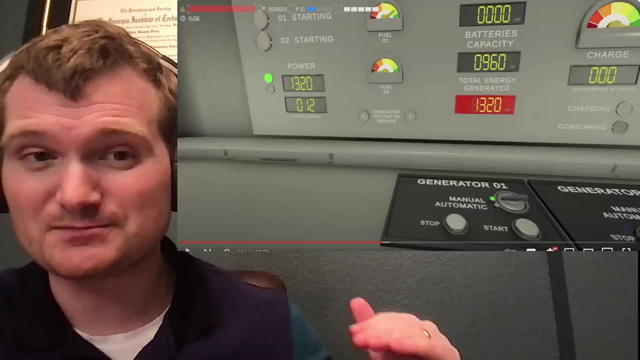 When you're jumping on the moving platforms. this- when to sync the generator- is the equivalent of when of are you jumping when the platform is close to you or when the platform is moving away from you? That is exactly what this sort of process is, because we now have the ability to produce. 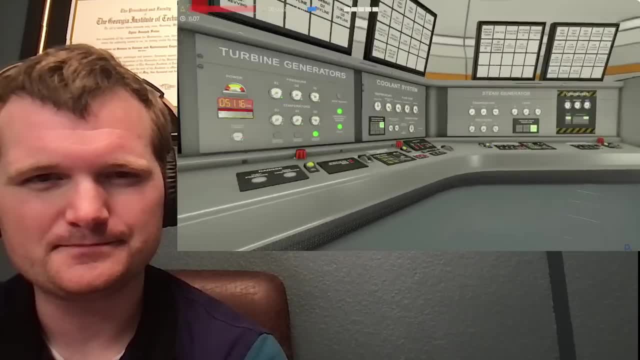 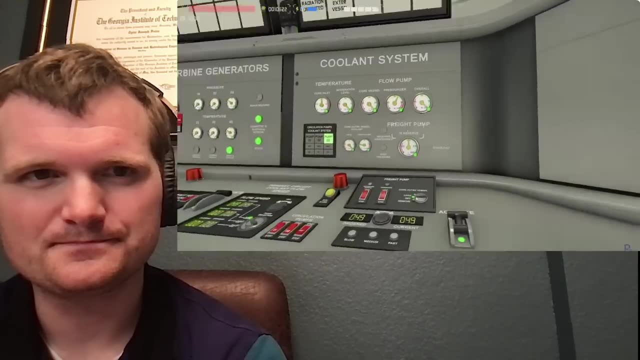 our own power. And now things start to get really, really interesting, really, really quickly. Now notice, I have not touched this yet. I'm just controlling the temperature and the cooling, If you want to think about, not through the primary cooling system, but by how much steam. 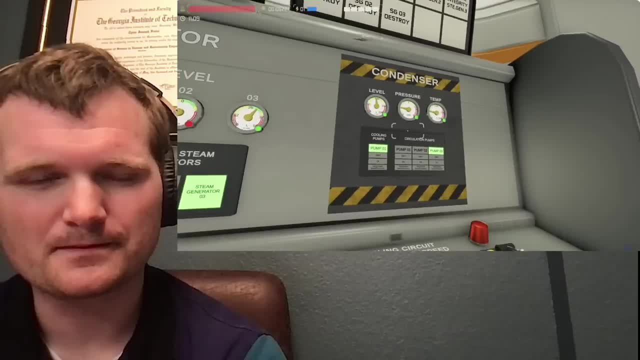 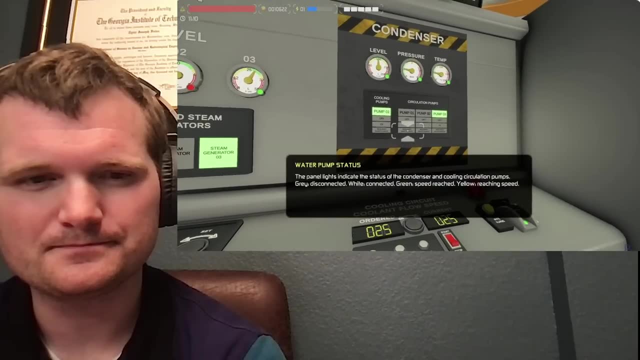 I'm using To uh turn into electricity and how best I can cool it off at the condenser. Remember, the condenser is basically the final place for all the heat we generate here And it only has a maximum limit of how much heat you can reject. 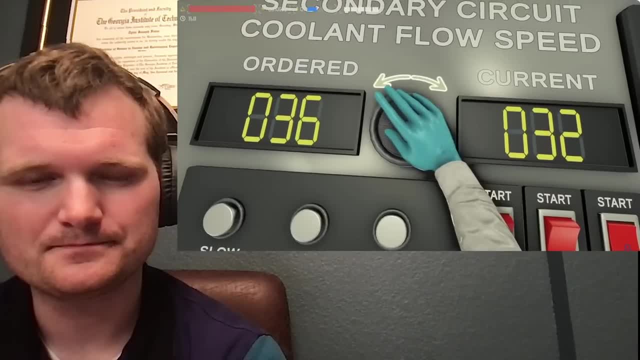 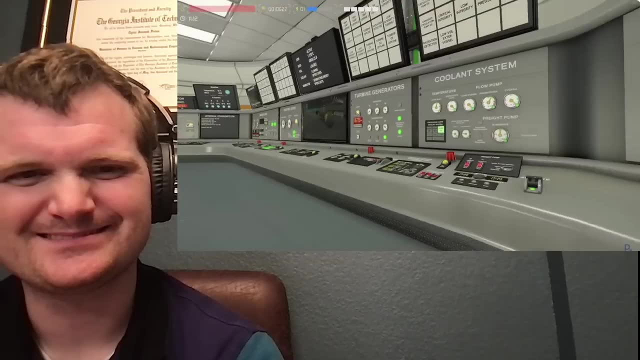 That's just one of those things. Oh, notice how this is starting to creep left again. So we're just going to go ahead and add a couple of percentages here, because remember reactors getting a lot warmer. actually, we'll kick it a little bit higher, go up to 40%. 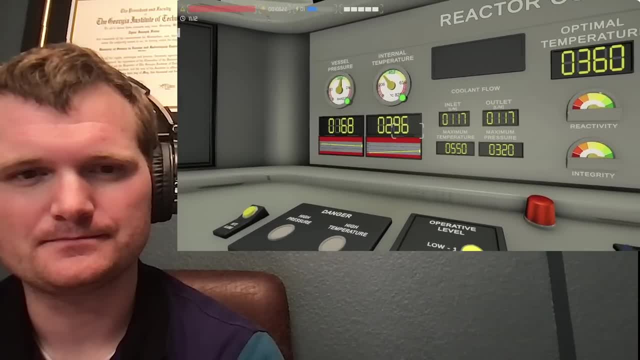 here Swing back over the coils itself. You can see we're about a three sixties ideal here, but um again, we're about 300 degrees. We could probably slow the uh temperature here, Climb here, Go down to 97.. 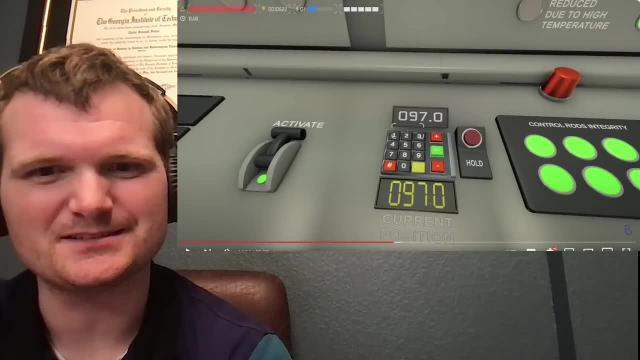 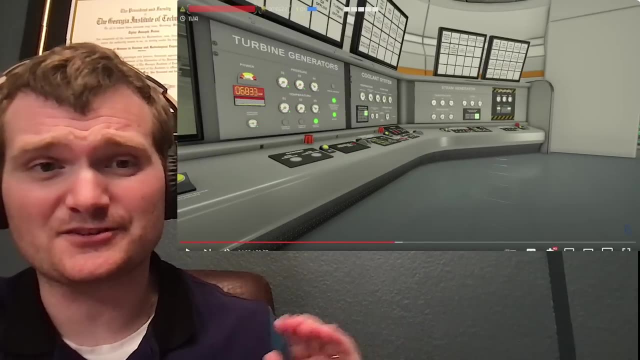 And again, that's just What is he doing. That's like a calculator. So position control rod, you don't need a lot of pool in order to control that temperature. Yeah, Usually you have a S. now this one is your. this one I'm used to seeing being manually. 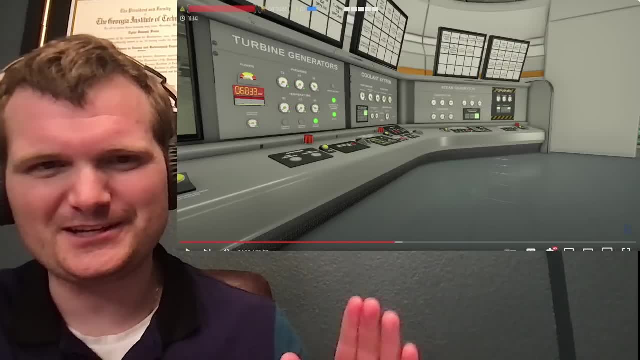 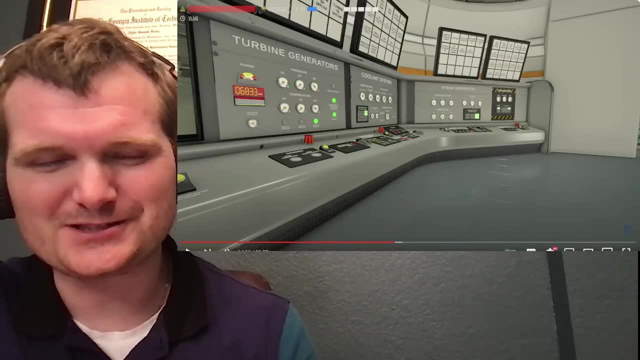 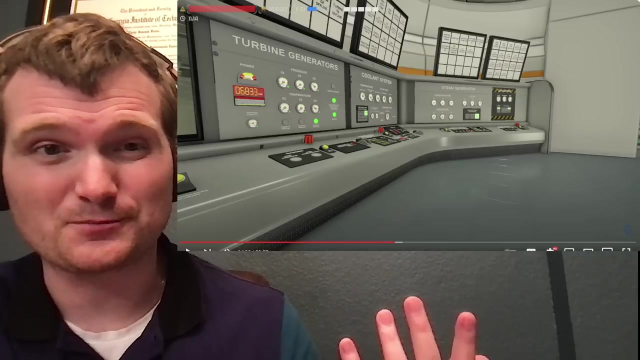 adjusted in order to, and there's so many control circuits and how well each of these things interact with each other that you don't have to do nearly as much babysitting. but I will say control rods are typically operated Manually, especially when you're starting up or raising reactor power, in this case. 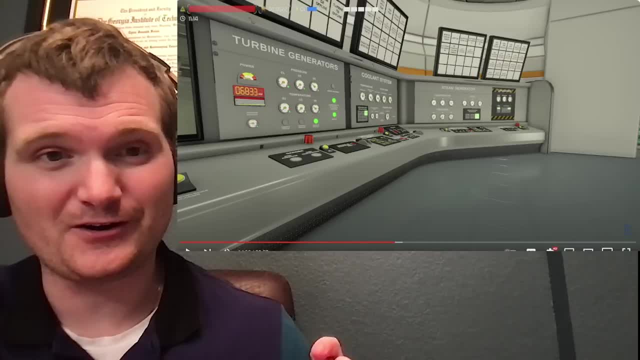 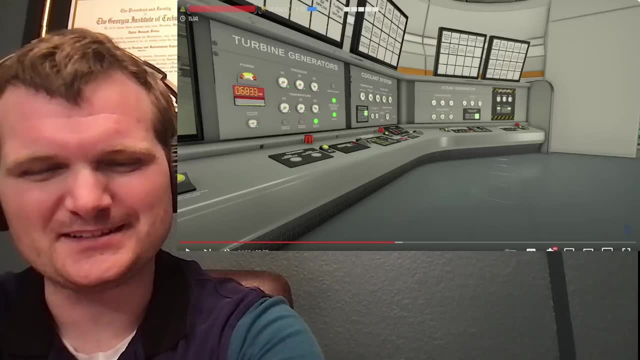 And keep in mind, each of these operations that affect reactivity are going to be peer checked by another reactor operator and oversight is going to be given by a supervisor, So everyone is going to know what you're doing and how it affects these other reactor systems. 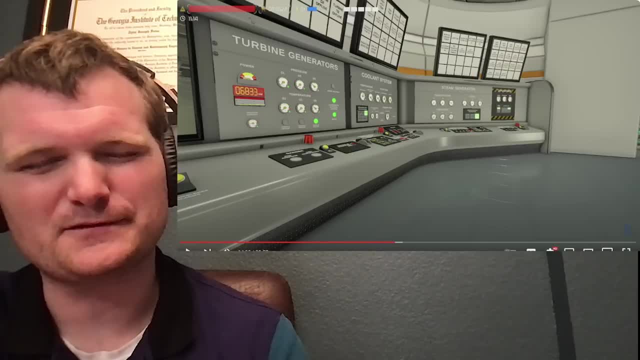 as you're moving this thing. It's really cool. I can kind of understand, for the purpose of the game, though, why they didn't make it in the first place. Yeah, I don't know. just to teach you sort of how things affect each other. 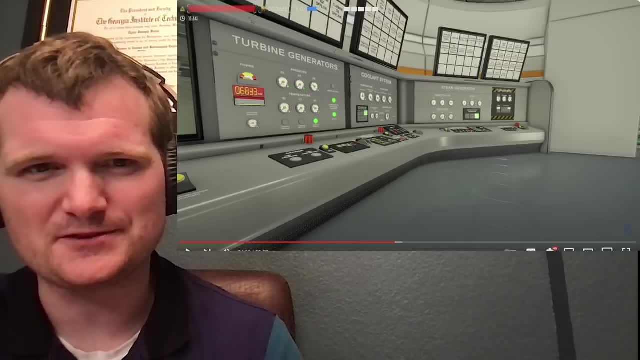 So while I've noticed that a lot of these numbers are off and it can let you do things, some things that don't have you makes, that don't really make a lot of sense. It is teaching you what in nuclear operations we call integrated plant operations, which 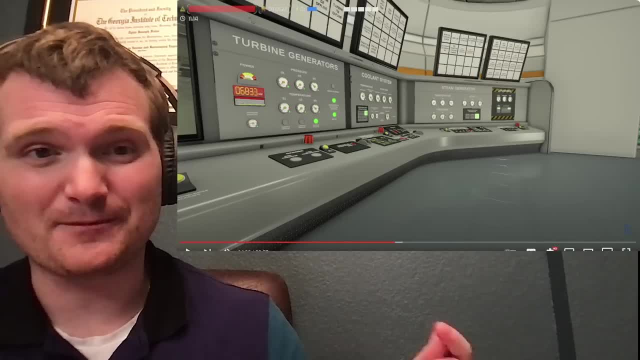 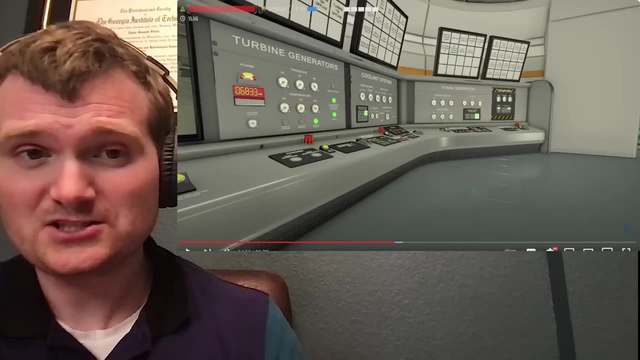 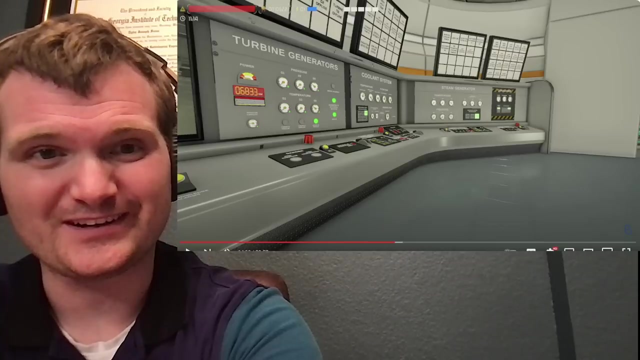 is basically how something affects something else, how what you're doing to the condenser affects, re, affects the reactor, and it's. the orders of magnitude are off, But the Yeah, The overall concepts are there and it's really cool to see that in a video game. 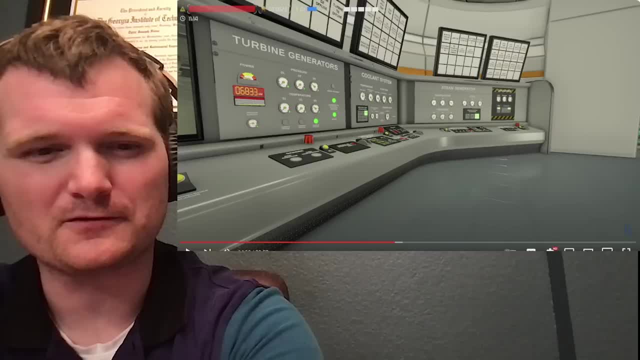 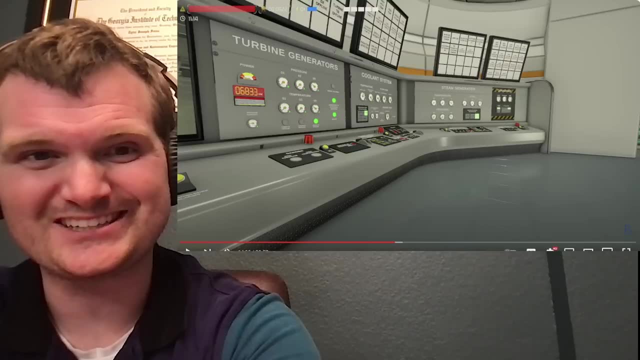 I think I'm going to go ahead and call it apart. I'm going to go ahead and call it apart for now. There will be a second part to this. Thanks so much for the recommendation, though. This is a really cool looking, shiny video game.